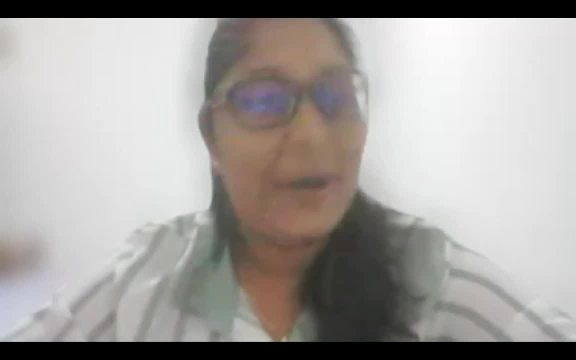 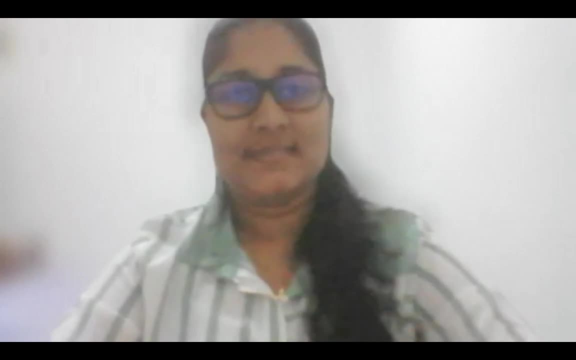 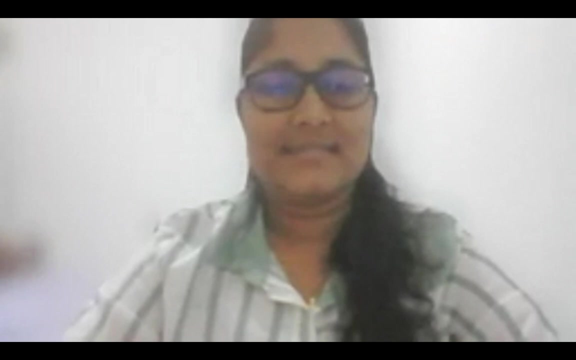 Welcome. I'd like to hand the session over to you. Thank you, Good afternoon all. So welcome to the workshop series of image processing right? So let's jump straight to the installation of OpenCV. So OpenCV is the library used for image processing, right along with. 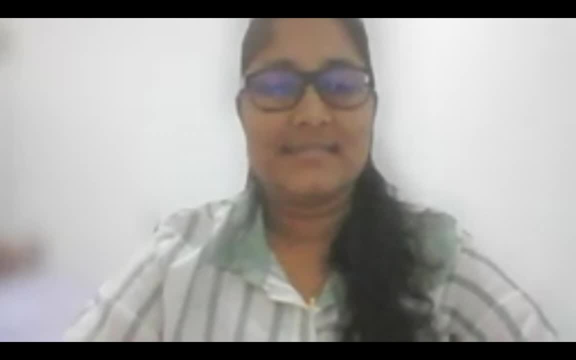 Python, So you have to. so prerequisite for this workshop is to have a basic knowledge of Python. right, You should have basic knowledge of Python and you should be able to. you should be installed. you should install OpenCV in your computer. So let's jump into installation. 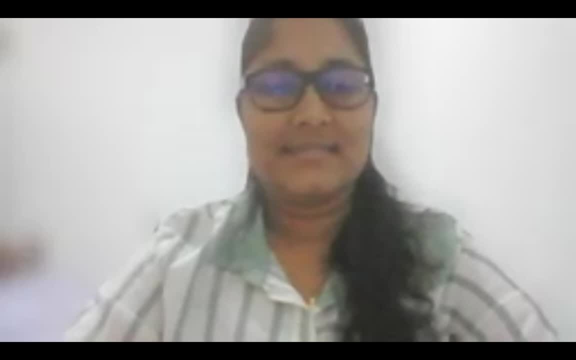 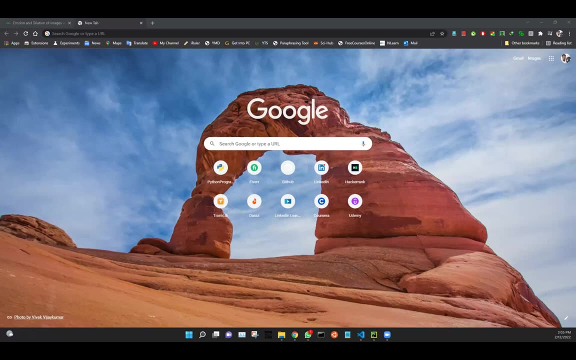 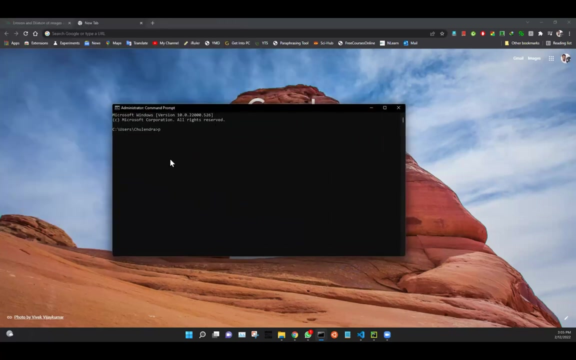 So to install OpenCV, you should issue the command tp install opencv-python. right, So this will install OpenCV in your system, right, So you can install this command. Also, you need to install NumPy. NumPy also has to be installed. 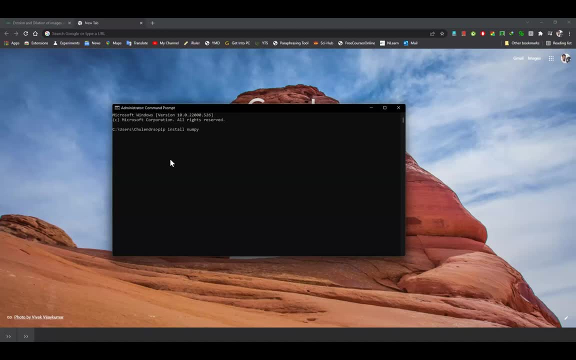 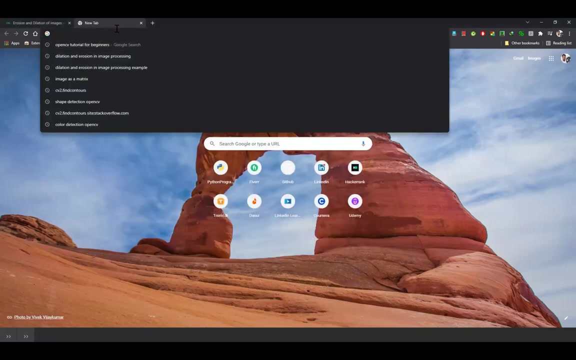 because NumPy is used along with OpenCV. So when we sometimes we need NumPy array for our code, So for that we need to install NumPy asset, So install these two. So if you are in Anaconda there is a nice, nice channel for OpenCV. 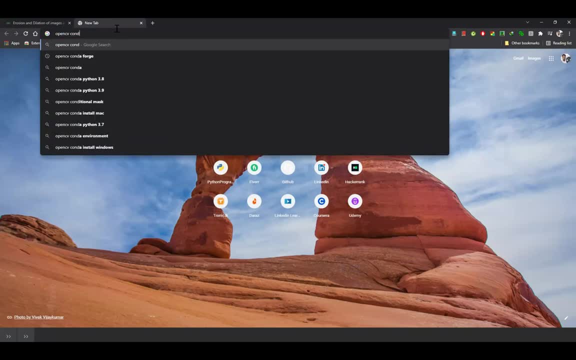 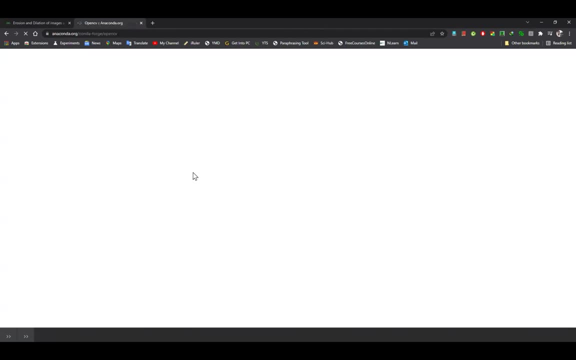 OpenCV-Conda-Forge. You can install OpenCV in Conda using this link, Either using one of these links, So I install using this link. This way also, you can install Anaconda. sorry, OpenCV. Yeah, so that's the installation part. 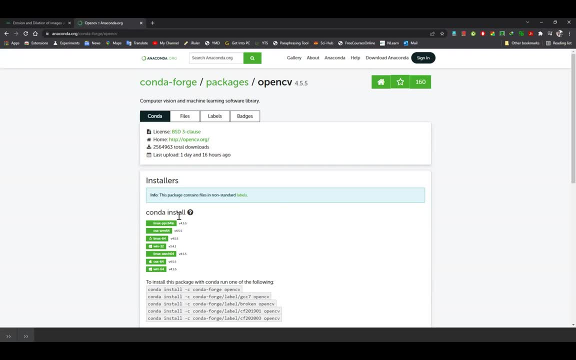 This is a heavy package. It comes with optional packages and dependencies Required for our workshop series. So it takes some time sometimes. So I recommend you. so if you are installing OpenCV now, I recommend you to install using: install opencv-python, right. So 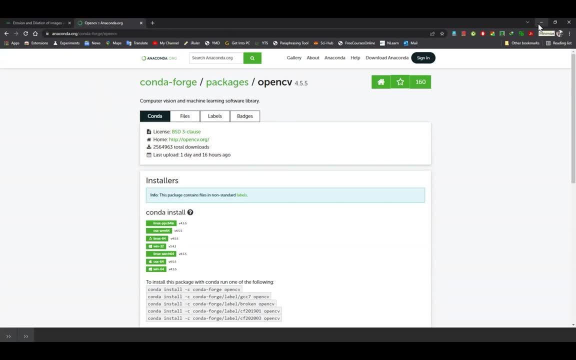 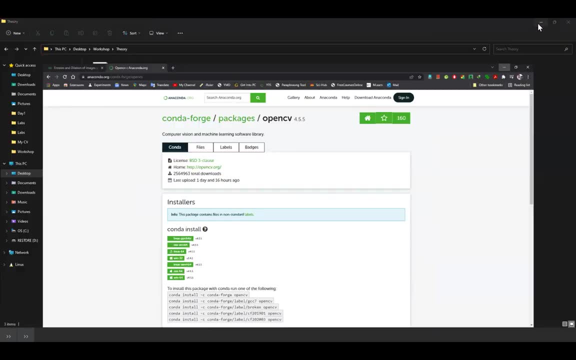 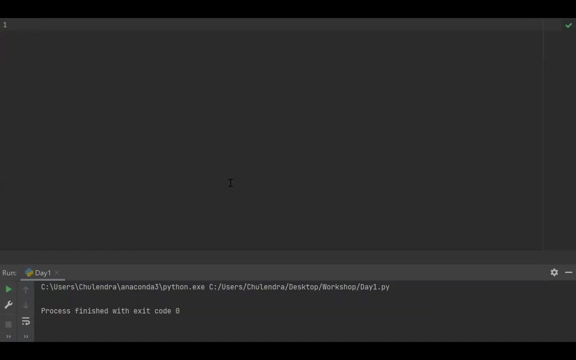 yeah, so this session will be. so our coding session will be done in using PyCharm IDE, So you can use your own IDE for this. So I prefer to use PyCharm. So now I am in PyCharm, right. 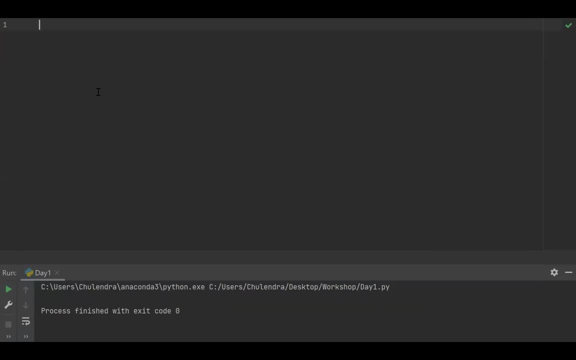 So if you successfully install OpenCV, you should be able to import, import CV2.. CV2 is the library for library in library. the of the OpenCV, This one is, and see whether you can import it successfully. 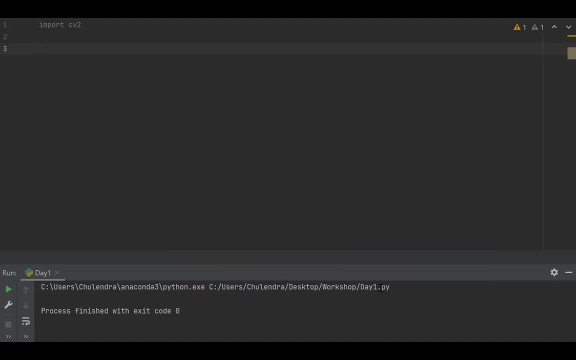 So my guess this in turn, in turn, successfully. So make sure this import CV2 works. Yeah, so. So if you have any questions, post them in the chat or unmute and ask the question. So for this practical, so this workshop, you need some materials. these are the images. 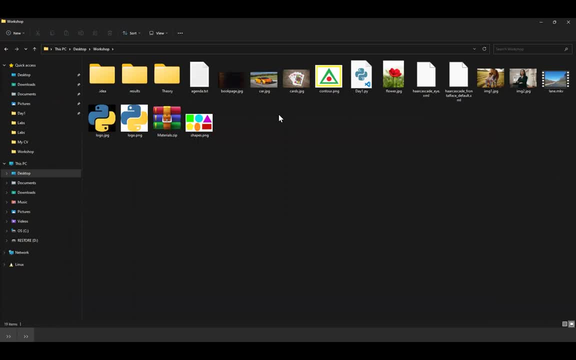 and videos that I am going to use during the workshop. So I made my zip file. I'll share this in the chat. Just download it Now. I am posting it into the chat. So let's talk about. So let's talk about. 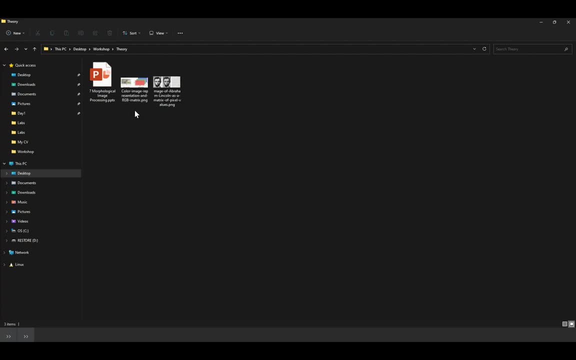 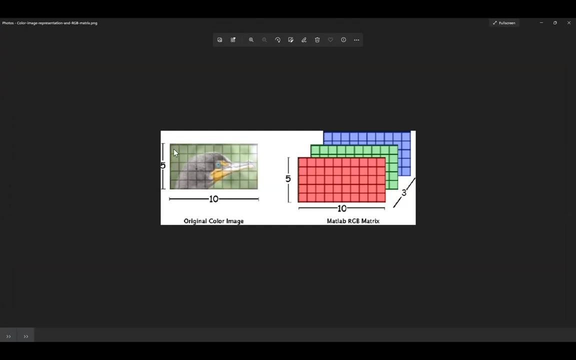 So let's talk about what's the image actually, right? So image is, so let me open this one. So this is the image, right? How this image is, what is the structure of the image? What is the? what is the structure of the image? how image is made, right? 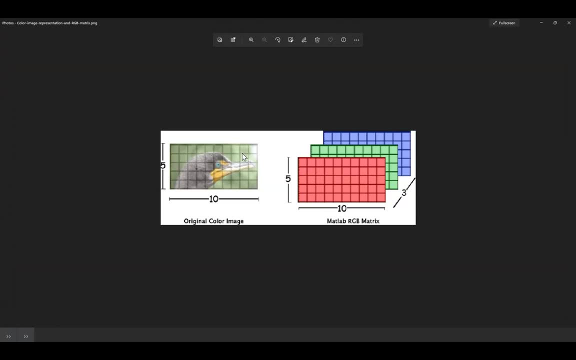 So image is made with, made with pixels, Something called as pixels. So consider these boxes as pixels, right, Boxes as pixels, And so so image. this image is nothing but matrix, right, It's a matrix. So so this, this is a color image. 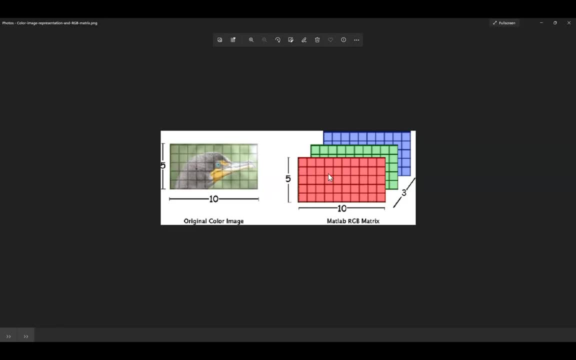 So color image has three channels right. These are the channels- red channel, green channel, blue channel, right So So the picture has a resolution associated with it. What is mean by? what is the meaning of resolution right? 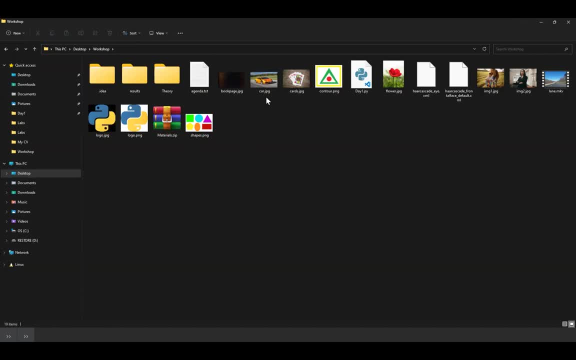 Resolution is nothing, but let me show you one picture. So this picture if you, if you right click and publish this picture, then it will pop up the detail of the of the picture right. Go to the picture. Go to the details. 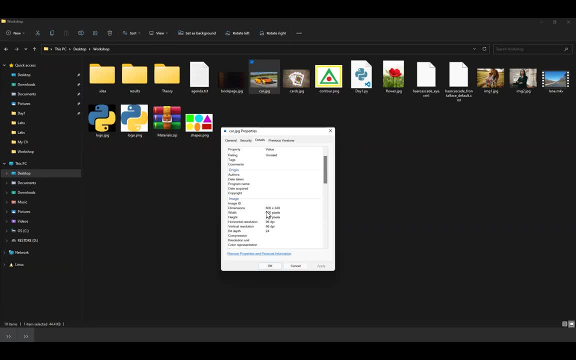 Then then here you have the resolution: width and height: width and height in terms of pixels, right? So this, this image, is a hundred pixel. we, we are wide in wide and 349 in height, right, So this is known as resolution. 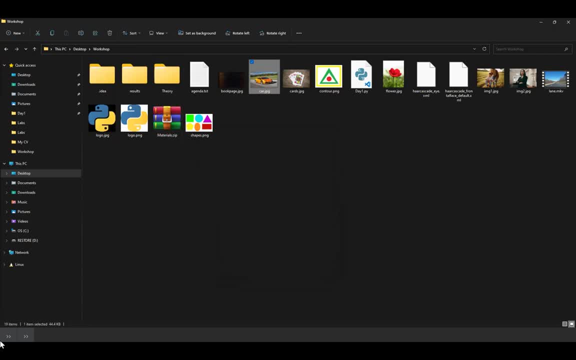 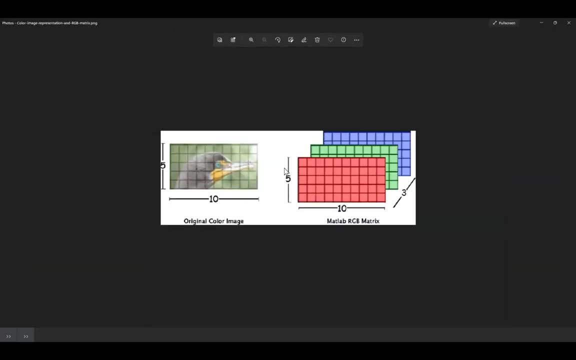 So, so, So this image, so this is the height, the five is height, 10 is width right. So resolution is: resolution is given in first, first given, given given as height comma, sorry, width comma, height. 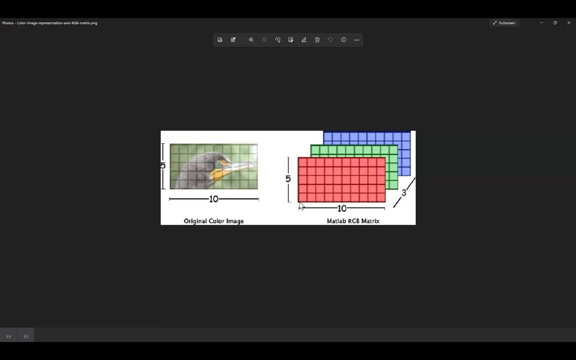 So in this, in this case, 10 is width, 10 is height, 10 is width, Because 10 comma 5 is the resolution, right, 10 comma 5 is the resolution, But the when it comes to matrix. so it it is 5 by 10 matrix right. 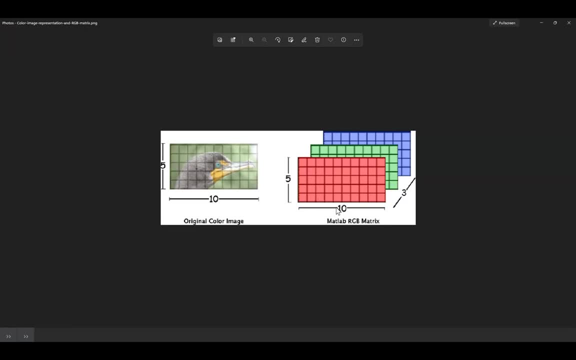 10, 10 comma 5, the the, the image with the10 comma 5 resolution produced: 5, 5 by 10, 5 by 10 by 3, actually 5 by 10 by 3 matrix right. 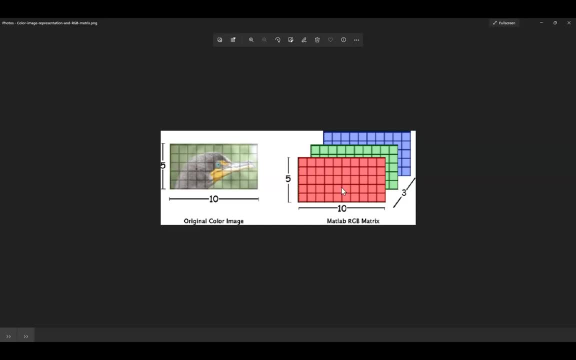 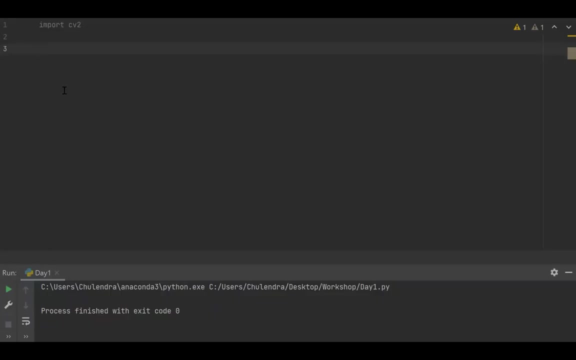 So, so, So, Yeah, Yeah, so let's, let's, let's check this, check whether this is true, right? so in my ide. so first, so let's, let's open the image using opencv. for that we have to write a variable, image equal. so this is an umpire. actually, image is an umpire. 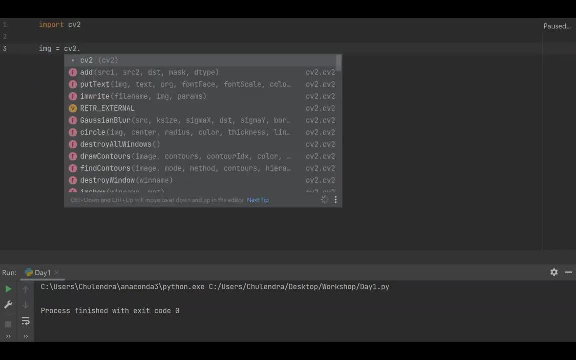 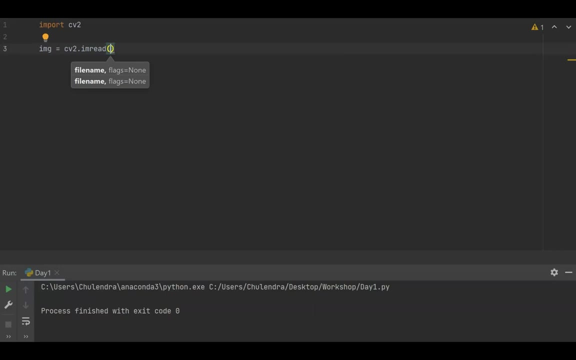 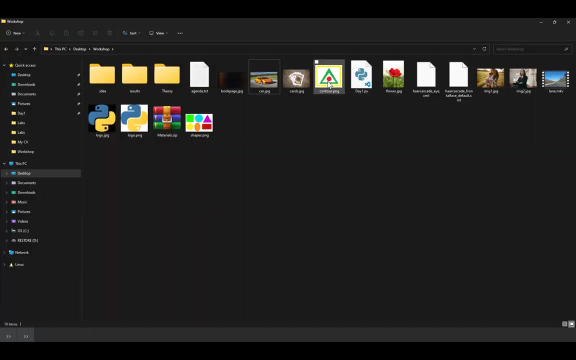 so cv2 dot in read. in read is the function used to read the read the image from a local drive, right? so here you have to enter the file path. so so i am. so my script is in this folder, this folder day one dot pi folder. so my image, my uh. 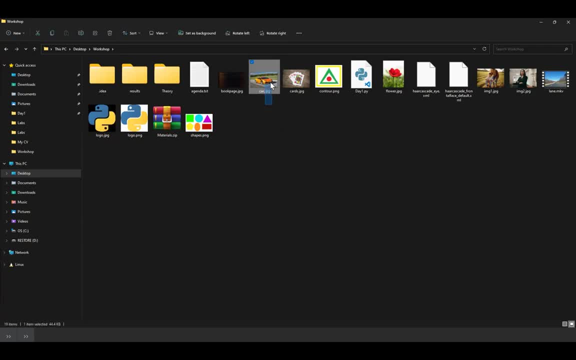 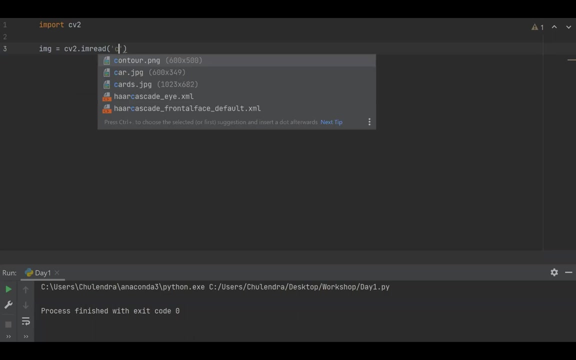 required image. the image that i'm going to open is carded jpg, so it should. it is in the same folder in as as my code, this right, so carded jpg, so carded, so pi charm. actually, it is very intelligent, so it suggests me the file name. 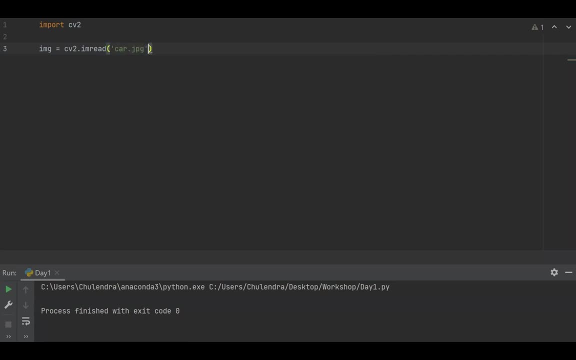 so carded jpg, jpg, then, so, then, so the image is successfully import, open. then let's view the shape of this array. shape means shape is nothing but the dimension of the array. so let's print this out so that we can see what's in it. let's run it so. 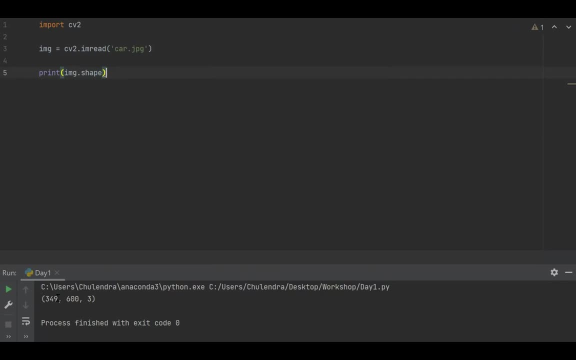 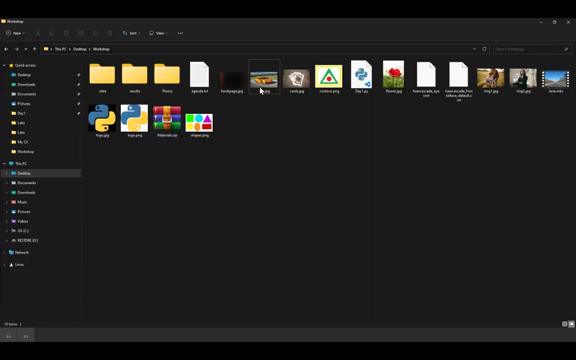 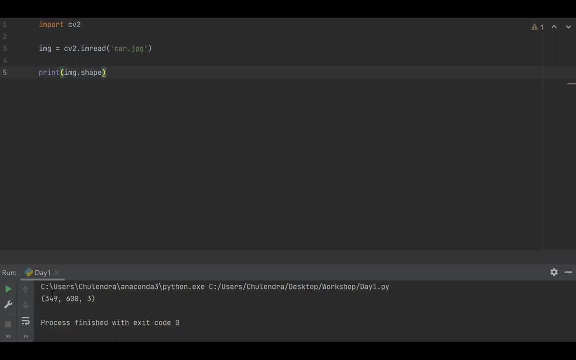 this is 349, 349, 600 by 3. see 349 by 600 by 3 matrix. so let's see whether it is true. so properties here: details: image: with this 600 pixel image height is 349, so so you get 349, 600 right. so first, first, 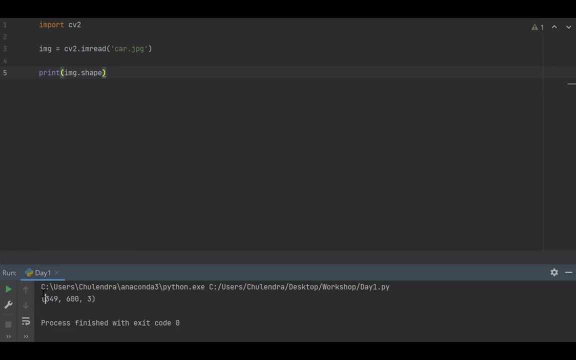 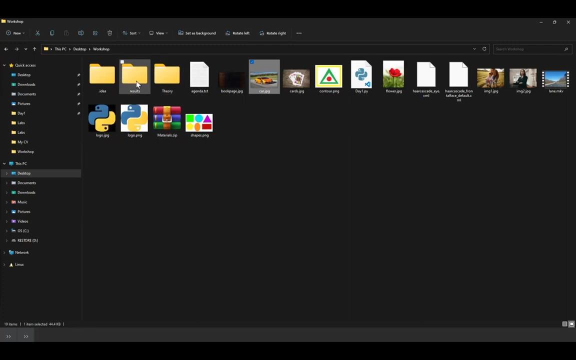 first in in in matrix notation: uh first it gives uh the first dimension gives number, uh the, the height. the second dimension, second term in the dimension, gives uh width and the last term gives the dimension. so height, comma, width, comma, channels, right, so there are three channels right. so that's what i uh depicted here. 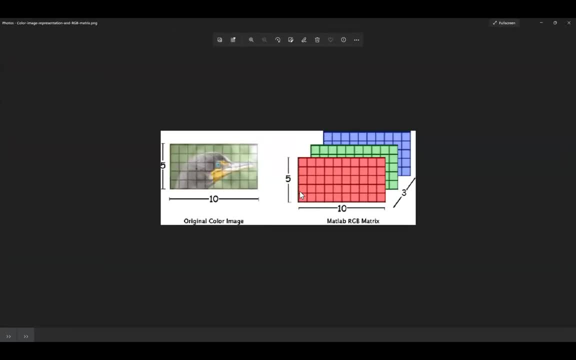 right, repeated here. uh, so so, but there is a problem here. what is that? so? so this, this is so. i downloaded this picture from the from google, so it says: matlab rgb matrix right in matlab. this is okay, red channel, green channel, blue channel, right, but in image processor, sorry, in in open cv first. 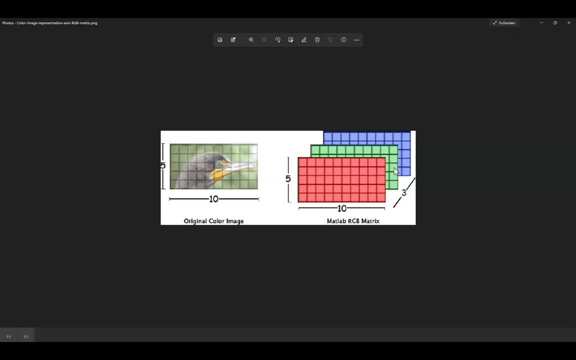 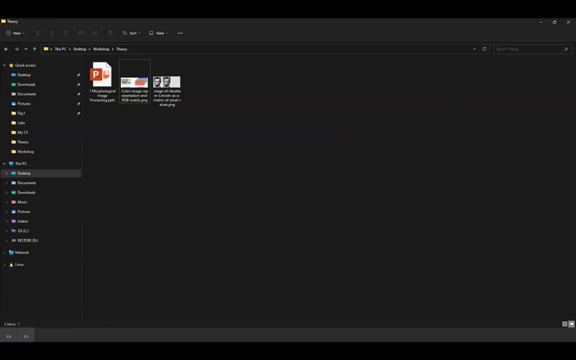 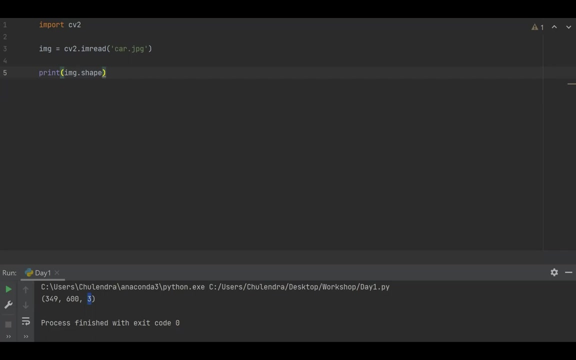 blue, then green, then red. vgr, not rgb. it is pgr. in open cv, the image channels are pgr, the. the order is bgr, not rgb. keep hitting your mind. so so let me, uh, let's visualize, let's see this image. you can see this image using cv2- cv2.in show. 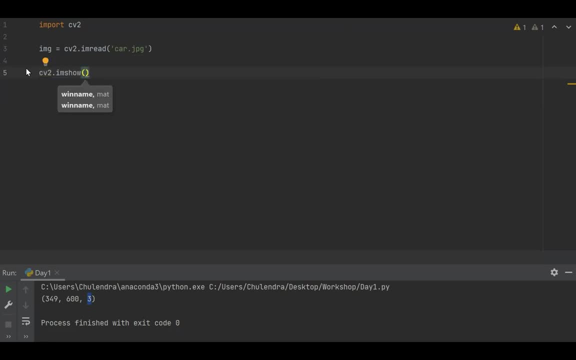 in show. then you have to give the window name. window name. i'll give a image comma, the. the array. array is image, the image is image img. so let's run this. before before run this, i have write one more, two more lines. cv2 dot: weight key zero: weight key zero is nothing but. 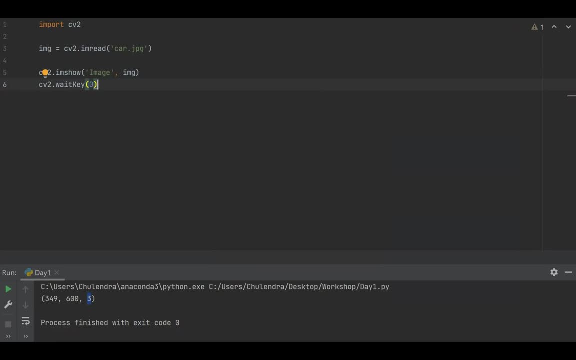 it. it waits until until you suppress a key keyboard key, right? uh, it wait until i use a press a key, right. so this zero means? uh, i'll i'll tell you what this zero means. uh, cv2, next cv2, destroy all windows, right? so this means so we, so we are reading the image into an umpire record. 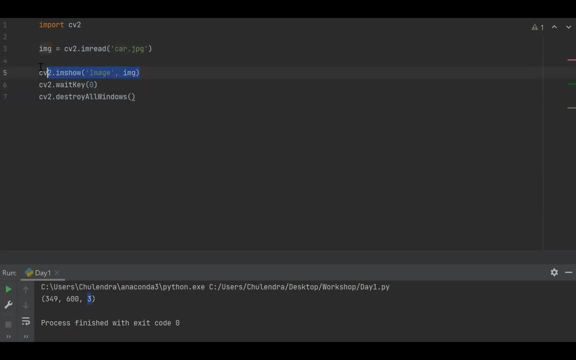 and g, then this image is visualized, shown right, then it wait until you suppress the key, and once you suppress the key, the image should, should, uh, disappear. the window should be destroyed. that's what that's the meaning of this: destroy all windows. it destroy all the windows. 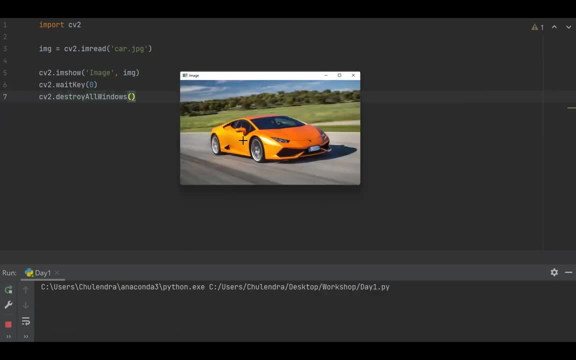 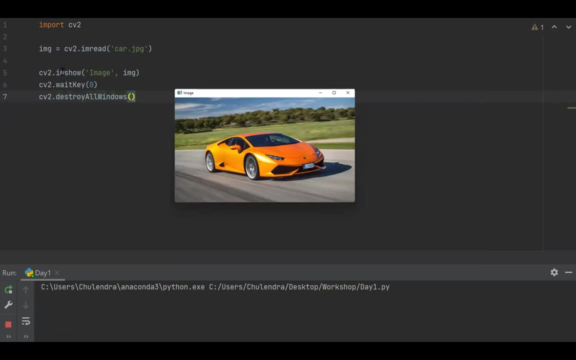 right, so let's run this. so this is the. this is the image in show. in show, this is the result of intro function for cv2.in show. the window name is image, so this is the name image and this is the uh imd. so this is the content of this imd. 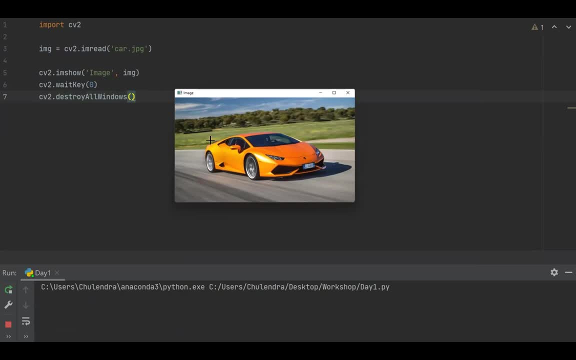 right, so, so it wait until you suppress the key. right, so you have to select this window and hit any, any, any key on your keyboard. right, then it will destroy that window. so that's the that's the basic idea behind this code, right? so let's, uh, let's view, let's. 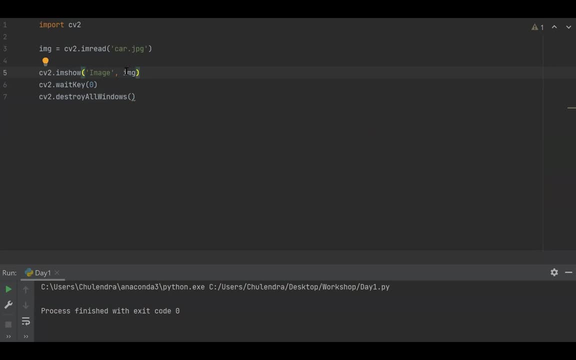 view the anatomy of this image. right, let's, let's print a single pixel of this image image. so i consider the zero pixel, zero, zero pixel. that means the coordinate, the pixel at coordinate zero, zero. so let's spin this out, so i'll come in this out. uh, let's clean this. so this is the. 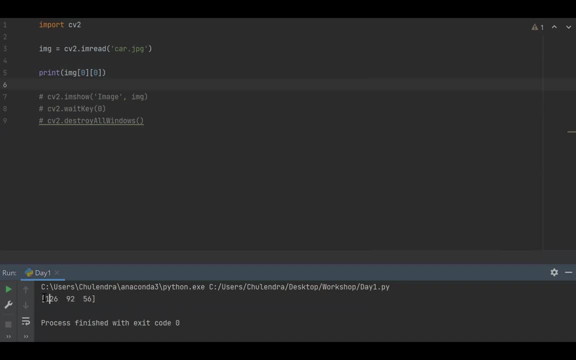 rgb value, sorry, bgr value. all right, right so, blue channel, green channel, red channel, blue green, red, bgr, right. so so this is the first pixel, first, first pixel of this image, pixel value of this image. so so it's a list of it is a row array of numpy array of three dimension, three dimension right. 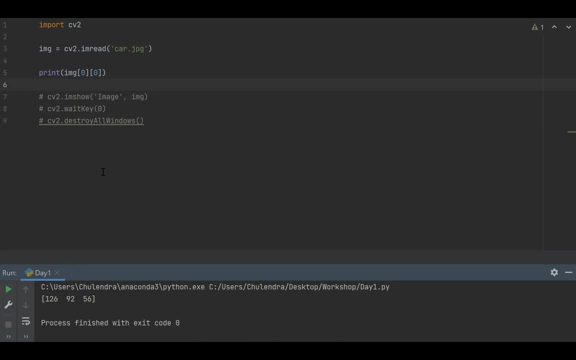 three, sorry, three, three items. so also i'll do some fancy thing here. image: i'll consider first, i'll sacrifice this image zero by zero. image zero by zero, uh, region of the image, right, i will make it as black black mean zero, zero, comma, zero, comma, zero, right. 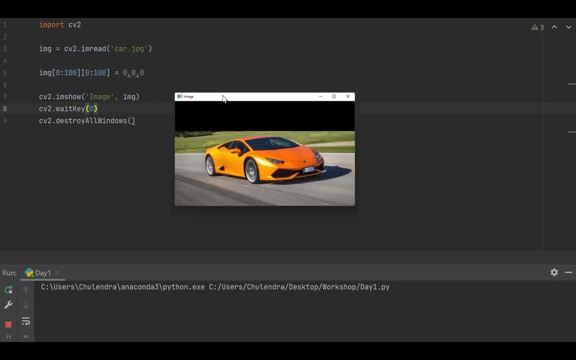 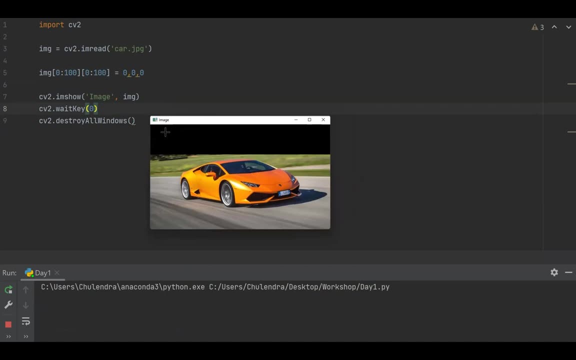 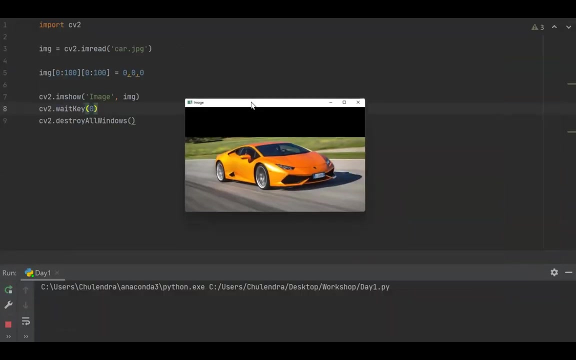 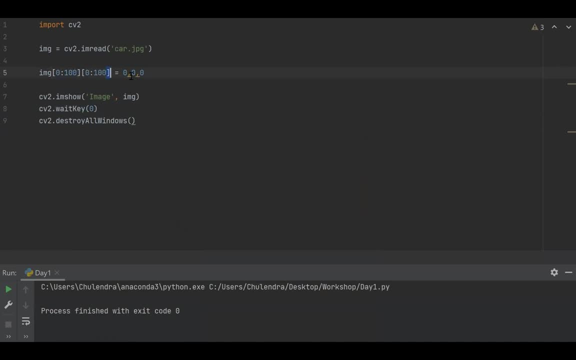 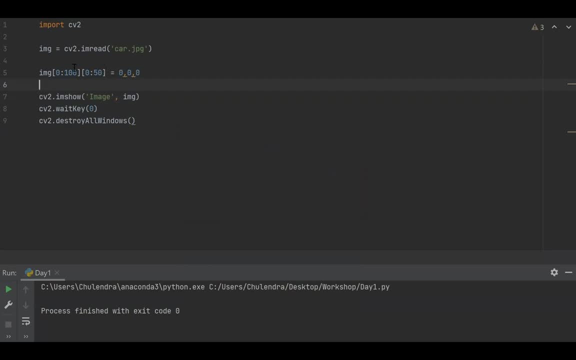 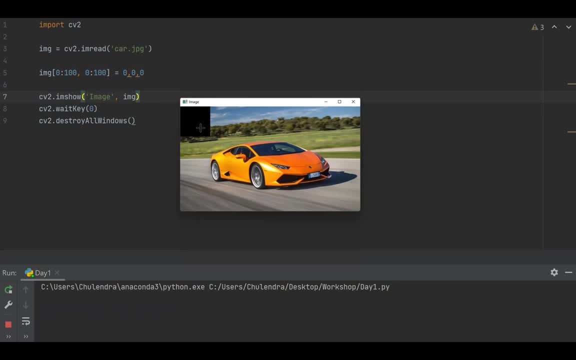 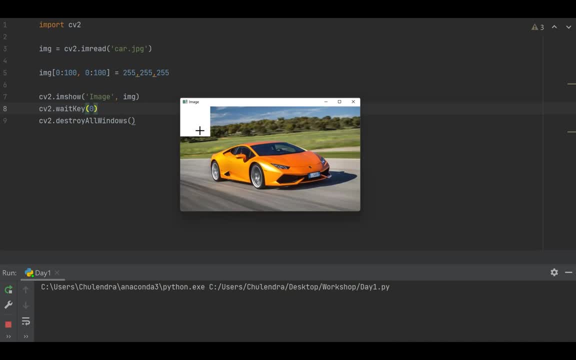 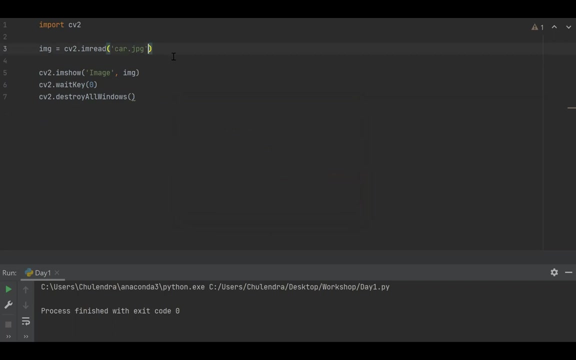 values of value of a particular pixel. so so let's exit this, remove this. you can directly be your image in black and white also. we can do this by issuing zero comma zero. this will give you a black and white image. this is known as grayscale image. right grayscale mean back and white, so 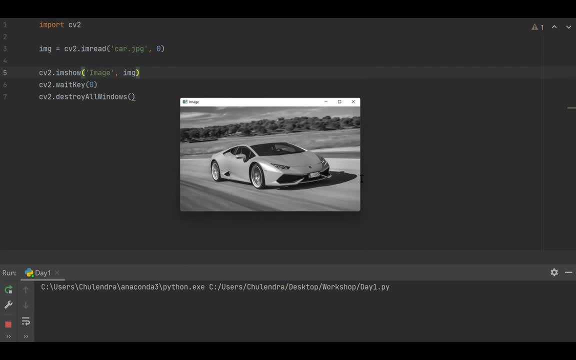 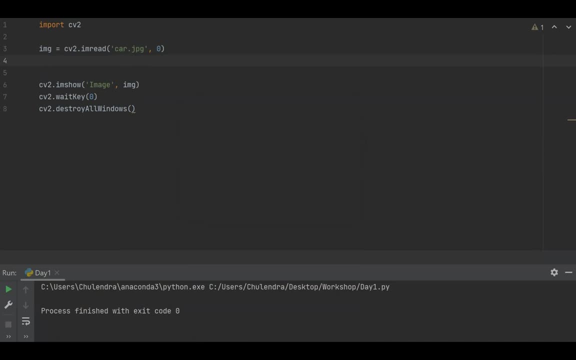 so if you inspect the shape of this array, so let me print img dot shape. so it is this array of uh array with two dimensions, right, not three. earlier it was three because it is a color image, because it was a color image, but now it's a grayscale image. grayscale image has a single. 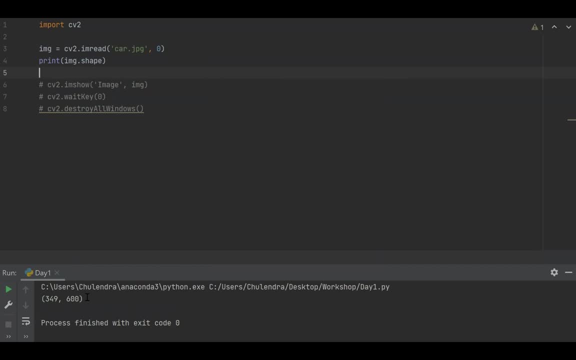 channel, so we don't need to worry about a third dimension. so that's why, uh, it gives 349 by 60 standard, right? so? so keep it also in your mind. so if you have any question, feel free to ask. next. next, let's see how to uh read your webcam. right to do that. 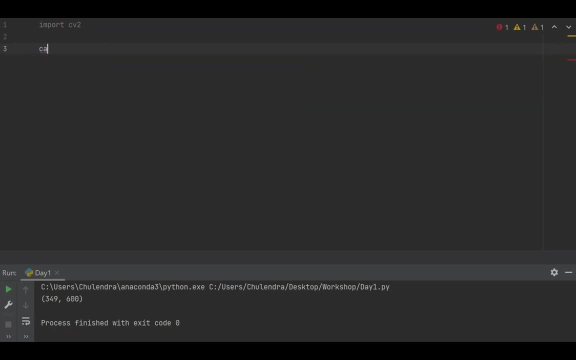 you have to create the object by name test cap using video capture pass cv2 dot video capture class. here you have to pass the, so to access your webcam, so your your. i think i believe everyone has a webcam with you because, uh, most of you, i think. 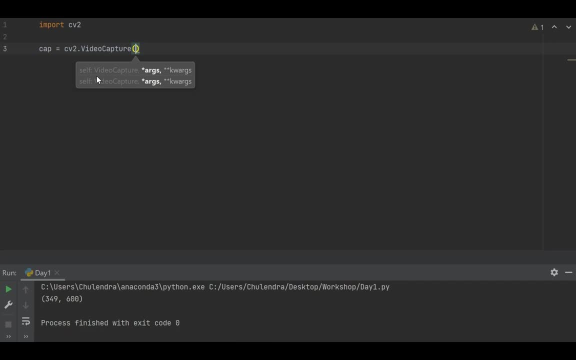 almost all of you are using a laptop, so the laptop should have a webcam. uh, if you don't have a pen, you have to connect the external webcam. uh, don't worry if you do. if you don't have a webcam, you have to connect the external webcam. 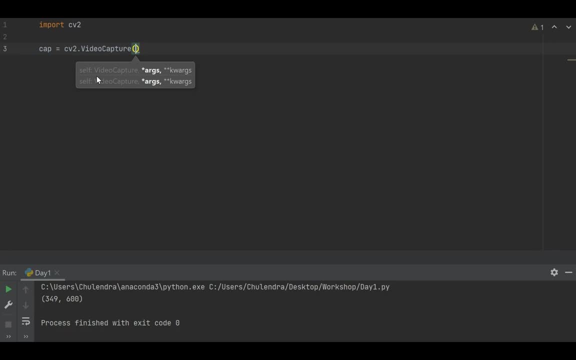 don't worry if you do, if you don't have a webcam, faltado long with this tutor, with this uh, with this uh workshop, using images, uh or video. so so i put here one. you should enter zero here, right, i should. so this is so. i have given you the. 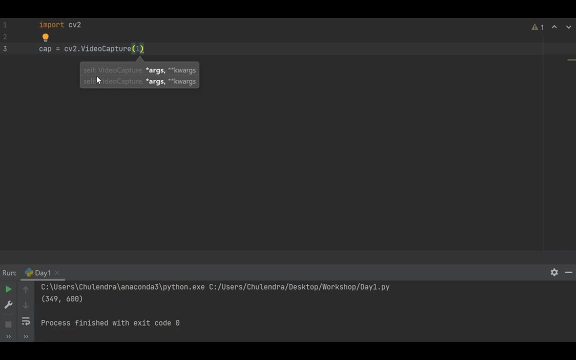 two things right now. i might write 10 in there, but i first leave them here and then i'll move them now if i want. so let me make my loses, or some of them. i'll include them in my Division s Java, Sandra. this is so: if you enter zero, it will read your first webcam. if you enter one, it will read your. 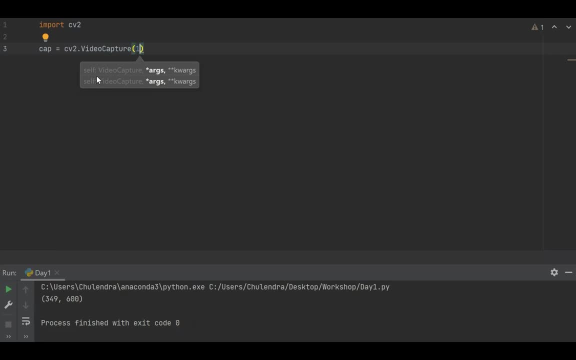 second webcam. i have two webcams: my laptop webcam and my and i, and also i have a separate webcam, uh, connected to my pc, uh. so so i'm using this webcam for this tutorial, so i do, i, i, i give one here, you, i think you should. you should give zero here, then, while. 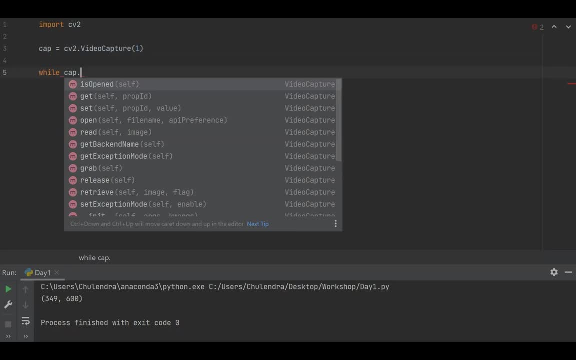 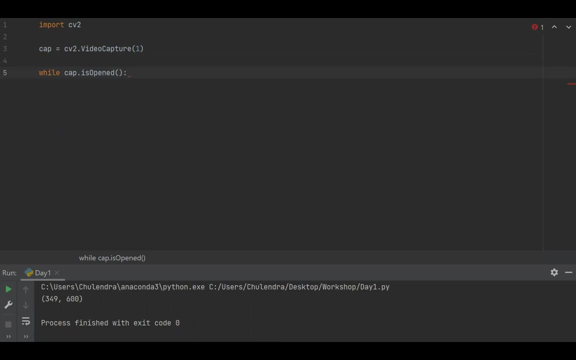 as long as this, this capture object is open, that means your it can is open. so that's that's what this means. cap dot, cap dot is open, so it will return, whether it is through or whether it is open or not. so it generates two or four words: boolean. well then. 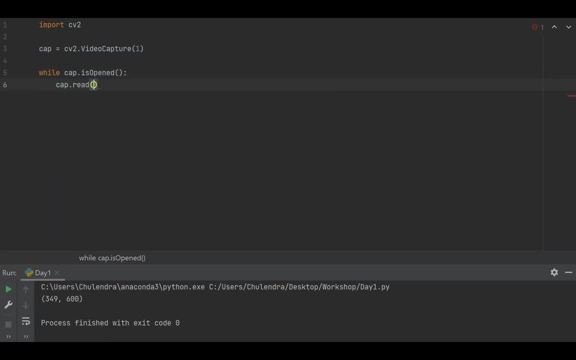 cam dot create. sorry, eight comma return value. uh, this, i'll tell you what this is, what these are: eight comma frame. cap dot tweet. so this is where you reading your webcam with webcam. cap dot tree. so this is your webcam object. so here, here you are reading your webcam, so it. 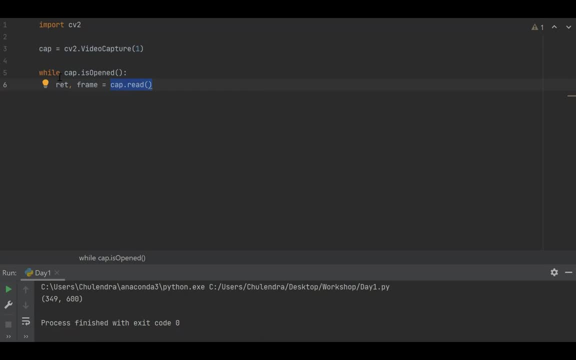 gives two, two tuple uh with two values, uh, return. very well, frame frame, the actual frame, right the, the image, image at a particular type, right? so rate value signifies. so it tells you whether, whether you, whether, whether, whether the frame is present or not, right, if, if, if, rate value is true. 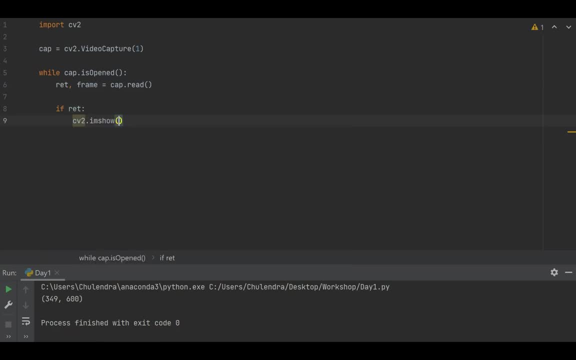 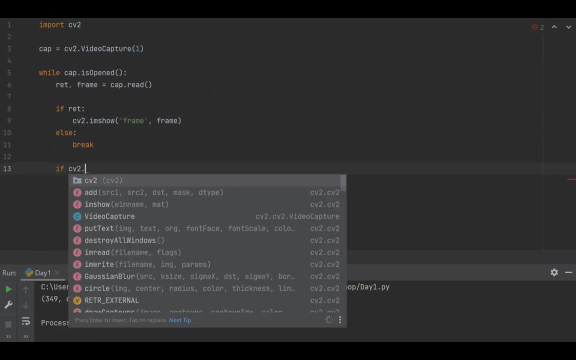 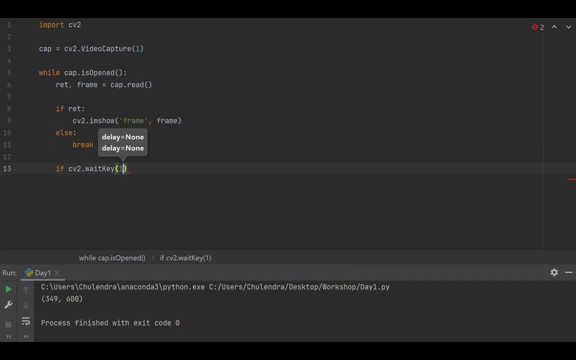 seem to, but ensure frame frame comma, same as we did for the image in the previous case, we are using again ensure function cvtteamshows the window name comma, the, the image array itself, then else if it is false, this row should break, also if there is another, if if cv2 dot waitkey. I put here one right. this I couldn't tell. 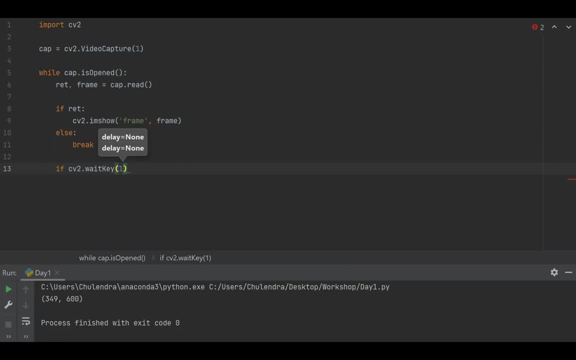 you about this waitkey function. there is some more thing which I had to tell you about that. This waitkey, so here, this one means the, the, the time, it time, it wait for the until the user image user user is present. key right, wait, wait. so this, this is, this number is in. 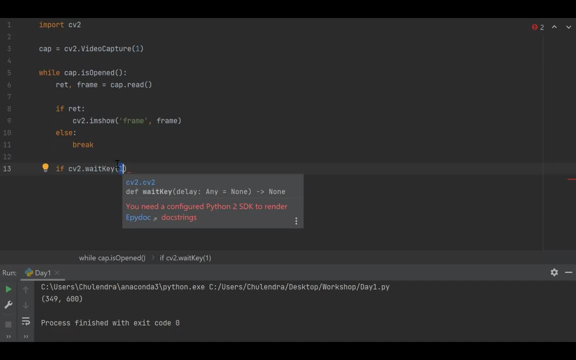 millisecond. so it wait but 1ms until user uh user token. so it question: wait for the user right? it'snah enter a key right, so previous time issue: zero, right zero means uh, wait infinite infinitely. right zero means wait infinitely. if you enter here: uh 30 millisecond. so it means that this. 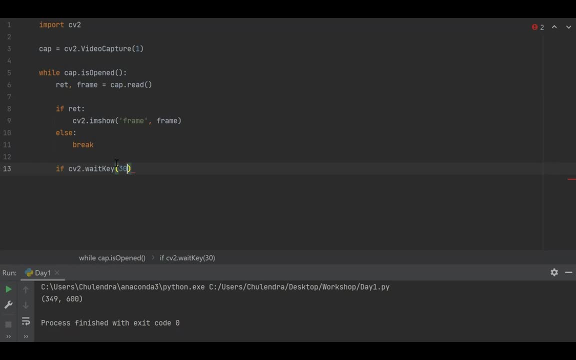 system. so so this system wait until user use a piece of key for a 30 minutes. so it wait for 30 minutes. 30, sorry, 30 millisecond, 30 millisecond, right. so wait, key 30 equal odd cube. what q? uh, i'll put here 27. 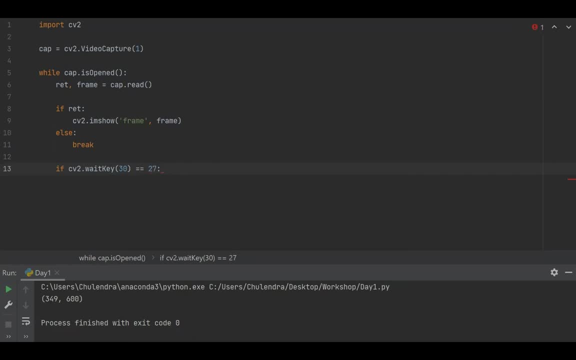 27 is nothing but escape the ski value of escape key. where escape key right then. okay, then, so that this mean if user press enter key, if user press escape key, this loop should break right. this loop should break right. then, after loop is is broken, capture object should be released. cap release. 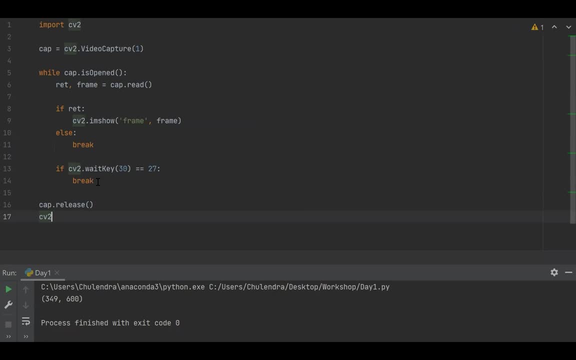 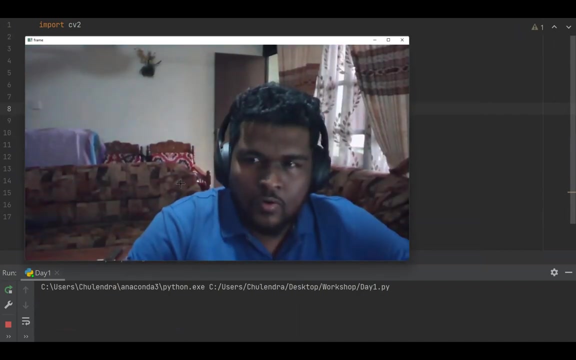 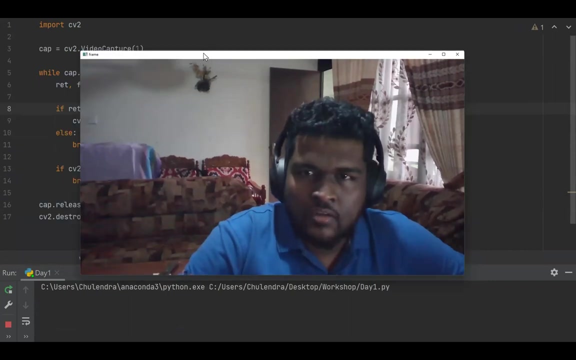 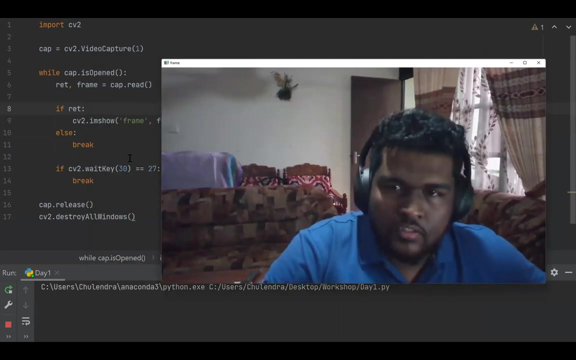 then this: all the windows should be destroyed. destroy all windows, right? so let's run this. so this is the uh webcam output of my right uh, so it waits, so so it wait. 30 millisecond each each time it take it wait, and 30 second until user enter. 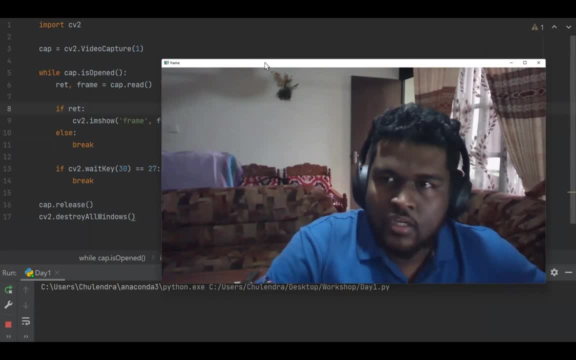 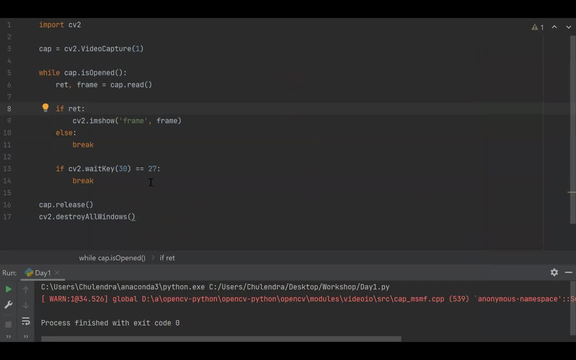 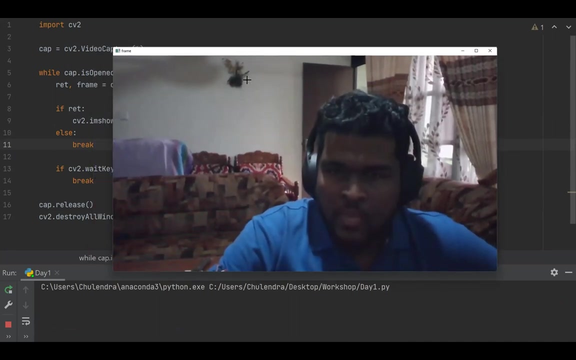 uh, uh, uh. escape key: right. so if you enter escape key, this will the- the windows will be destroyed. right. escape key, right, uh. so this is the uh, so this is the uh. The user is waiting for 30 seconds to enter a key. Then the next image appears: 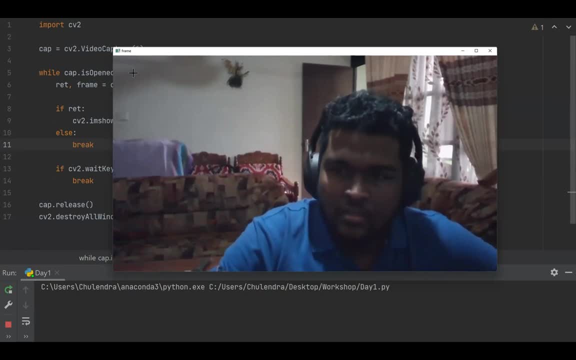 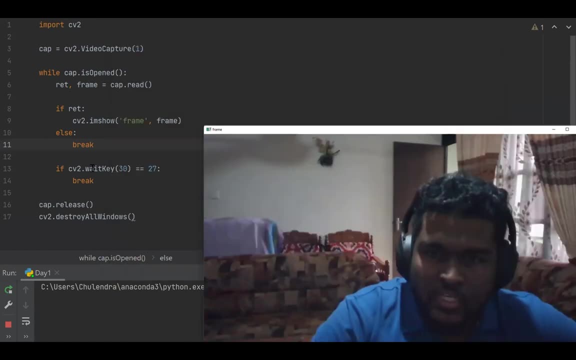 The user is waiting for 30 seconds, Then the next image appears. That's how it works. Then I return the value of cv2.waitkey. What is that value? That is the key to press the user. This cv2.waitkey function returns the ascii value of the key the user entered. 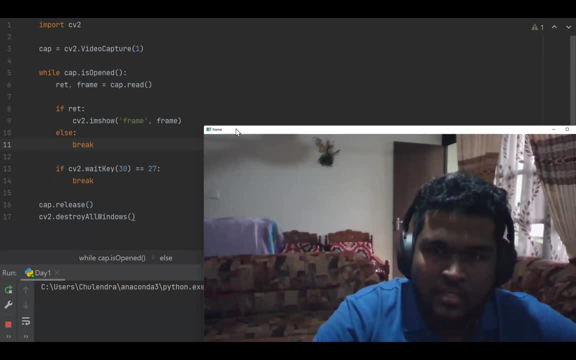 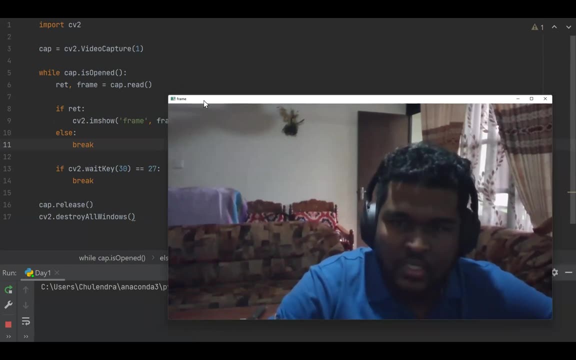 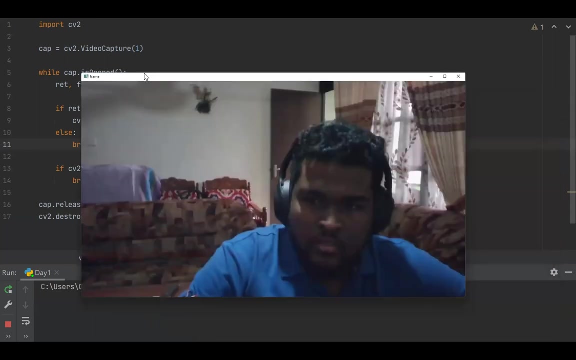 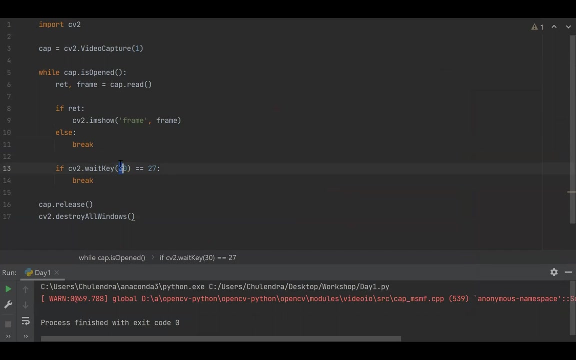 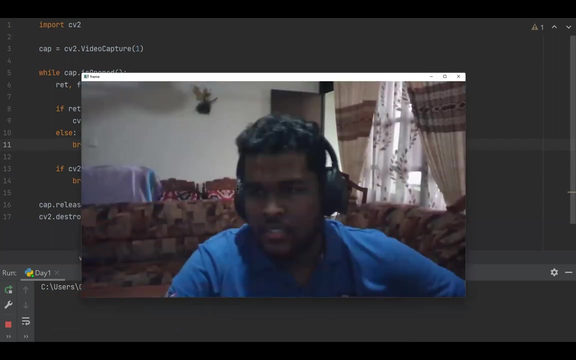 User pressed. The ascii value of the escape key is 27.. That's why I put 27 here. Okay, If you put higher than a second- something like 1000 milliseconds- that means one second. There should be a delay in your webcam feed. 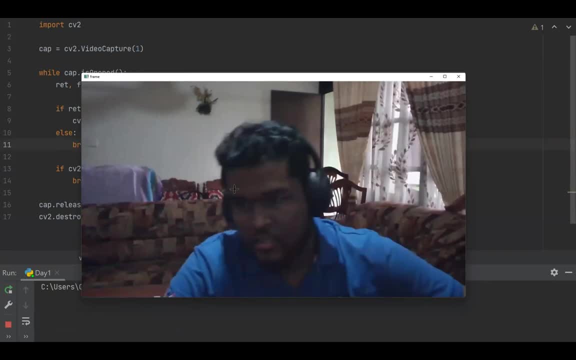 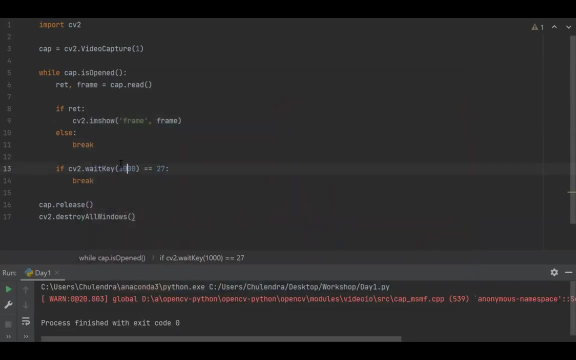 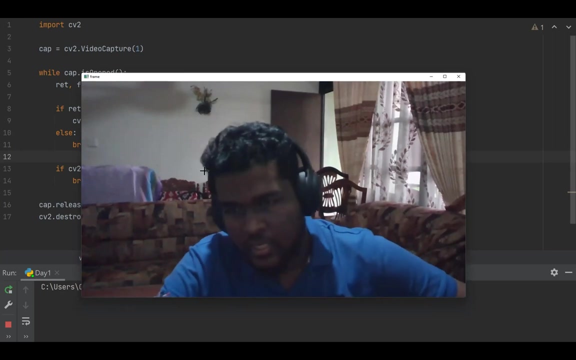 Something like this. I'm moving here and there You can see It only gives one frame per second Right. So normally a webcam has a delay associated with it. So even if you give one millisecond here, it has a built-in delay. 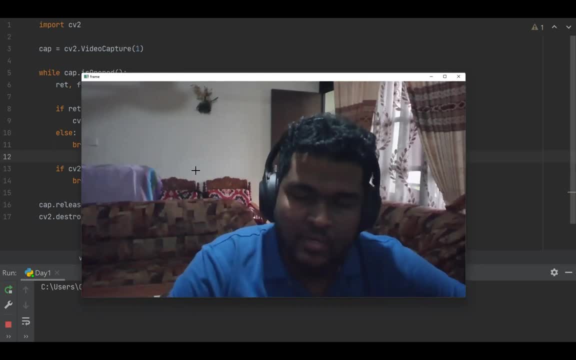 So normally a webcam has a built-in delay. So normally a webcam has a built-in delay, Is and has a built-in delay. So there is a built-in delay in the webcam slot. At that moment, every suspense can be the following as 1 millisecond or so. 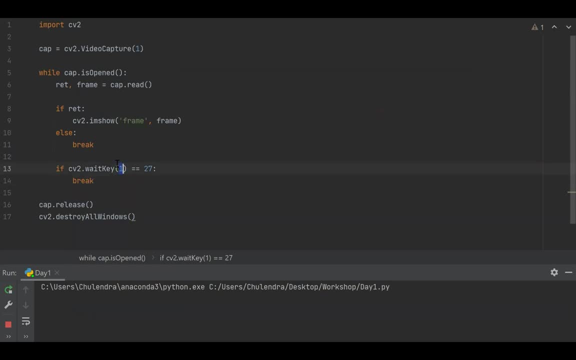 Even if you press cv2 waitkey, it generates an infinitely long delay with 1 millisecond. I'm moving in this text box to make this infinitely long And here is a θαqfj Shirin giving an infinitely long delay. 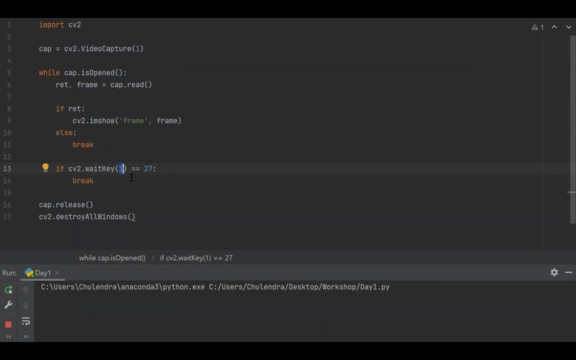 Just press the key. then If it is 1 millisecond it will look at it for another 1 millisecond. then it will think that if it is 1 millisecond it will not play it fast. That's not the case. 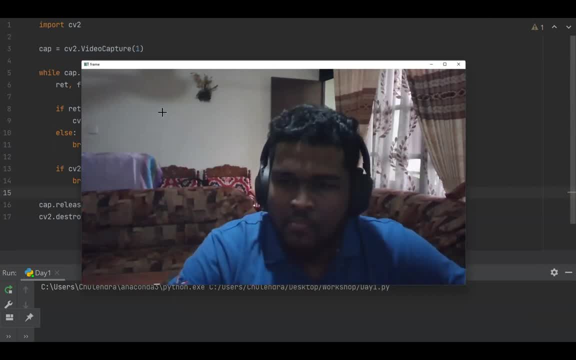 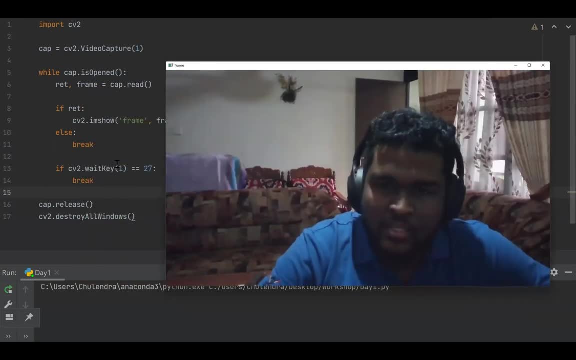 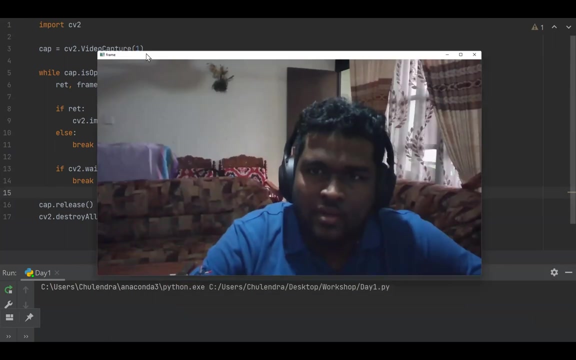 The delay in the webcam is 1 millisecond. when we use the webcam We are using 30 milliseconds. so when we play video, it will look at 30 frames per second. When it plays 1 millisecond, it will look at it for another 1 millisecond. 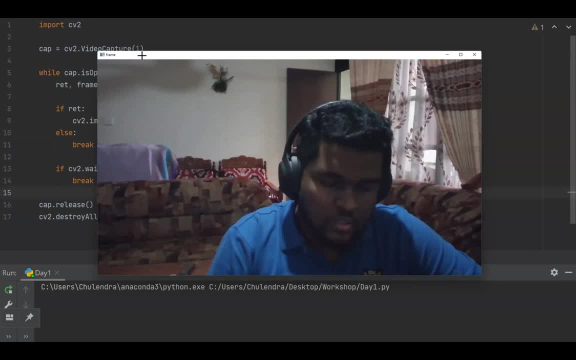 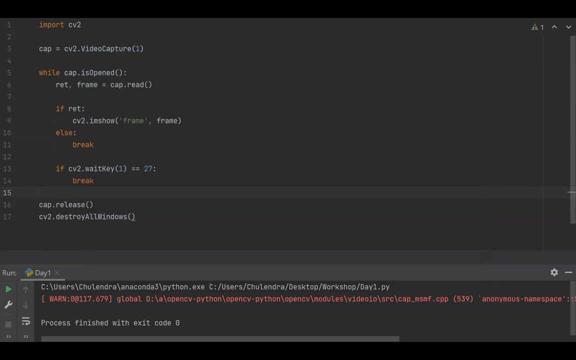 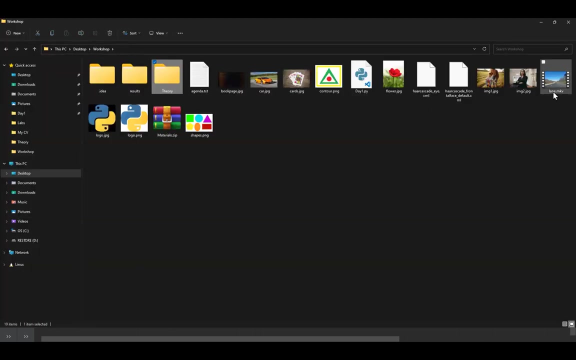 Now it looks at it for another 1 millisecond in second. 30 second is the ideal gap between two frames, right? so if you downloaded my materials, they are. there should be a web video, lanemkv, right? so if you have, if you have a another video, you can use that as well. so i'm using this lanemkv file. 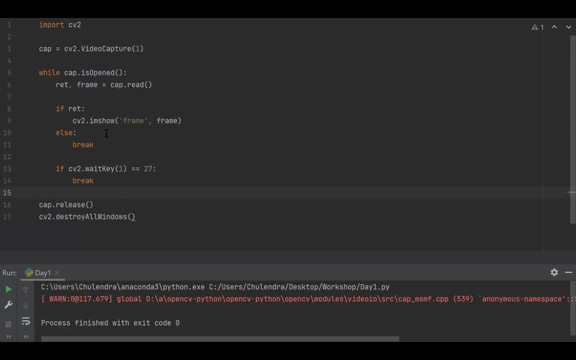 so this lanemkv file, so you can enter this lanemkv file to this right as a string. lanemkv- right, so if i run this, so it plays very fast. right, because the the delay between two frame is one millisecond, right, so if you enter 30 millisecond, so it plays fine. 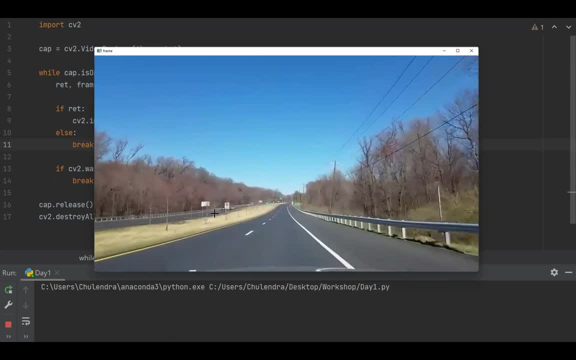 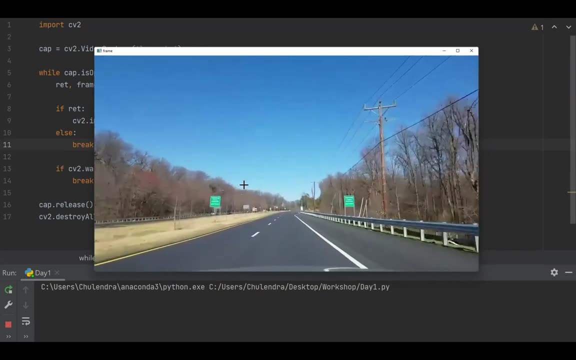 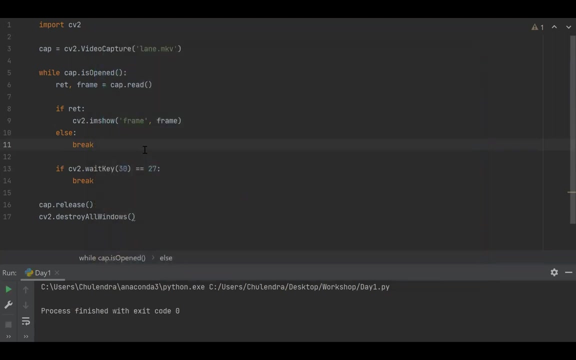 so this is the. i think this should be the ifm fps for this video, right? so if you, if you enter escape key, then the loop will break and the capture object is released and videos are video. all the windows are destroyed, right? so here you can. if don't know, 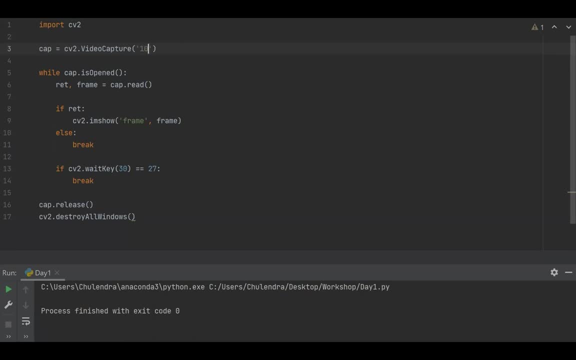 so you can, even me, you can even use your ip camera with this video capture object. i'm using this lambert mkv file. then suppose if you need to break this loop, if you center the, the, you center the q button in your keyboard right. to do that you have to use odd function, or q. or q returns the sq value of this. 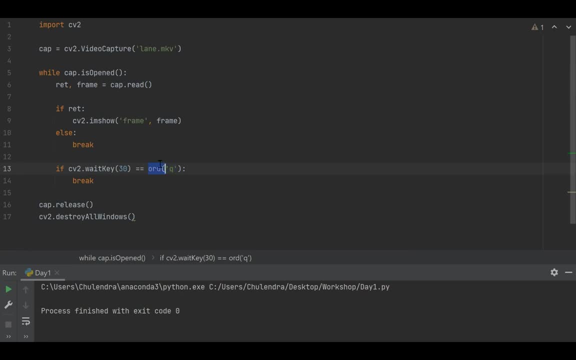 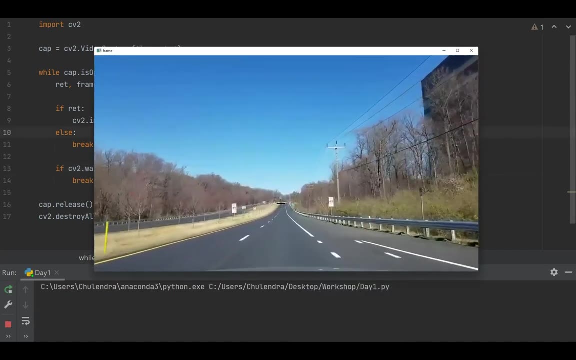 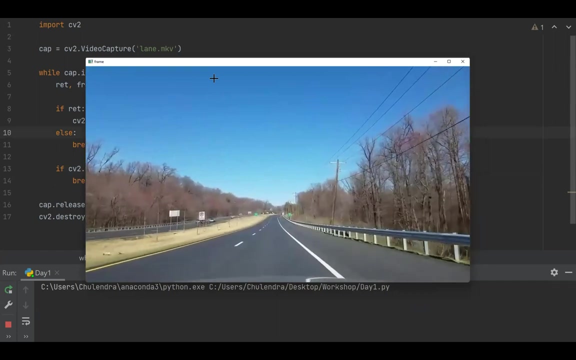 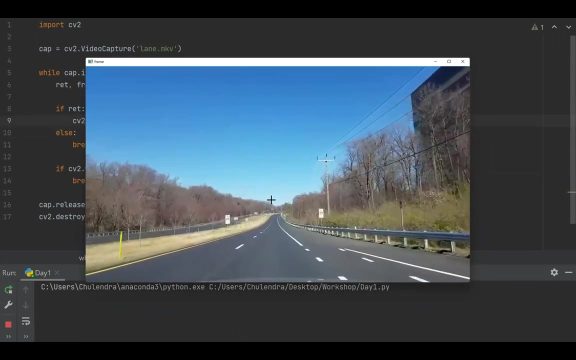 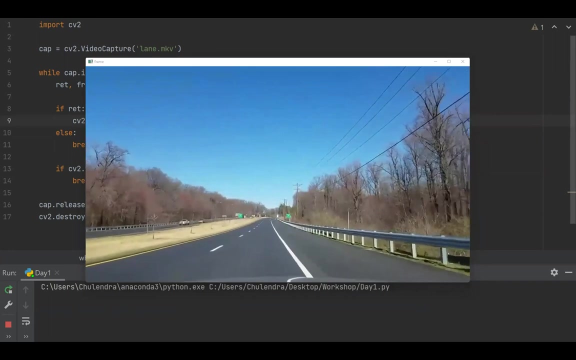 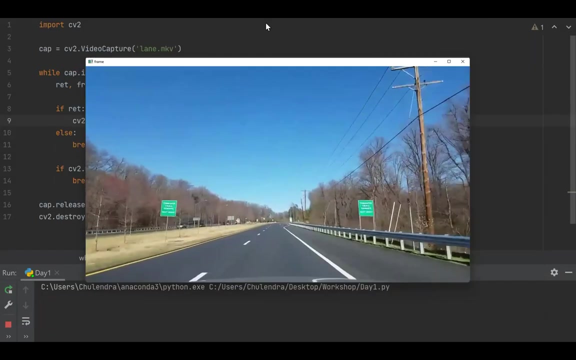 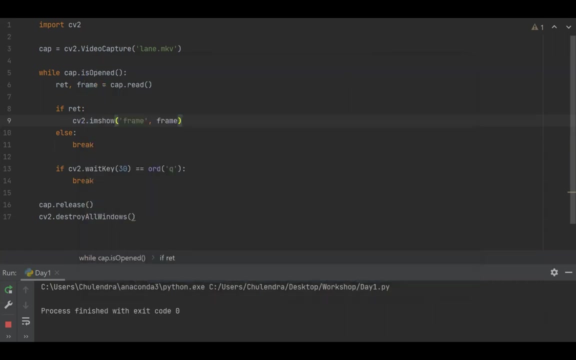 character right. so then if you run this, so while q q about it that i make a destroy window. there is a question, sir, can you please explain the functions in the while loop? okay, so first we, we are creating a video capture object right, cap object cap, uh, called cap right. 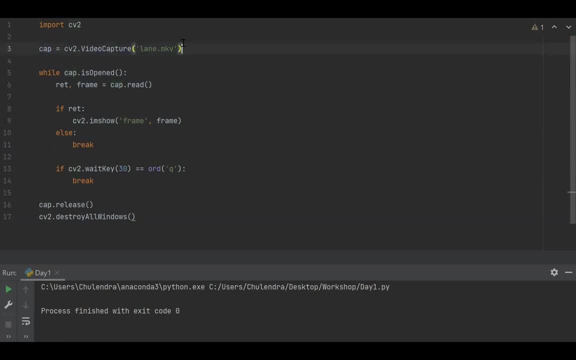 video capture object. right, so this is where you will link your media to this object, right, so cap object. then, as strong as this cap cap object object is open, as long as it is open, we are performing this function, this call, The first function. what it gives is capread. capread means reading a frame, reading a. 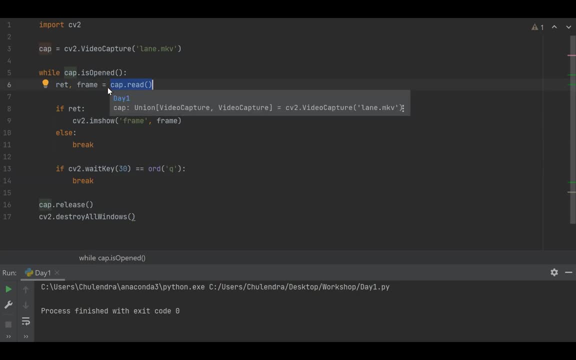 particular frame at the current time, capread. so it is just reading a frame one by one. So it gives two values: return value and frame value. Return value is the indication whether there is a frame or not. If there is no frame, 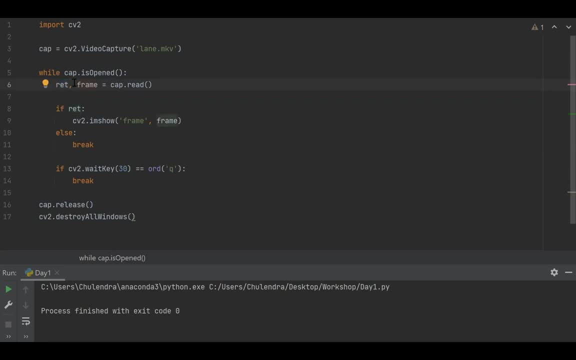 If there is no frame, this rate value is false. So this video example. so what happened is so it reads image, read this cap object one by one and after the end of this video, the rate value is false. The capread can no longer read any frame. 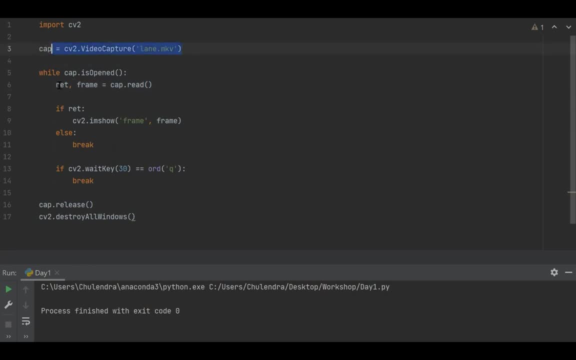 So it has to read the frame which is in this lambda mkv file, So rate value will be false. that's why it will break the loop. So if I put one here, so this will run very fast and the window was destroyed, right. 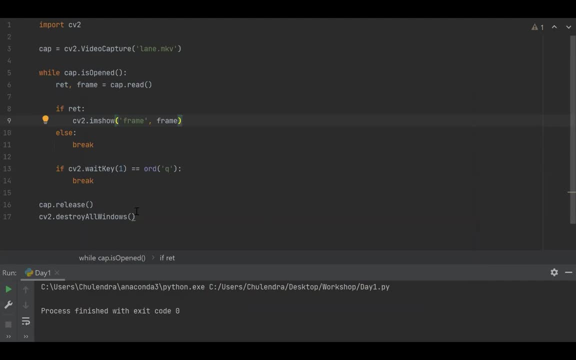 How it destroyed was how it was destroyed. How it was destroyed, right, How it was destroyed, right. So let's try it again. it destroyed because the rate value was became false, rate value became false, return value became false. that's why this whole window was disappeared, right? so as long as there is a return value, 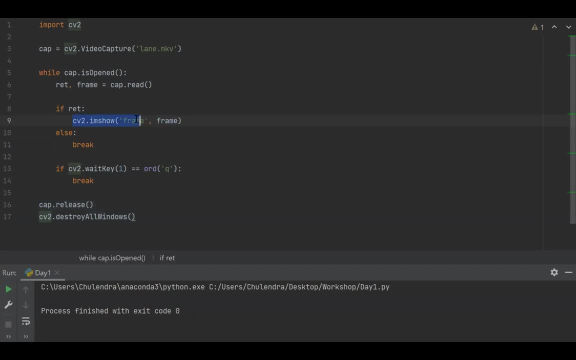 we are showing that particular image as in the frame in the window right. as long as this return value is true, we are. if this, sorry, sorry, if this return value is true, we are showing that image frame window right. if there is no, any return value, let me return. sorry, return value is. 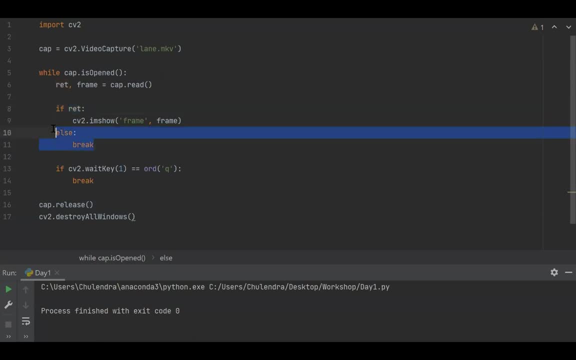 if the return value is four, the route will break. and also we are checking, uh if, whether whether user is pressing q, here in this case q, whether user is pressing q, right, we check whether user is pressing q with one millisecond delay, right? if user user is not not is not pressing any key, it will return minus one right, of course. 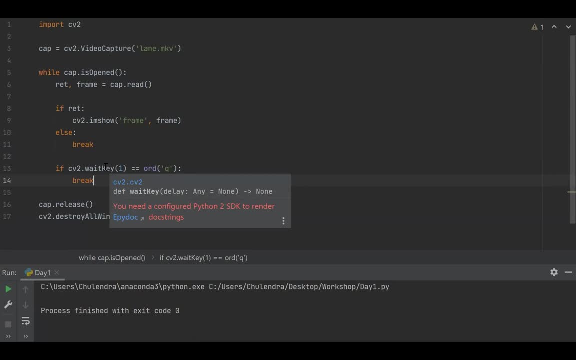 is not there, right? if? if the user is not pressing any key within one millisecond delay, it will return minus one, right, so minus one, right. so. so i have a question, i have a question i want, so, uh, so, so what is the change that we have to do? uh, if you suppress any key other than q, 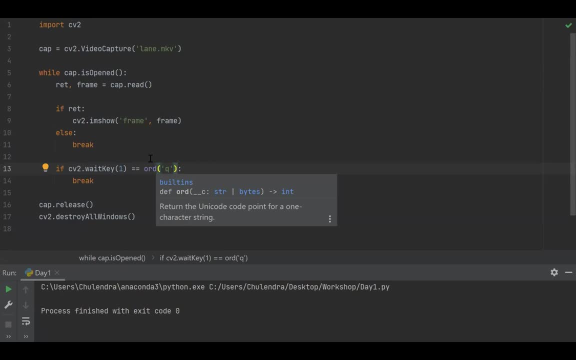 right. if you suppress any key, sorry, not other than q. if you, if you suppress any key on your keyboard, only on. if you suppress any key on its keyboard, we should break the loop, right how to do it? if you have any idea, you can post it in the chat. 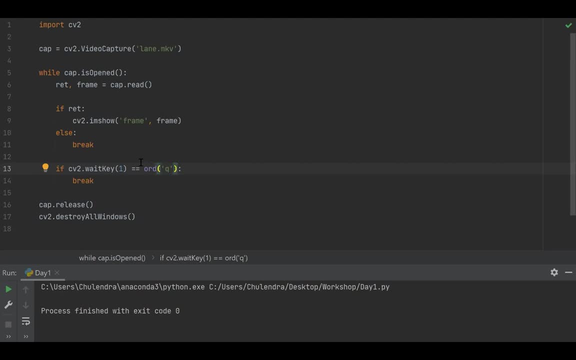 what is the? what is the change that i have to do in this slide? if you suppress any key, any key right. any key on the board, any key on the keyboard right. if you suppress any key on the keyboard, i should be able to destroy this loop. right, if you suppress any key on the keyboard. 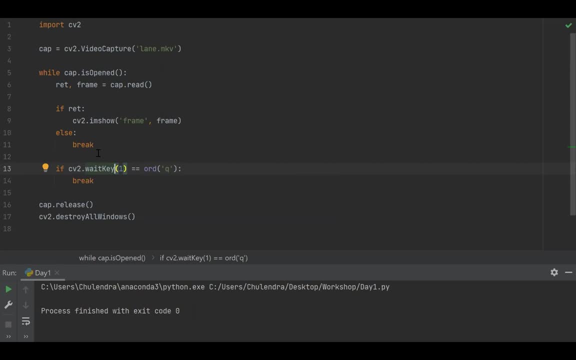 this: uh, destroy this file. i should be able to break this file loop and destroy all the windows, right? so how to deal? can someone? yeah, yeah, good, very good, uh, weight keys. is not t equal to one minus one? yeah, that's the answer. we can check if the weight key is greater than minus one. greater than minus one, yeah. 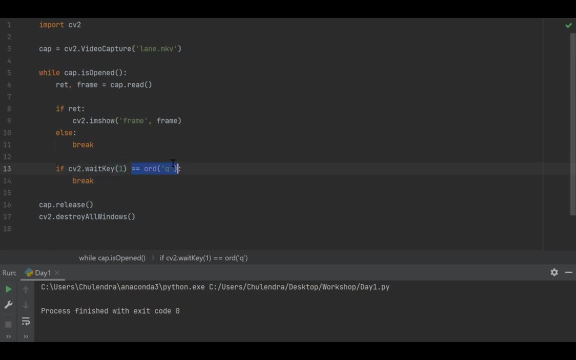 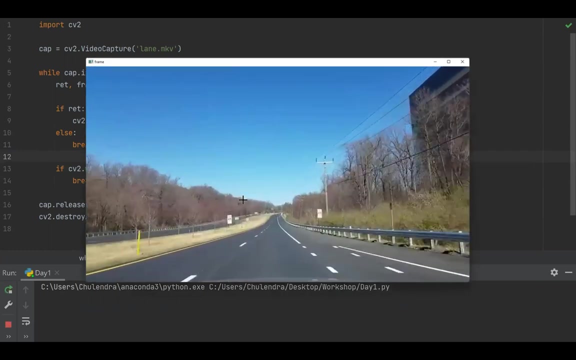 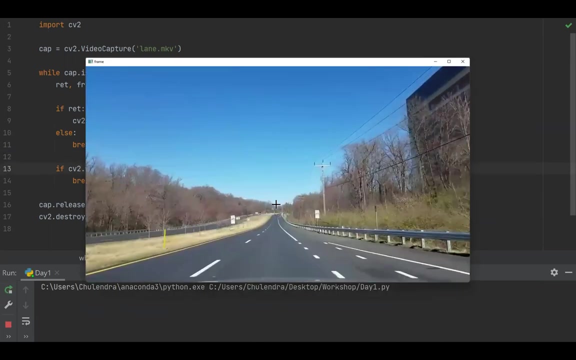 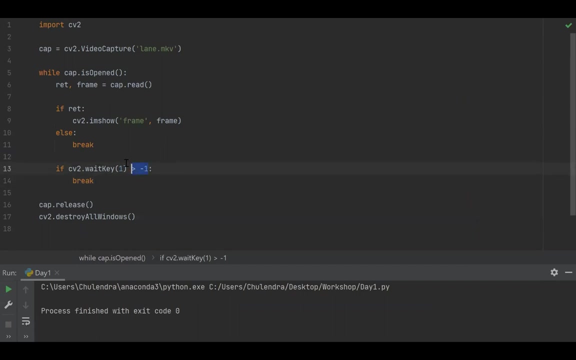 greater than minus one. it's also, i think also, it's also it's also okay, i think. let's see, yeah, it's also working right now. yeah, it's also okay. yeah, that's good, that's also correct. yeah, i usually do like this: not t equal to minus, right. 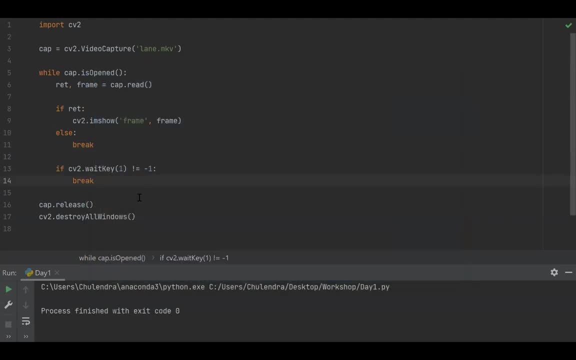 yeah, i think, i think you are okay with this simulated weight key right, the function of this basic, the underlying principle of this version of this weight key right, uh, okay. so if i also, um, i'm again going to read my webcam one, i'm going to use the first webcam of second webcam of my my. 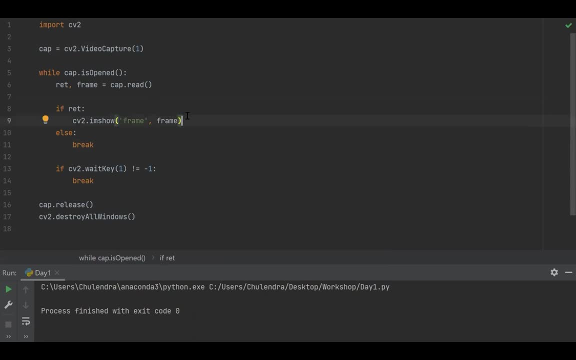 if i uh, if i need need the gray image also, i can do it like this: cv2 dot. there is a function for cv2, cvt color here. first you have to enter the image, so in my case frame comma, then uh, code, code me: cv2 dot bgr. 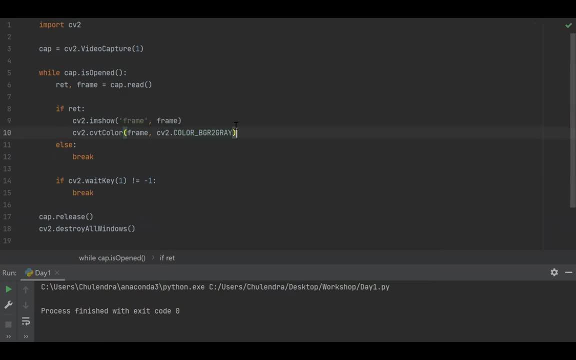 to gray code me: cv2 dot bgr. to gray code me: cv2 dot bgr. to gray right and i'm i'm also showing this gray image, also right, gray. sorry, this should gray. so this is the color color db colored image and this is the respective black and white image. 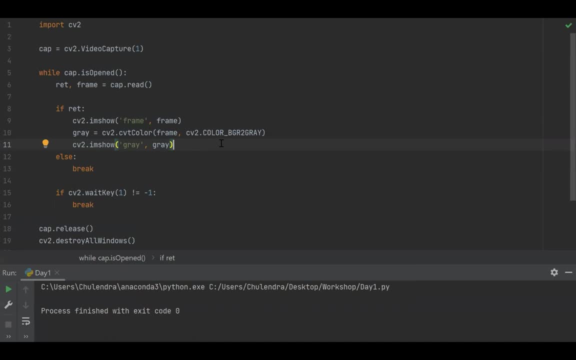 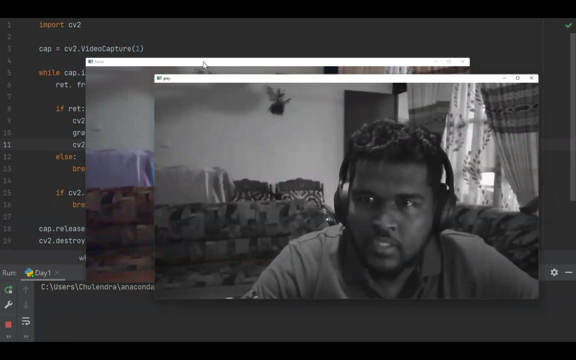 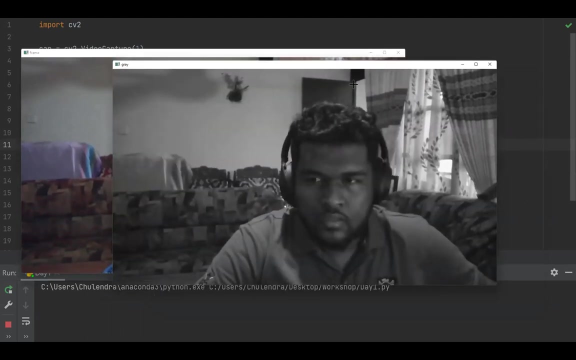 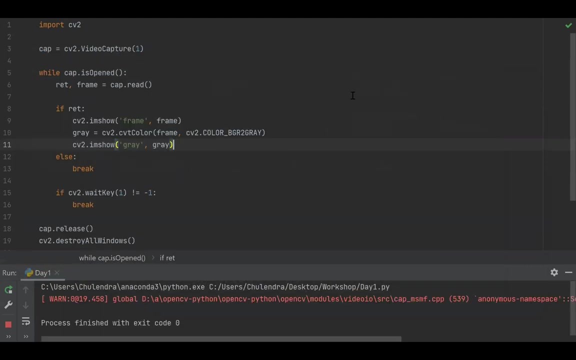 respect to gray scale image, so let's run this right. so this is a gray image. this is a colored image, so we- i can press any key to destroy this windows. okay, so if this also in your mind, cv2 dot convert color um. we are using this in later sessions also. 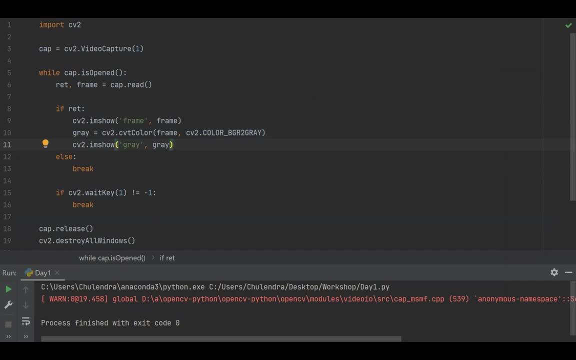 uh, um, um, um, um, um suppose if you need to resize the frame given by the webcam right, you can do it by simply cap dot set three. three refers to the frame with, frame with. you can enter frame with- I learned we are the autonomy frame with the height to have the identity resolution. 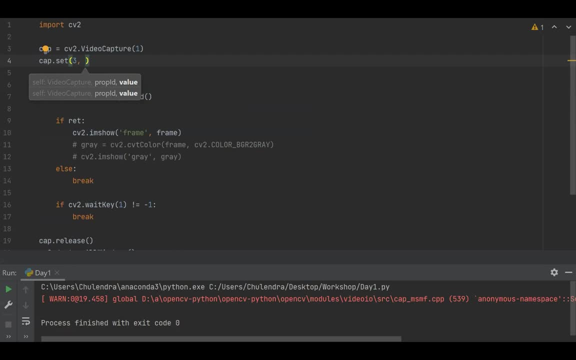 when I make a resolution, then the feed of the webcam. I have to look at a specific resolution. here is my full HD resolution. then I have to look at a lower resolution webcam feed. then there is a program. there is a program in this program to support the webcam. 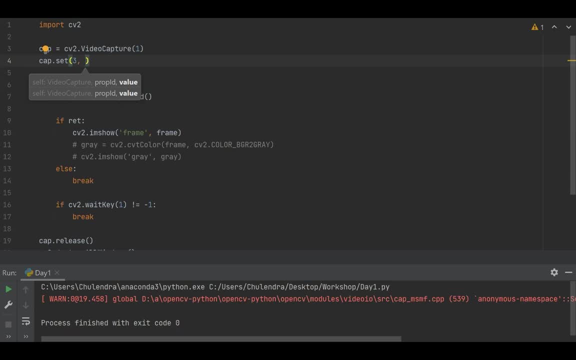 in this program. there is a program to support the webcam. in this program. resolution has a little bit of a key. that is why this is not the right solution to all of the webcams. there is definitely a resolution if you are using this method right. webcam has supported resolution set right. 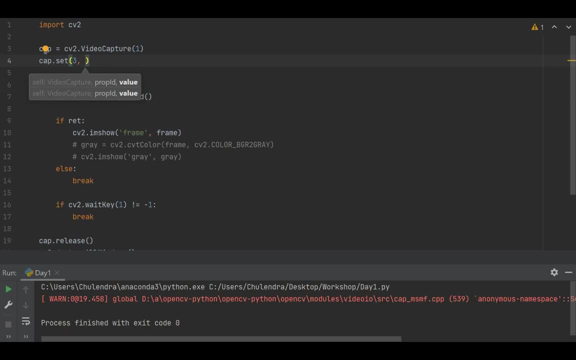 so now what I'm going to do is I'm going to resize the image given by the vector. right, so there are set of resolutions supported in your webcam. right, so we only choose such resolutions. i'll enter 340. i don't know whether this work. let's see. 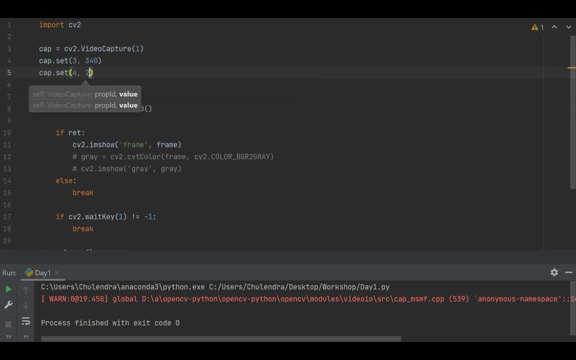 there is one more question. yeah, can you explain? second variable: pass to conduct color. yeah, so this variable, yeah, this variable means color bgr to gray, right, that means so i, i first, in the first, first, first of all. i said first time, mister is itself. i said the image in open cv is red, dash bgr. 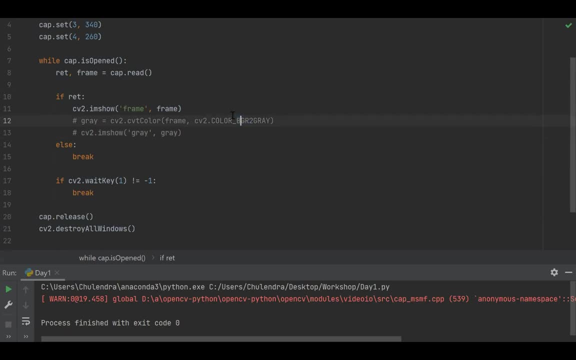 the channel sign bgr order right, not rgb right. so bgr, so color. bgr to gray. so this is a conversion conversion pattern. right order bgr to gray. so this is a flag color bgr to gray, right, so cv2.color bgr to gray. so later we convert bgr from bgr color space to: 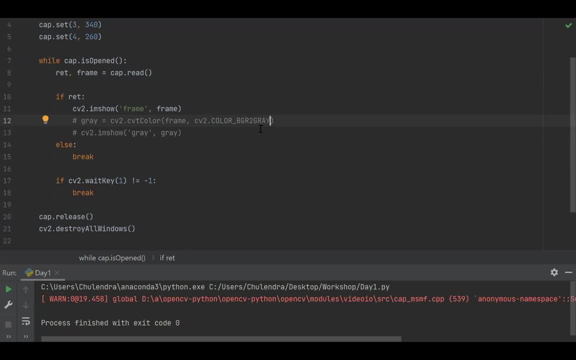 some different color space, like hsv right, so in that case bgr to hsv, hsv right, for in this case bgr to gray. gray means day scale. so if you are, if you want to convert a particular frame, particular image into grayscale image, you have to issue this flag c into both. 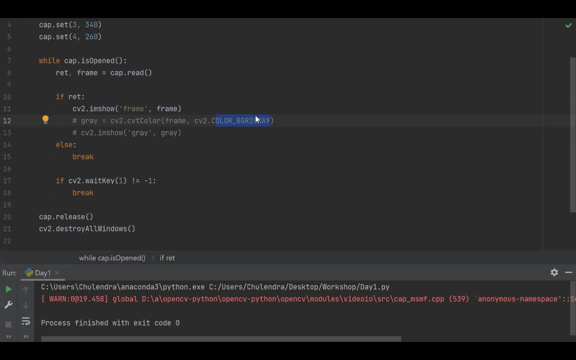 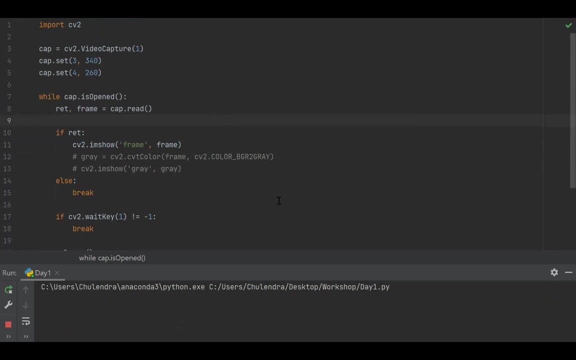 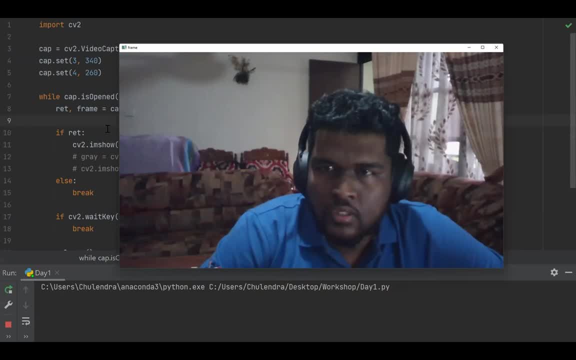 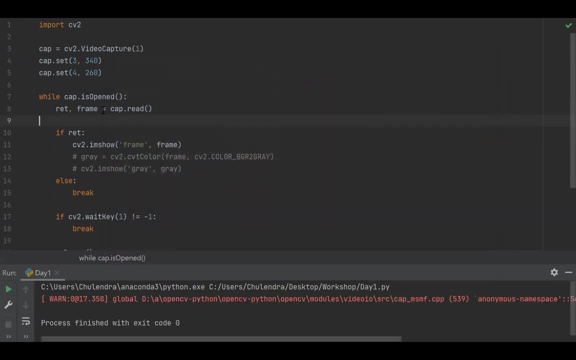 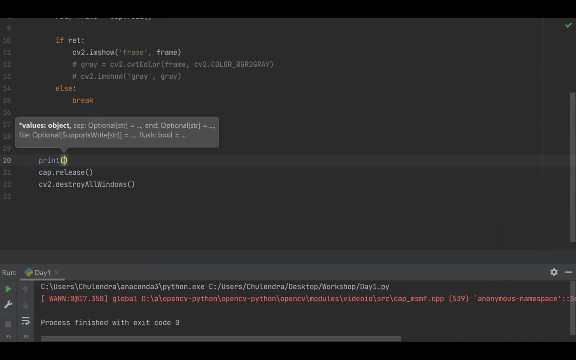 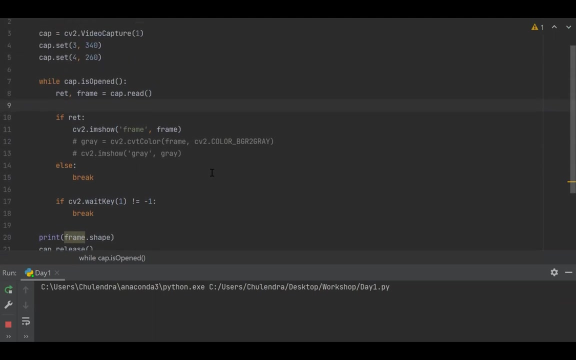 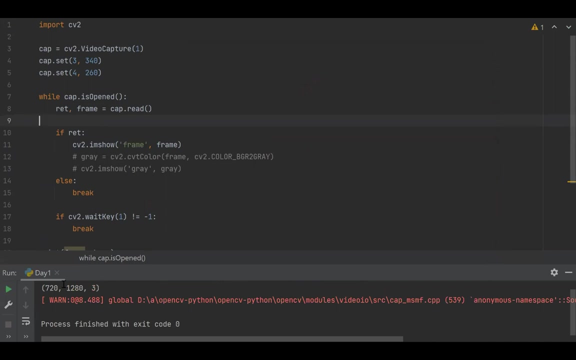 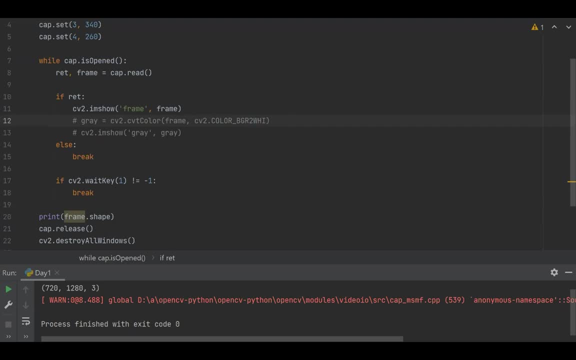 white. You can't use VGR to white or something. there's no such thing. VGR to white? there's no such thing. Only this color VGR- there are a bunch of. there's no such thing for VGR to red or something. 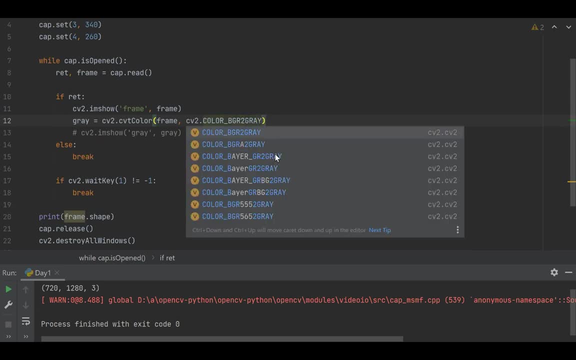 right. VGR to gray means grayscale. There are lots of VGR to conversion. I haven't used all of them. I only have used VGR to gray and VGR to HSV. HSV is a different color space that we are going to talk about in color detection section. 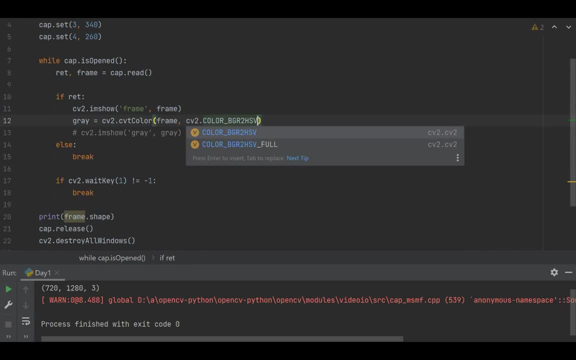 Right, So So Okay, Keep it in mind. gray means nothing but grayscale. grayscale means backhand white. Okay, I was seeing this tree means. this tree means cap frame. with you cannot see, You can see it clearly, right. 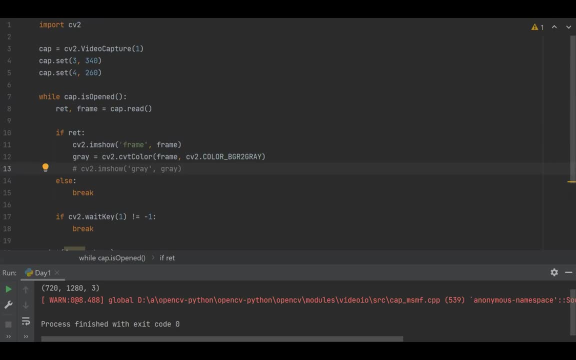 Okay, It is, It's just. It's just. you can either use trio- you can pop this analysis instead of for for me. so to see you, tutor, seem to do right frame width and frame height. also, you can pass 3 & 4, 3 & 4, right, there are a set of numbers and the top legs associate with it. 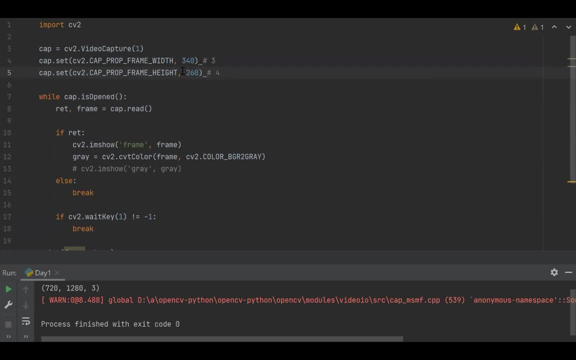 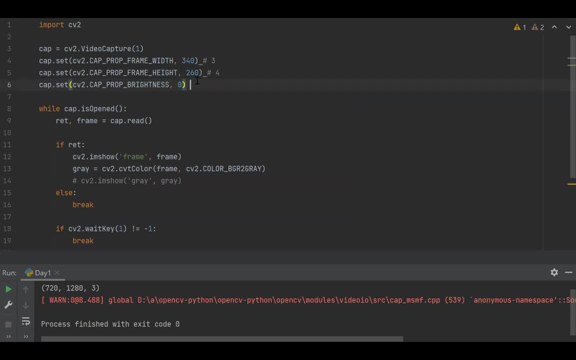 what 0 means 0 brightness mean and mean what 0 means 0 brightness mean and mean. let's see what it gives so you can. let's see what it gives so you can. let's see what it gives so you can entertain here instead of captain can. 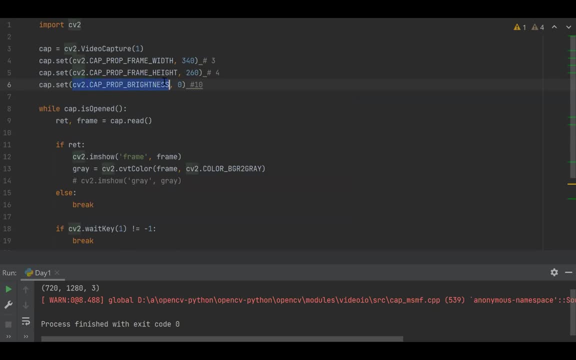 entertain here instead of captain. can entertain here instead of captain. can don't cap from brightness instead of don't cap from brightness, instead of don't cap from brightness. instead of this, mister you can pass, then here. let's this, mister you can pass, then here, let's. 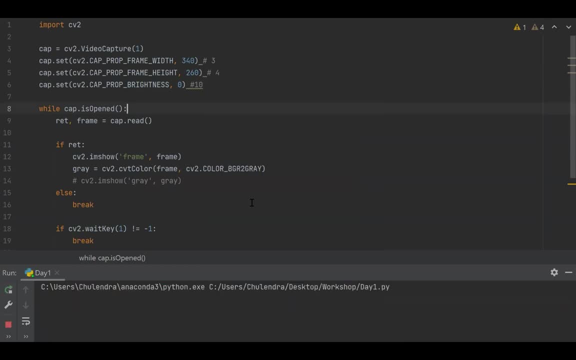 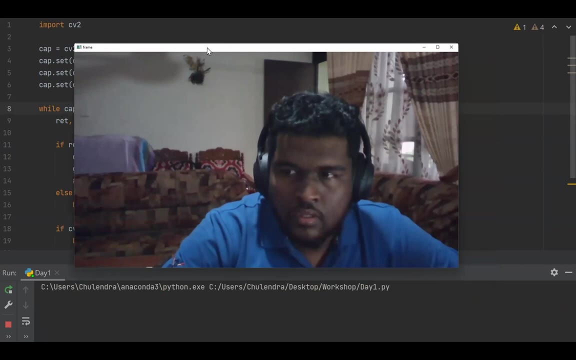 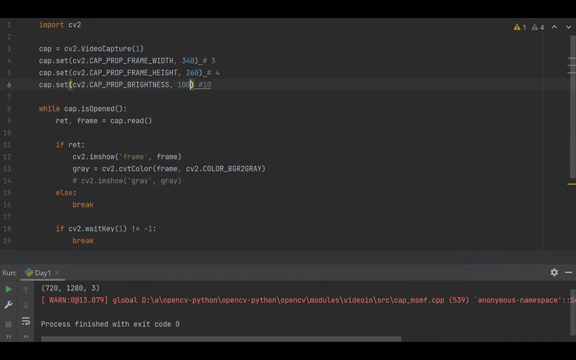 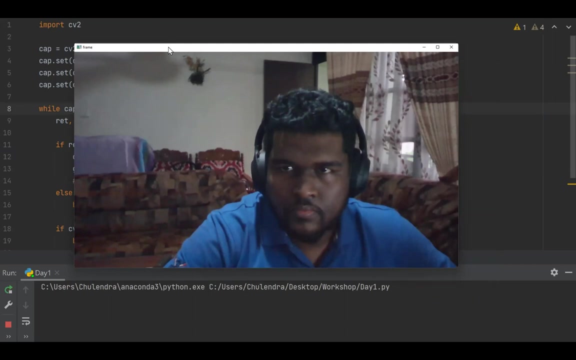 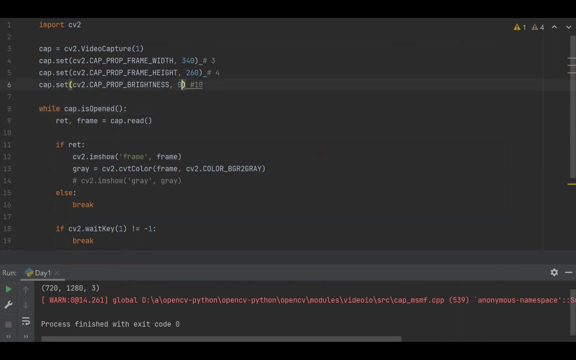 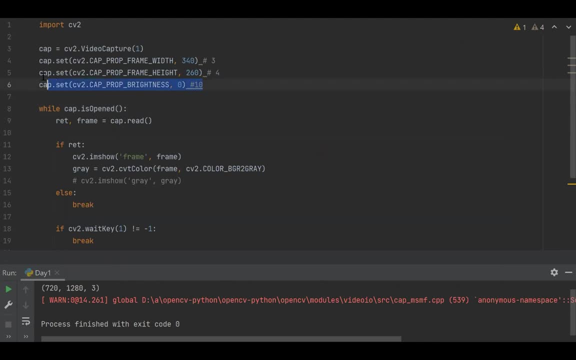 okay. I just just said that we can. I just okay. I just just said that we can. I just okay. I just just said that we can. I just fight this here. why doesn't make him fight this here? why doesn't make him fight this here? why doesn't make him change? 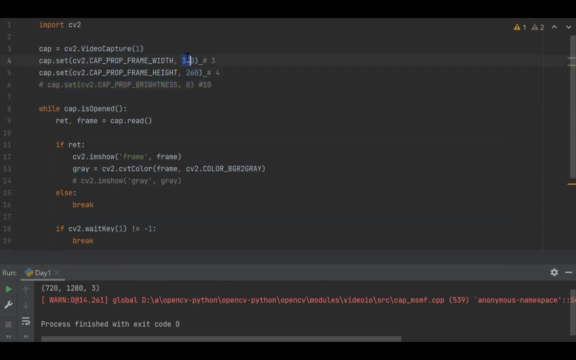 when it's coming it out, so here you can. when it's coming it out, so here you can. when it's coming it out, so here you can pass the solution and high resolution, the solution and high resolution, the solution. and high resolution desire the solution. so on location. 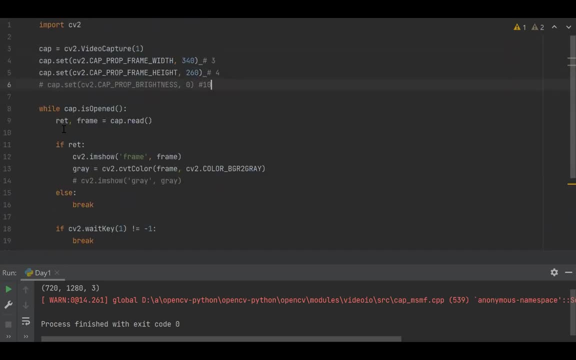 on location. on location: bone, bone, bone. yeah it. let me, Sir, uh, red, signal, right that that indicates whether there is a frame or not, right? so if i print this rate, so let's, let's bring this rate. return value, so let's bring this and let's run this. 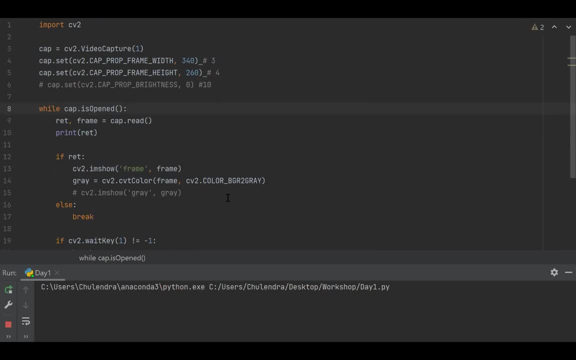 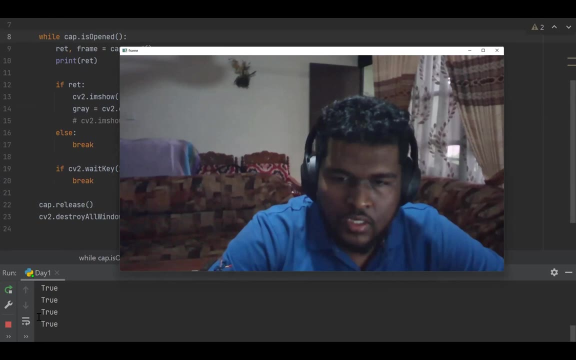 so you can see through through each printing route right in the down through it, through through. there is a frame right, frame and frame and frame right. if there is no frame right, you should return false, but in this case you should each if it is not returning false. 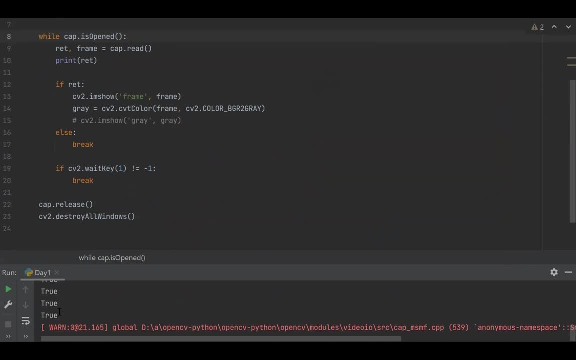 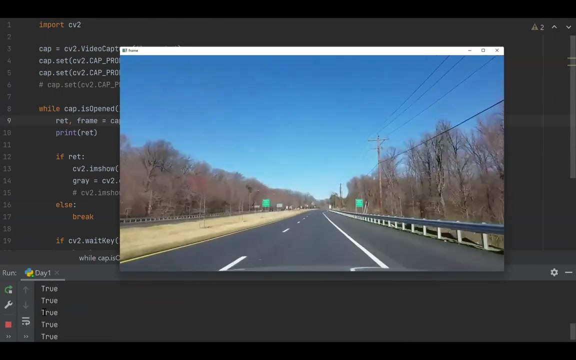 uh, if there is no frame, right, you should return false. but let's, let's say let's choose that lane button k, because there is no ending webcam, right, the end marks after we, after user in enter key right. so let's run this so through through, through through. ultimately there should be false. 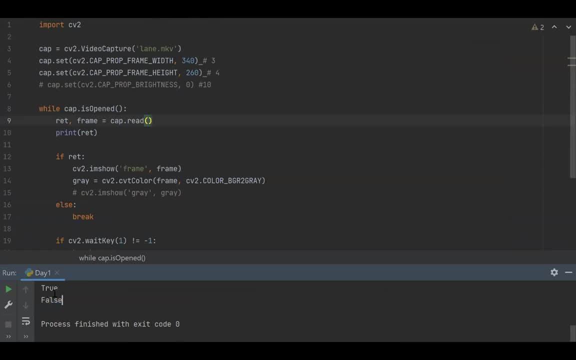 false, right, false, this. this is the last frame, last frame return through, right last frame and it returns through and it, uh, it then again continues the loop and again cap is read red and new frame is null. null frame is generated actually, none, none, none, none type objective. 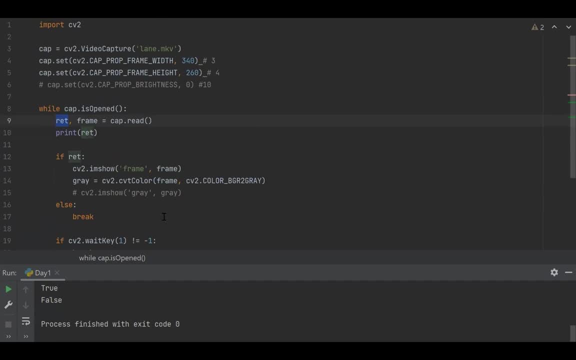 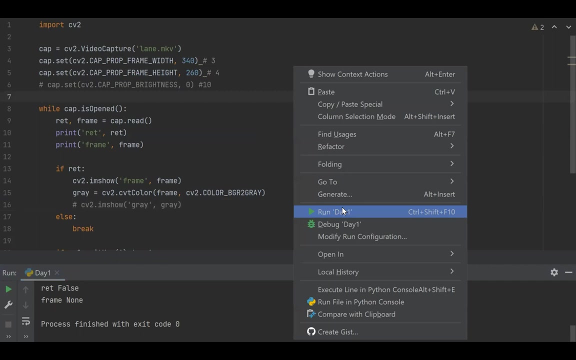 returns here and zero returns right. so if you print a comma frame with comma, i'll, i'll put like this this: this is raster right. last frame is none, none and false. that's how, uh, this low loop, break loop first, broken right. androp lost up, uh. 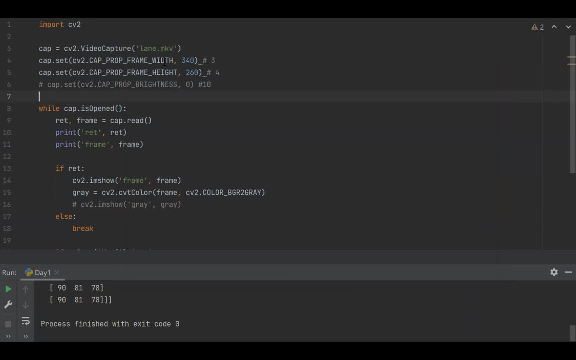 you can change right now when you log in, uh to raster this resolution here, but i'll i'll show you one more with one method, another method to resize your image, right other than this. you can play with this right. so let's see how to resize the image while coming this out. 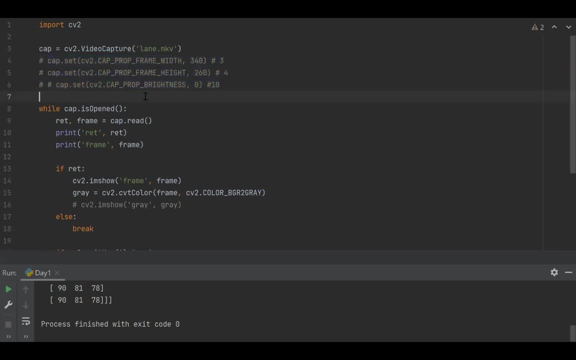 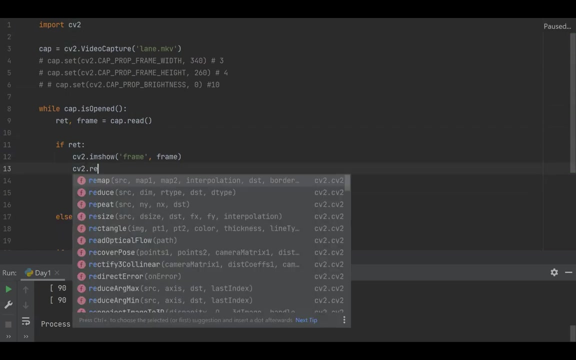 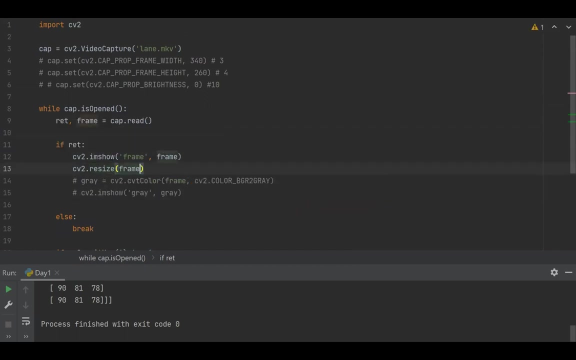 so okay. so there's method called resize, cv2 resize, so i'll resize in this frame before the. let's first first. so this: here we have to put a tuple. uh, it should be. uh, you should first come with with and then have the tuple if you want to do whatever you want. so here we have to put a tuple, so that's. 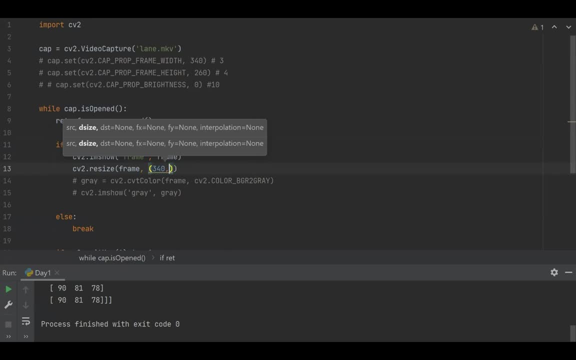 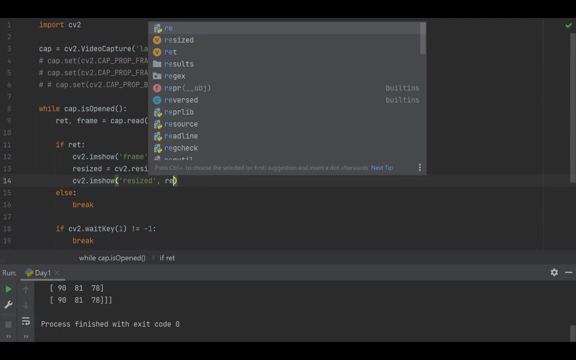 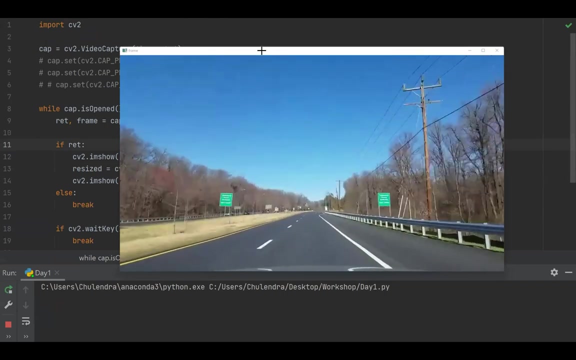 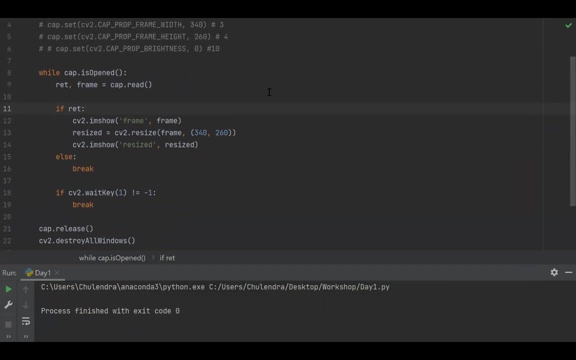 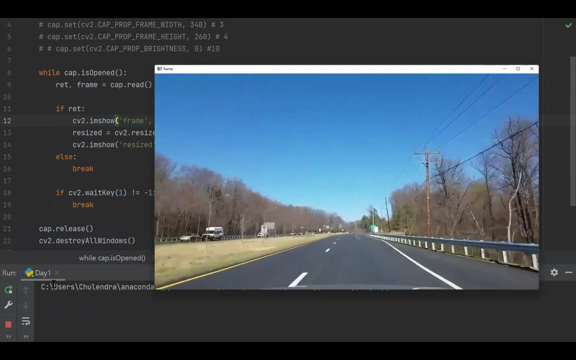 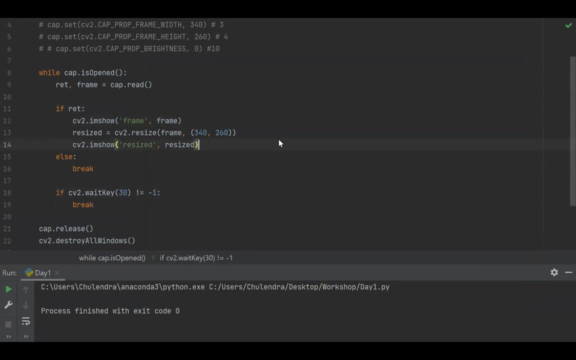 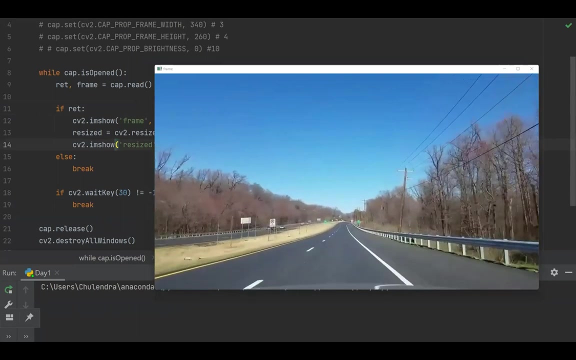 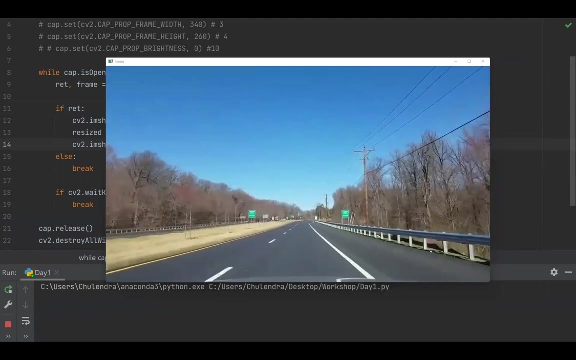 i will select 340 as width and 260x height, right, so so this is precise. this is my research. let's resize. this is that's my research image i- i haven't sure where is my research here here. here the resizing image. right, so that's how you are resizing the image. 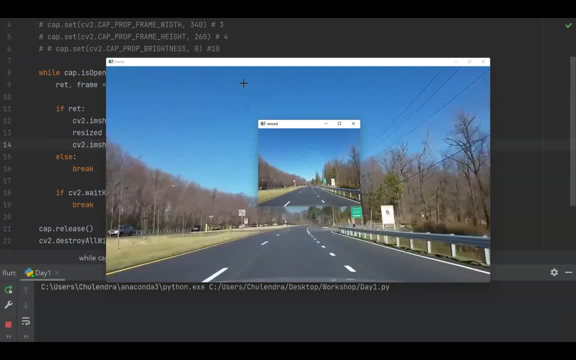 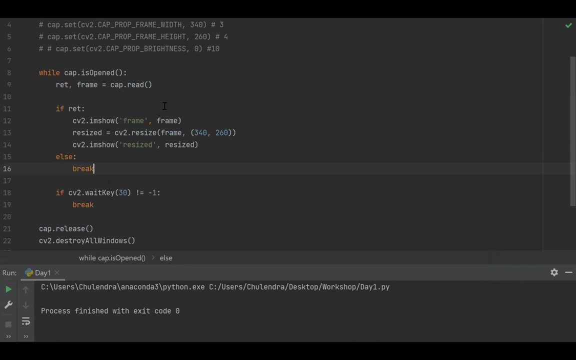 so why? okay, so first you have to put the frame right- image- then you have to enter dimension, uh say resolution, resolution of the desired resolution. your solution that you want to resize this is: this is my desired resolution, so the image will be resized to 340 times 260.. 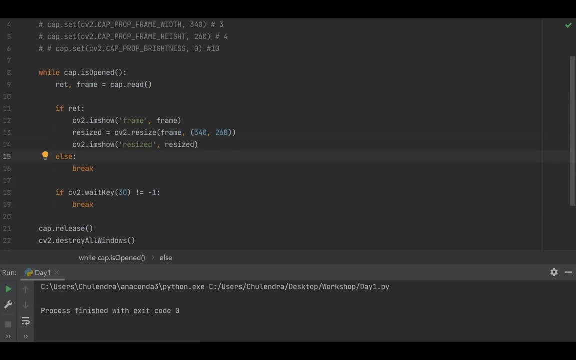 right, yeah, so that's about resizing. uh, okay, let's again read that call means it type, and then you can see that it's a very good look at the list so you can see that this is my last page, so i'm going to go to the next page. 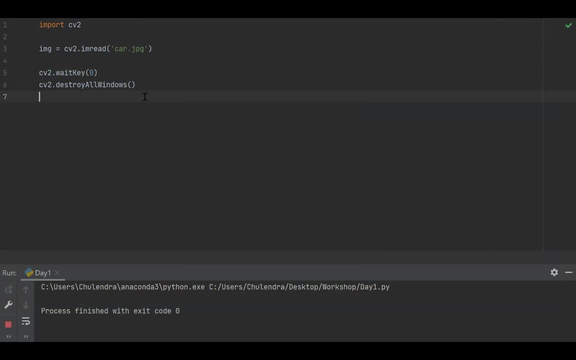 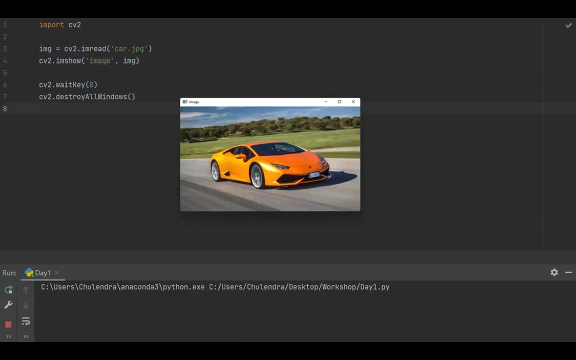 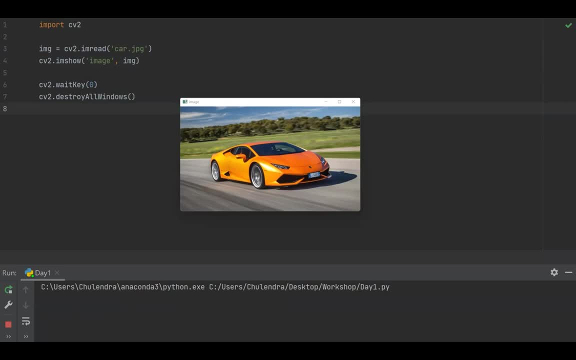 does the resize change pixels so? so i see millimeters, so i see millimeters. Resize change pixels. it is the values used in pixels, so it will change the resize function and we will get the pixel values, not the millimeters. We need to change the resolution of the image: width, height. 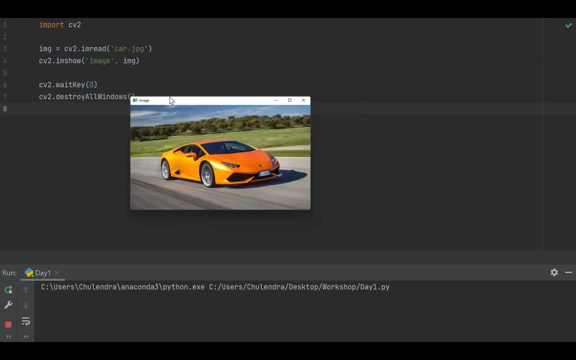 Now we are going to change the color of the image. We need to change the line. Now we are going to increase the size of the image. Now we are going to increase the size of the image. Now we are going to increase the size of the image. 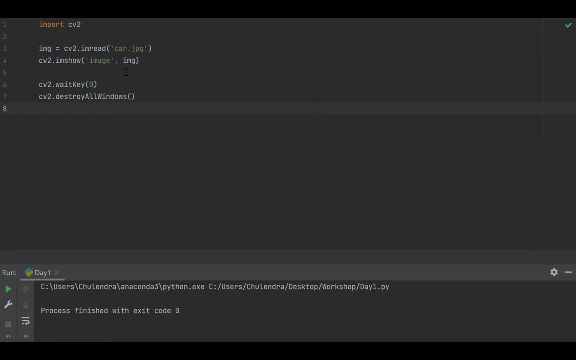 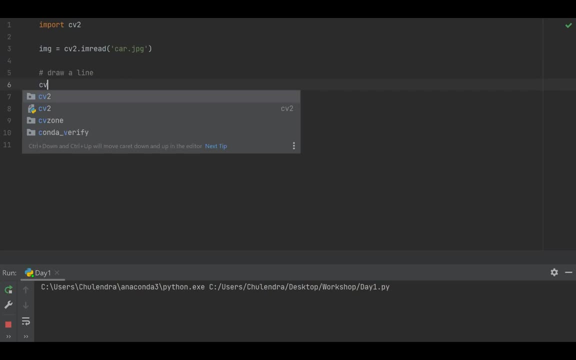 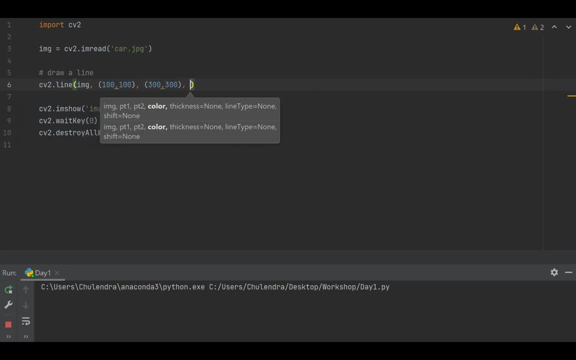 with comma height And I'll. so this is the color 255.. I'll put a white line. So you see it is 255,, 255,, 255. Then color is color. is that then thickness, Thickness, let's say 15.. 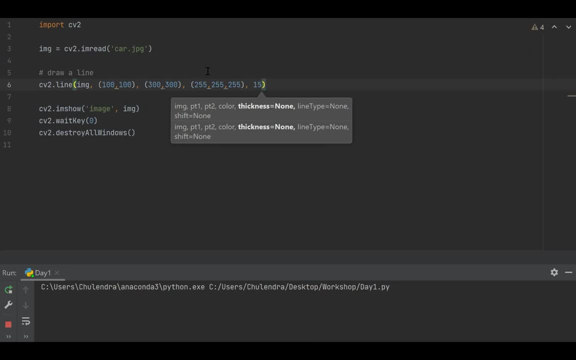 So it is in pixel, Thickness is in pixel, So let's run this. This one right, This one right. That's a thick line. Now look here I've written 100 comma 100.. Here, 100 comma 100 coordinate. 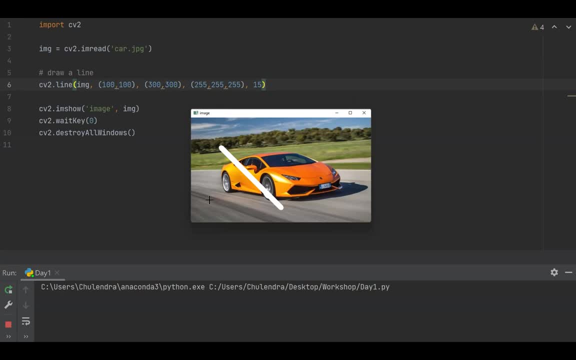 100 comma 100 coordinate. 200 comma 300 coordinate, here 300 comma 300 coordinate. So here is the line Because the pattern 255, 255,, 255,, 255,, 255,, 255, 255.. 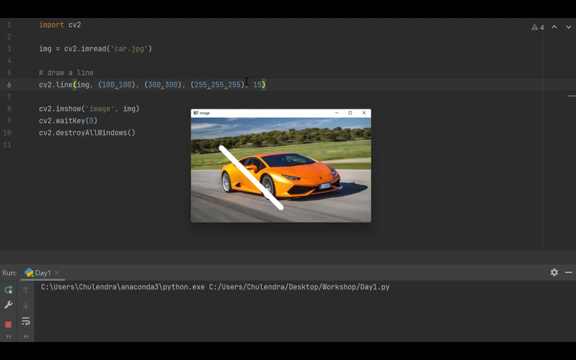 Now this line is the line what? what is it? so I am going to use white color. width will be 5. 5 is the width. see if I draw width. I can do it. add width. width to sorry. thickness to line. thickness to line. 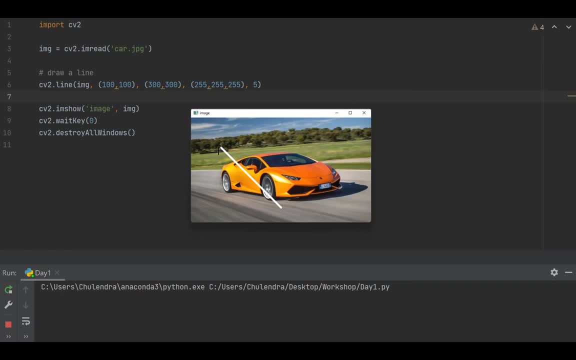 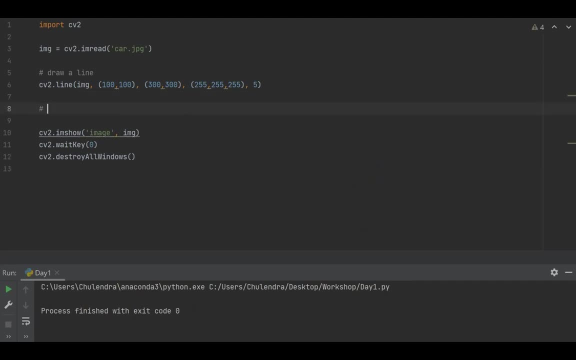 see I am going to plot line on image. see, draw a line. see how to draw rectangle. For that we have to use cv2.rectangle. Again, image On which are we going to plot, right? So image. Then we have to give a coordinate of 50,50 to the rectangle. 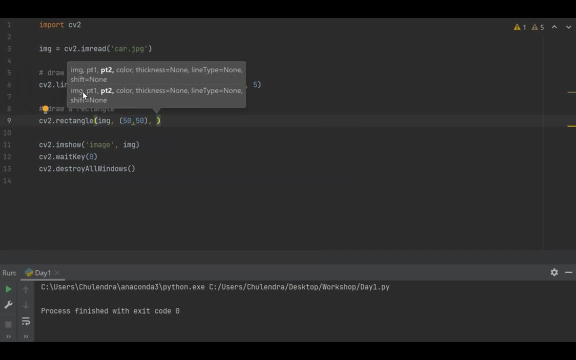 Diagonally. I will show you that. After that I will give a second coordinate. What is the part? What is the part? I will use a blue color: BGR, BGR Blue, full blue. Others are 0.. 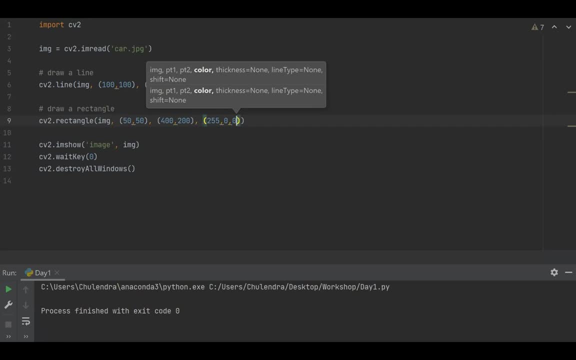 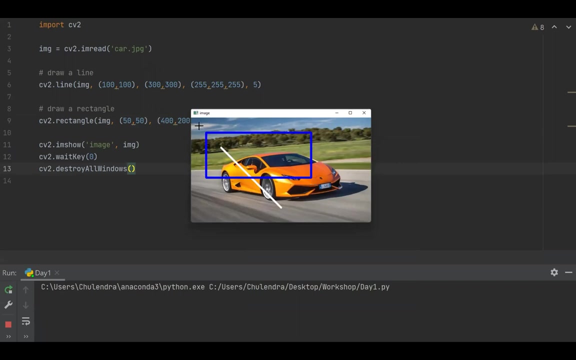 Green are 0,, Red are 0.. Blue, fully blue, BGR. Then the thickness: I will put 5.. So let's run this. So here is a rectangle. So these are the coordinates that I selected: 100, 100.. This one is 100, 100, 100 by 100. 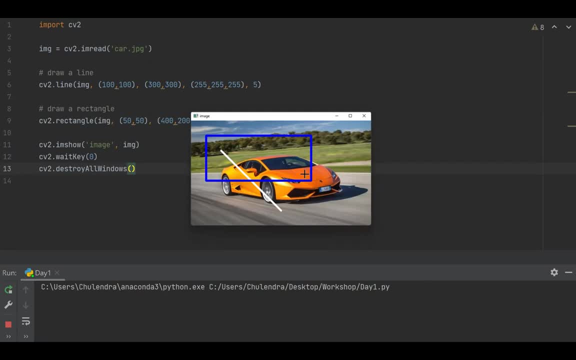 This point is 300 by 300.. You can use any color you want. If I put here 170.. Let's see what the color is. This color I put 150.. This color I'll keep blue right. So that's how you are plotting a rectangle on an image. 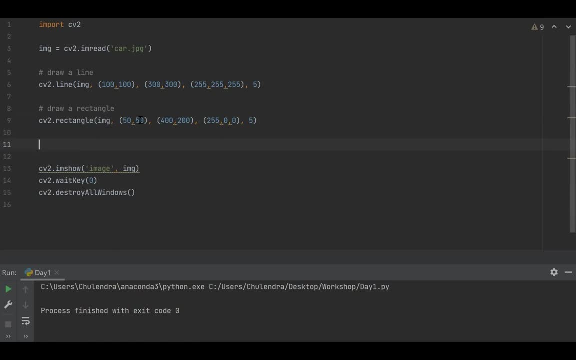 Next, let's see how to plot a polygon. Sorry, Before that I have some interesting thing. If I enter minus one as thickness, let's see what happens. As you can see, it is a field rectangle, right Field rectangle. 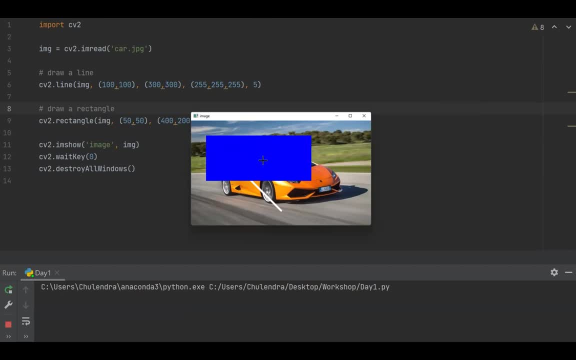 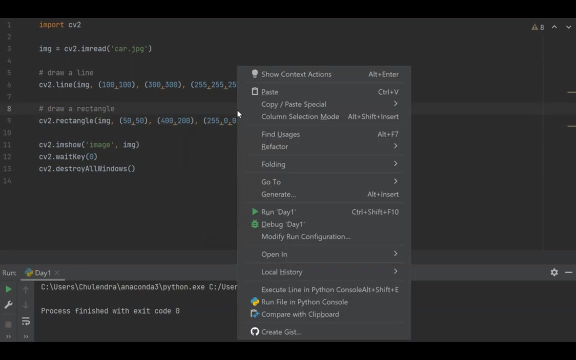 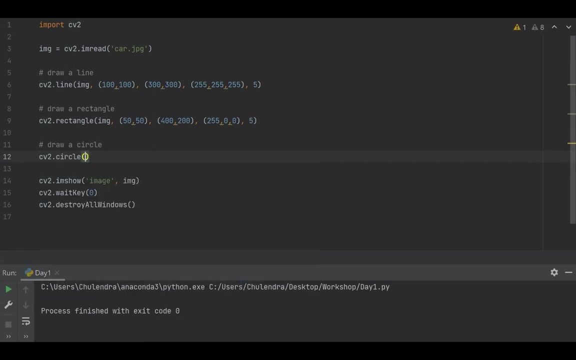 Field rectangle Minus thickness is minus one. That's, that's interesting, OK, so then Let's draw. OK For that cv2.circle. img. I'll put another one here. img. I'll put a center coordinate. 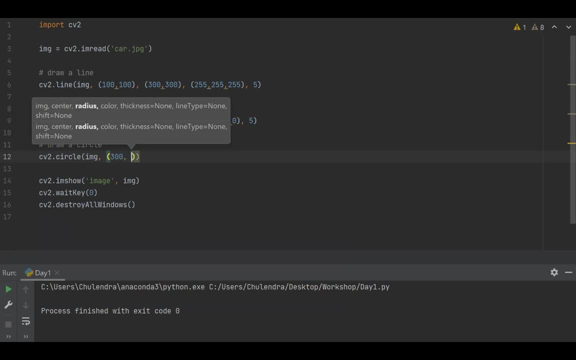 For the circle I'll put a center. For the center I'll put cv1, cv2, cv3.. For the circle I'll put a radius 30 degrees. This is the radius of the circle. I'll put 0.. 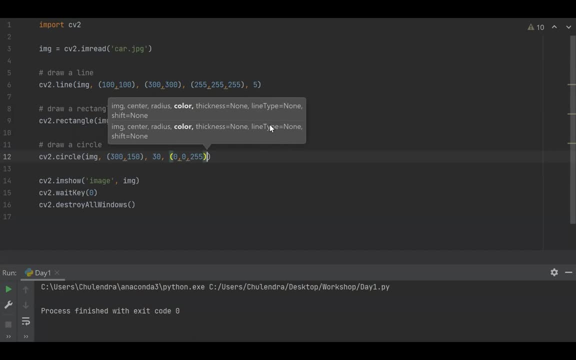 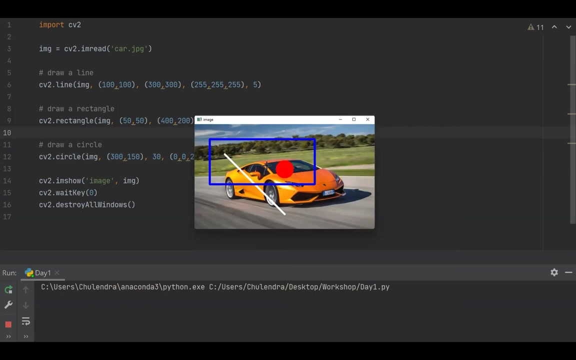 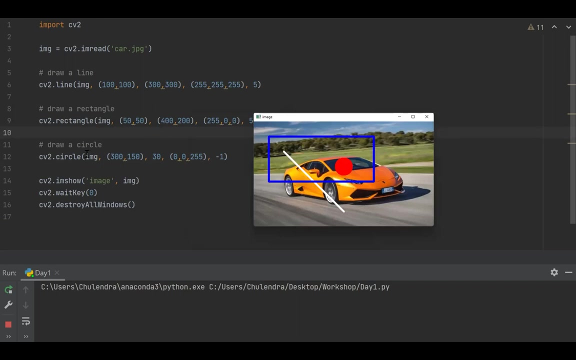 For the circle, I'll put… bgr. I'll put a red réfractor, I'll make bgr 0 in red. Look at that, It's a fill circle. so the center of the circle. so this parameter- so this is the first parameter- is the one. 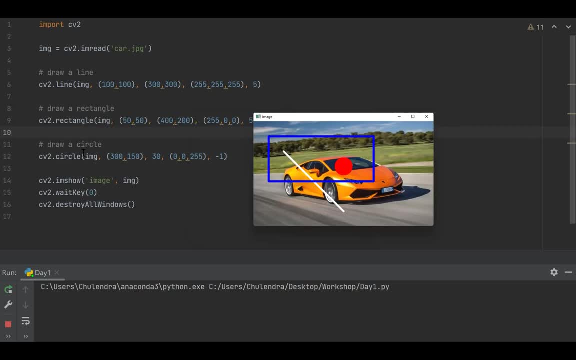 the, the, the image we are going to plot on right then, the next parameter is the center of the circle and the next parameter is the radius of the circle, and this is the color of the circle. and this is the thickness of the circle. thickness minus one means fully. 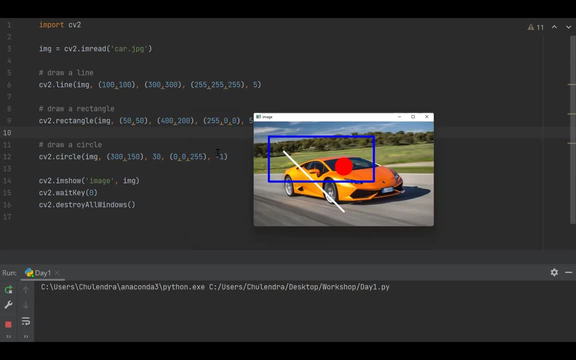 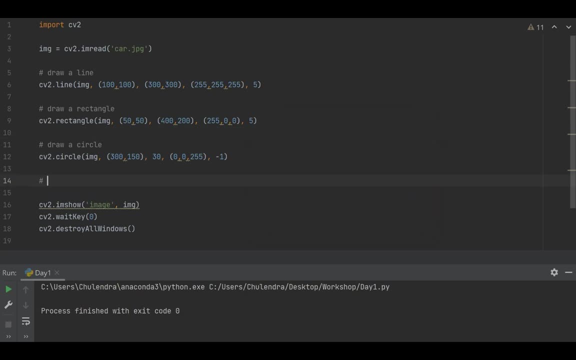 uh, fill, fill, filling, fill, uh, fill circle, right, so that's how we are drawing a circle on image. uh, let's see, let's see how to draw a polygon for this. i have to import numpy, sorry, numpy- library, import numpy as np. right, we have to, we have to uh. 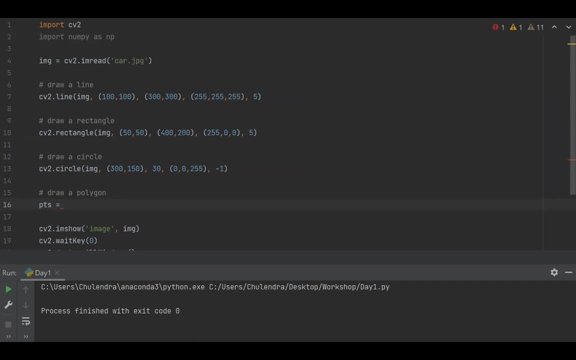 determine the points that we are going to draw, right. uh, that we are going to draw the polygon, right. so what are the points? these points, i will copy and paste: numpy array, so it's an array of coordinates. right, those are our controls. right, just keep, keep it mine. 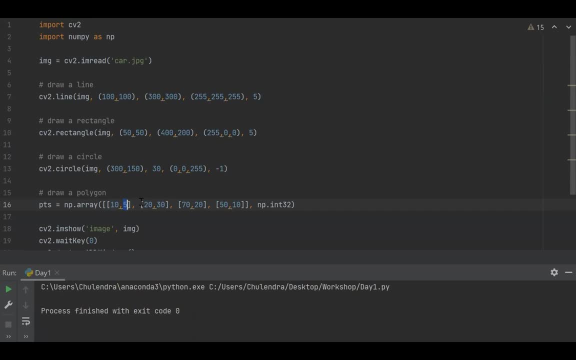 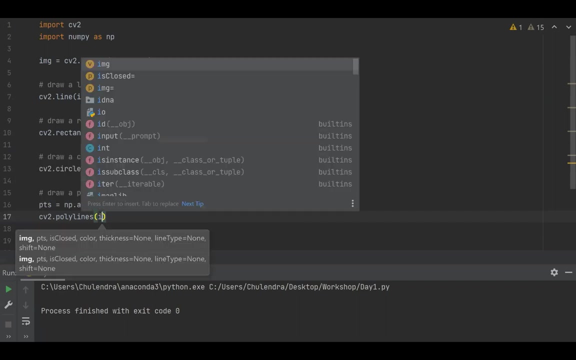 keep it in mind that this, this is height, this is sweet height, sorry, with height, with comma height, with comma height, right with comma height. that's how you was uh, define what? uh, Okay, Then next slide C2, both polylines, Polylines, Same as before. image. Then what? 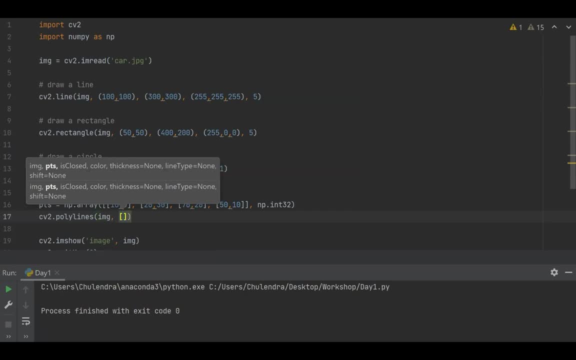 are the points Inside the bracket. Inside this bracket we have to put the points. Points Then isCross. IsCross means whether this polygon is crossed or not. Right, I'll put through Through. means ending starting point and ending point of this polygon is connected. Right. 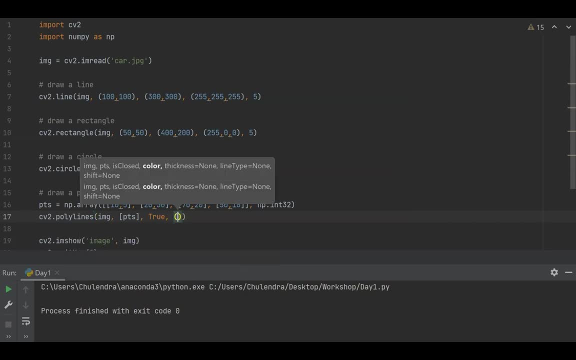 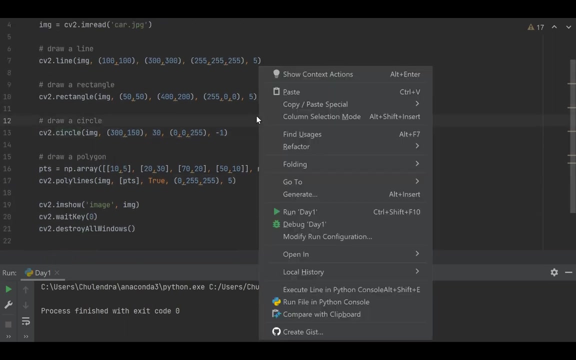 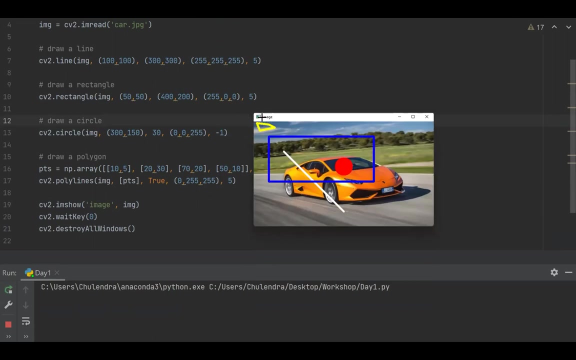 Then the color 0, 255.. 255 is my color And the thickness, This is the size. I drew it as 5.. So if I run this, So this is the polygon I drew, Drew, Right? Hmm? 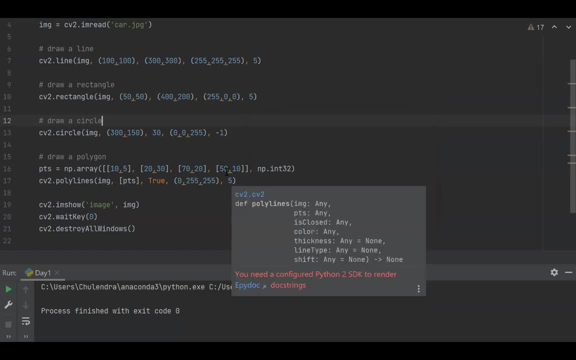 But here you can't enter minus 1 for the thickness. It will give you an error, Right? So here is this error. So I don't know how to draw a fill polygon in OpenCV. Probably there should be a way for that. 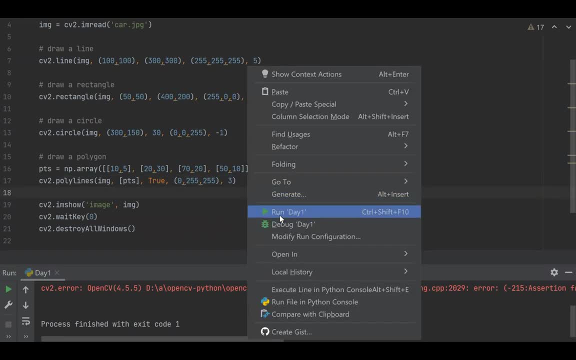 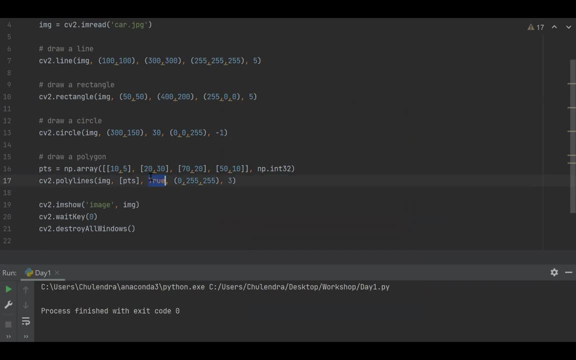 Hmm, Hmm, Hmm. Okay, This is how you draw a polygon. So if this is force, the starting point and ending point needs not corrected, Right? So if we run this, So this is starting point and ending point needs not corrected. 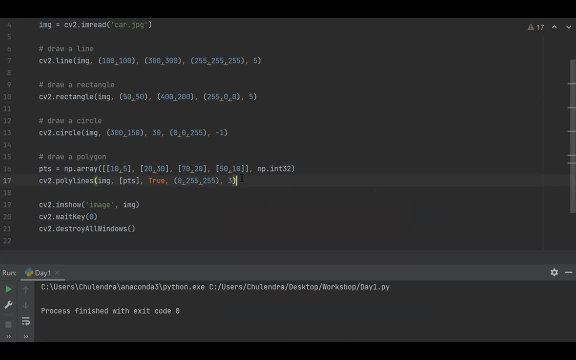 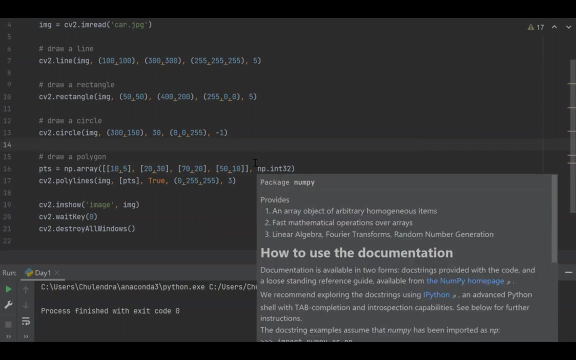 Okay, So, So I put it. That's true. then question is us: what is npin32 in 32 bits? yeah, but you can use uint8 or something. wait, oh, uint8 doesn't work. right, in 32. is 32 in 32 mean 32-bit integer? right, the data type of this array? right, that's, that's how we. 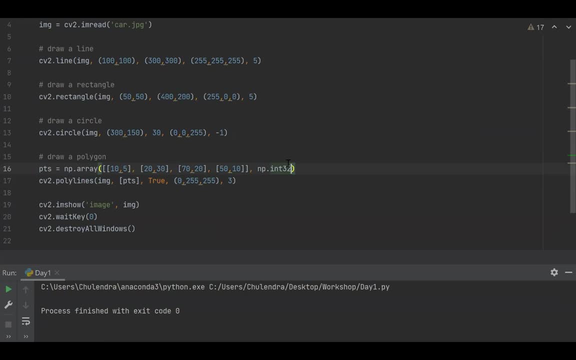 do it. so this is the data type of this array. if we need this one, there should be a right. no, it's working. it's working. yeah, it is optional, but in uint8 doesn't work. right now, uint8 can't be used. yeah, this is not not the color. well, it's not in 32 is. 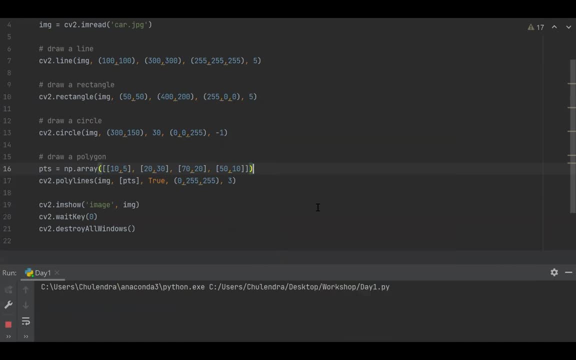 but we can omit this one. it works. so this is a data type of this umpire, right? okay then let's let's see how to write on image. writing text. right, writing text. let's see font. sorry, give me to that. put text. what is the image that we are going to write on? 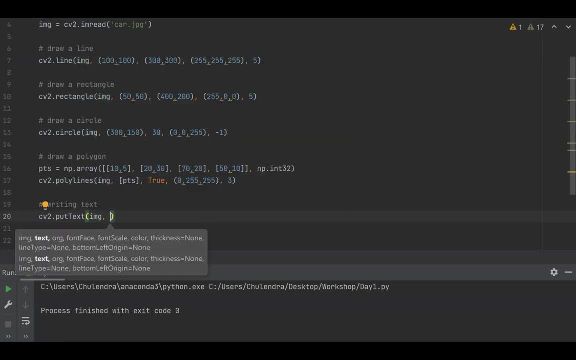 it is image. then next parameter is the text that we are going to write on. i will put workshop next, the next, the next, the, our g miss uh the point where we are writing, the place we are placed, where we are writing the text. right, i'm writing on. 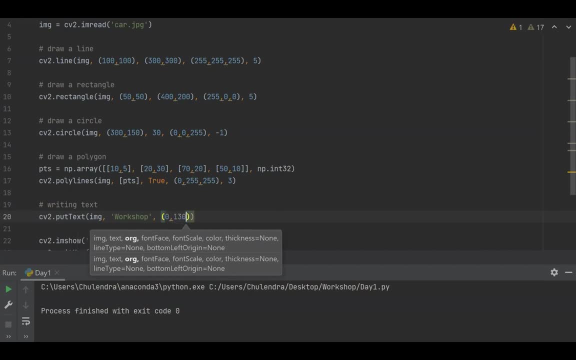 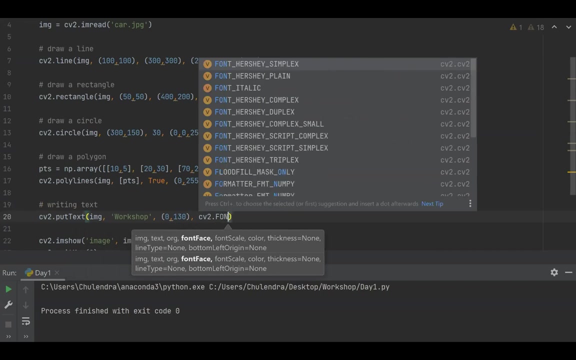 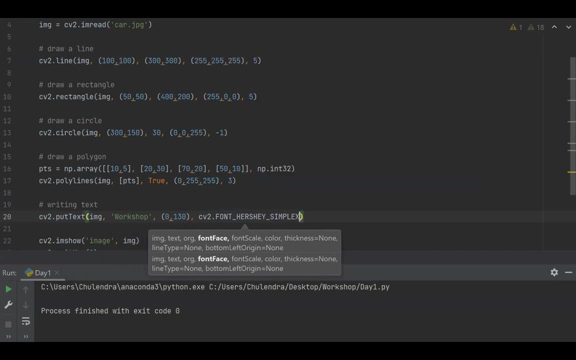 this is the top result, 3 130, and the font font face me. font face me phone font that I'm going to use is c2.. There are couple of font. I'll select font Hershey Simplex, Simplex, Hershey Simplex. 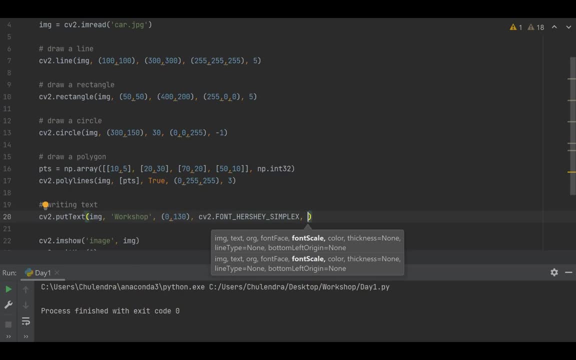 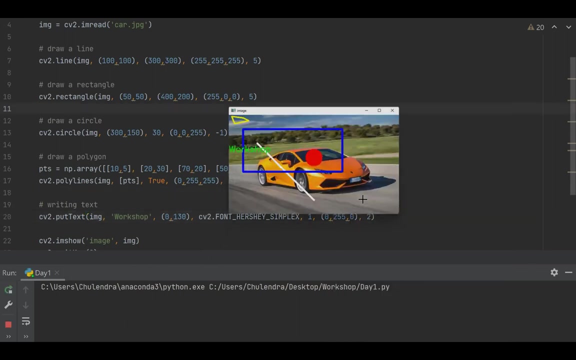 Font scale means font size, I'll put 1.. And the color of the font. I'll say green BGR. Thickness is 2.. Thickness of the text is 2.. Let's run this So it is written in green. 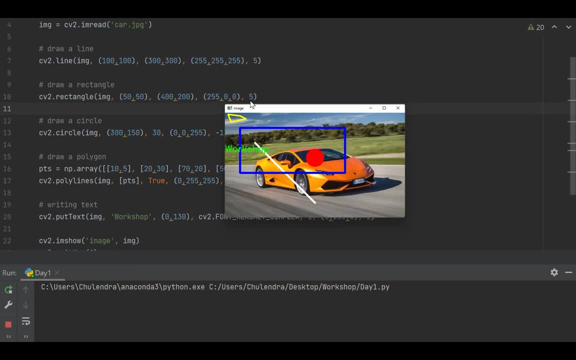 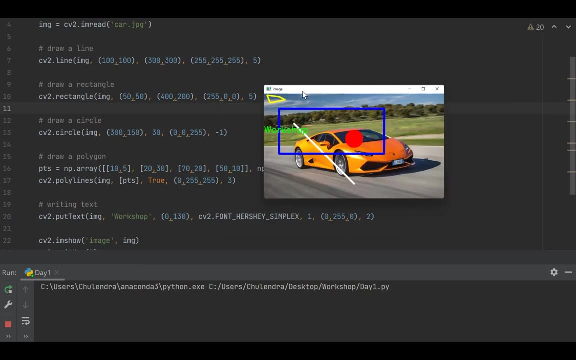 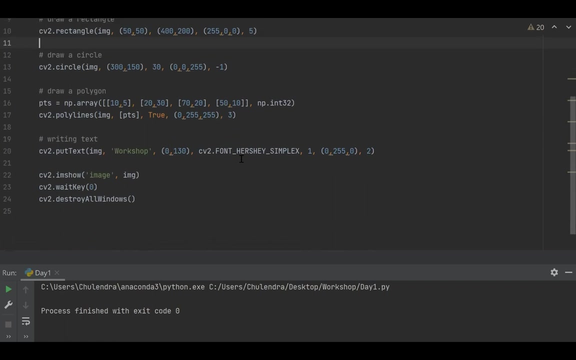 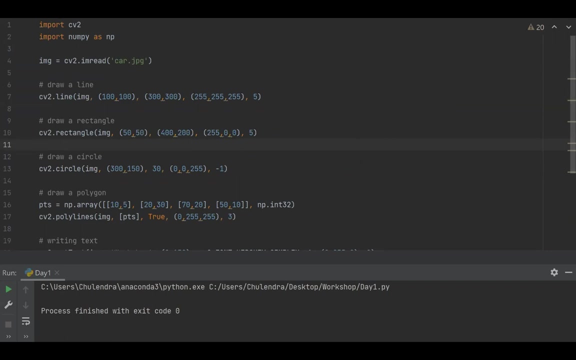 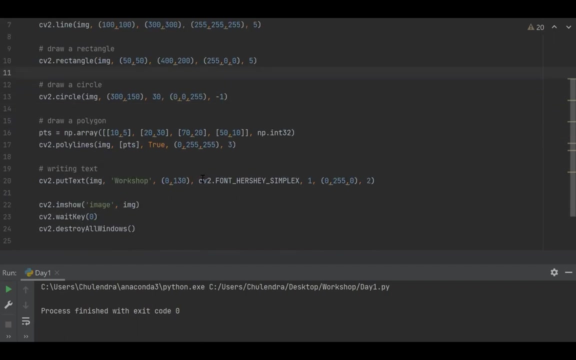 So this is how you are writing a text on an image. Those are the things that I needed to cover in this section. If you have any questions, please feel free to ask. Thank you, Let's talk about image addition. If you don't have any questions, I'll move on to the next section. 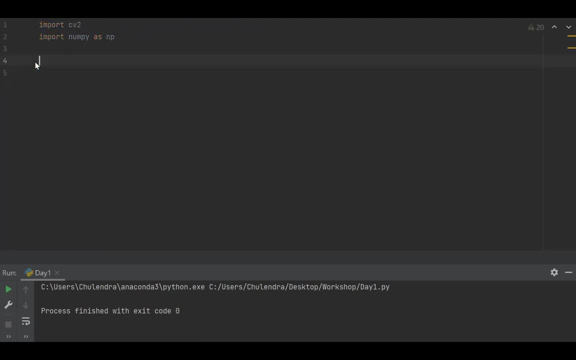 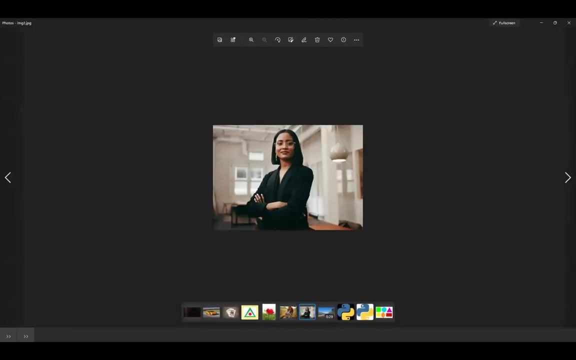 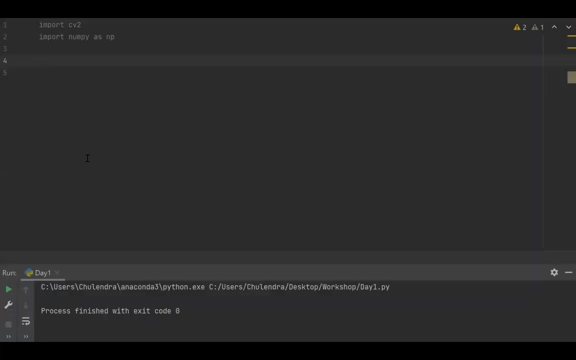 There are two images, Image 1 and image 2.. These two images, These are in same size. right, We need images in same size for this section. I'll first read these images As image 1 and image 2, like this: 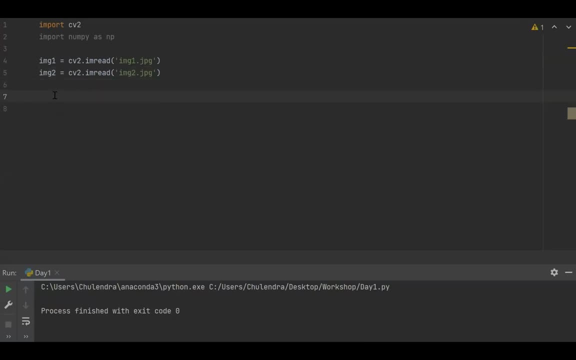 Then I'll perform row addition. right, So this is about image addition. Okay, So you don't need Lampy array, Lampy library. First addition: I'm performing row addition. Row addition means nothing but image 1 plus image 2.. 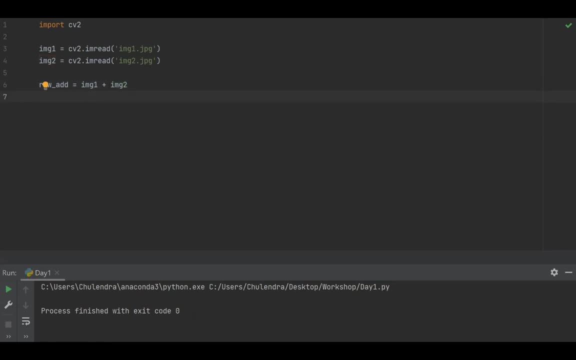 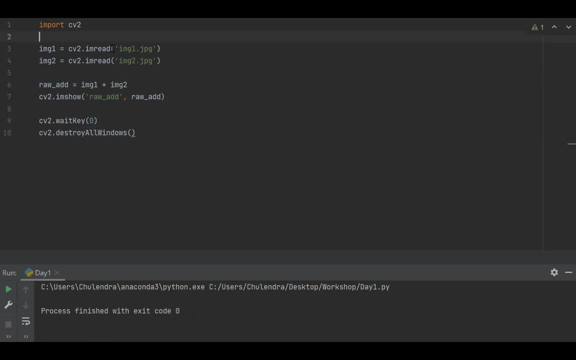 Faster. Yeah, let's run this. This is the result. right? Kind of ugly, right? This is a row addition. This is a row addition, That is. that means it is nothing, but simply added two arrays. There's another addition in OpenC. 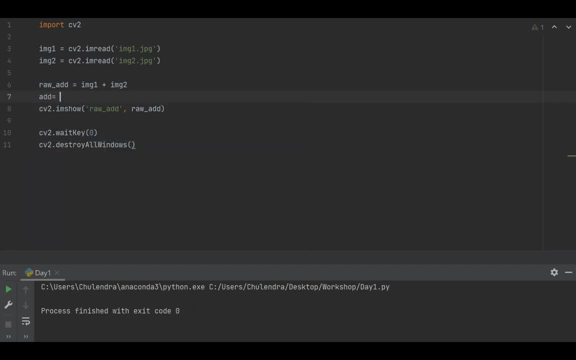 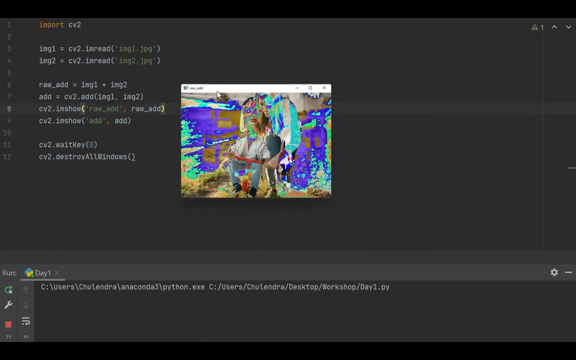 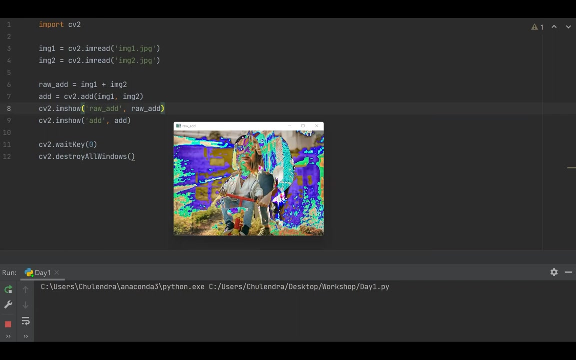 CV2add. I'll say add CV2.add. image 1.. Lift up from original. That's everything right. comma image 2. I, So let's initialize this. This is the result I got. So observe the difference between these two. 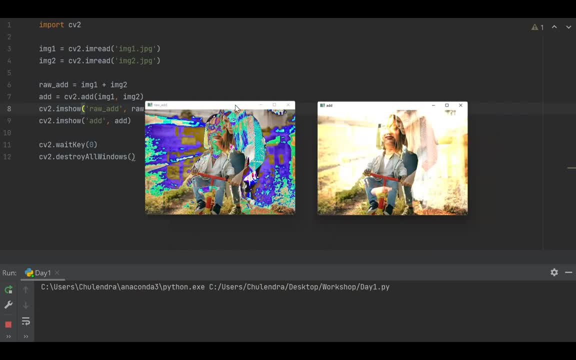 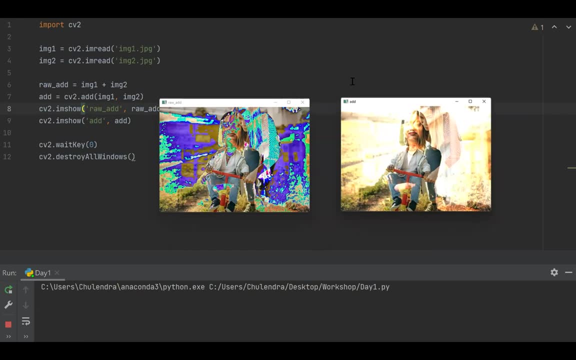 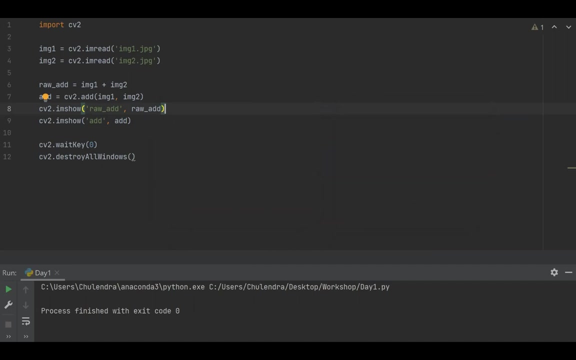 This is row addition. This is the addition given in scene2.. Why there is difference? I will tell you about this. Why is that? I will comment this out. Let's say I have a pixel. Pixel value is xnp, It is unit. 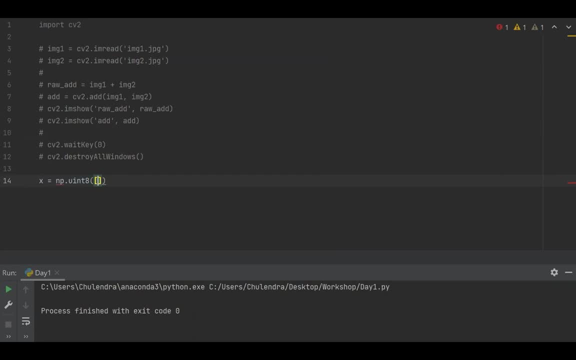 unit format. It is 250, 250. Then I need umpy here. Let's take another pixel value. Why, Since it is a pixel value, I chose uint8.. uint8 means the values of values, of values in the array, So it is. 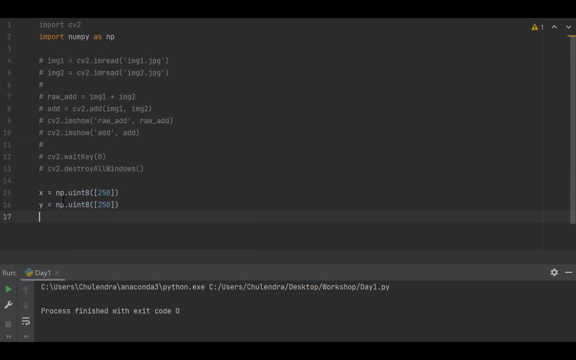 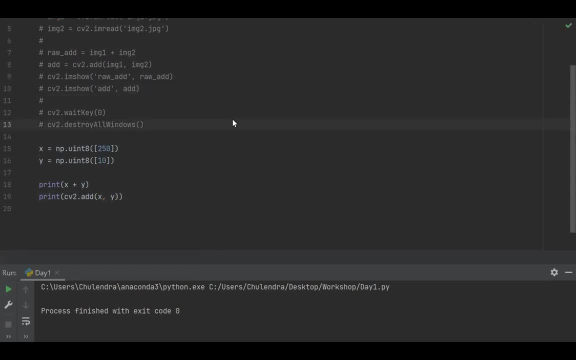 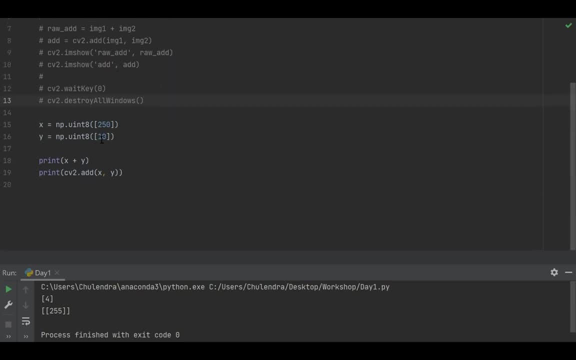 Then you can see the reason for that. I took two points: x and y. It has a pixel value of 0 to 2.5.. I took that with uinted, So this is the row addition that we added. This is the row addition of x plus y. 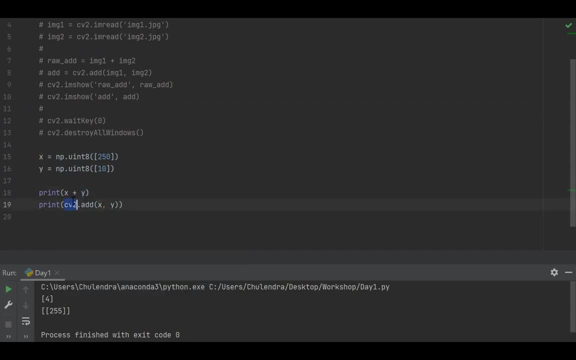 This is the addition of normal m. This is the addition in the library. If you look at the row addition 255 times 10 is 30.. 30. But we have 4 answers. How will 4 come? 4 will come. 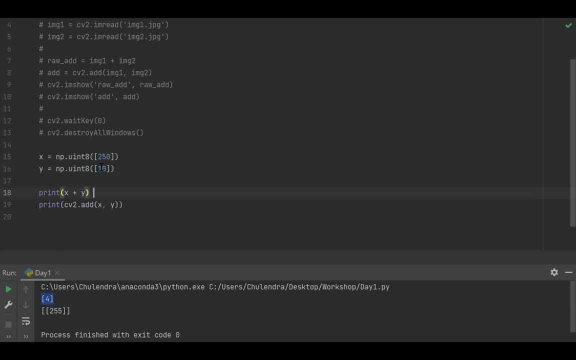 The number that can be kept inside this is more than 2,500.. Then it is 230. That's why 230 cannot be kept. It can be kept more than 2,500. Because this value is still there. Before 2,500, it was 4.. 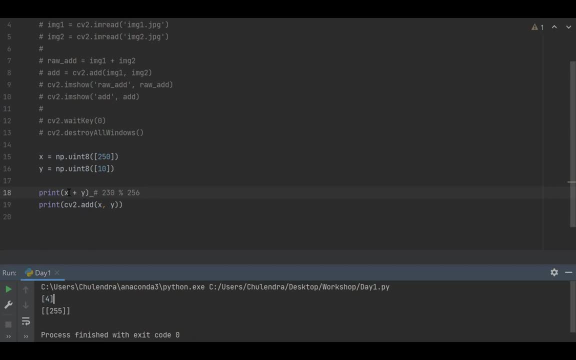 4 is 4.. So if you add this, 4 is still there. That's why 4.. Because this can be kept more than 2,500.. And this addition can be kept more than 2,500.. But it's not 230.. 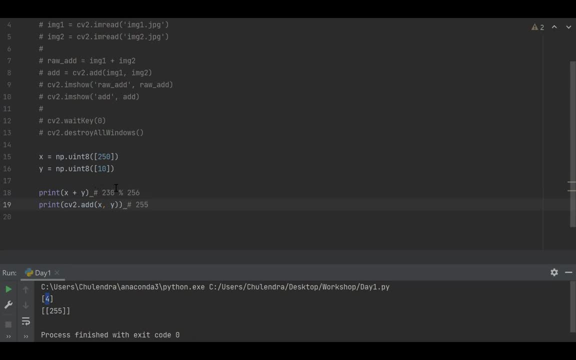 It's still 2,500.. So this is the difference between these two additions. So in the first way, so you know that the addition of 250 and 10 is 230.. 230 cannot be held inside the unitite array. 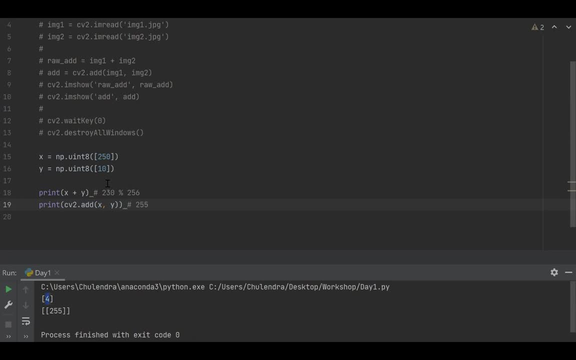 So it produces the result. It returns the result of the demand of the 230 divided by 256.. That's how this 4 came. So how this 255 came is in this cv2.addition method: x, y, 250 plus 10 is 230. 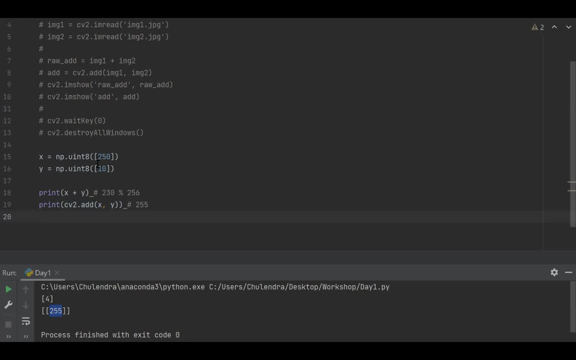 230 exceeds 256.. So 250, actually 255, right 0 to 255,. we can hold on to 0 to 255.. So the maximum value is 255.. So that's why it remains at 255.. 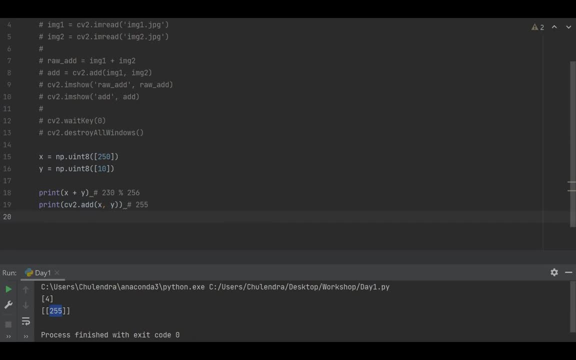 So we have a question: How did 230 value come 230, value come Sorry 230,? no, not 230, sorry 260. Sorry 260, right, 250 plus 10 is 260.. So 260 can't be held in unitite array. 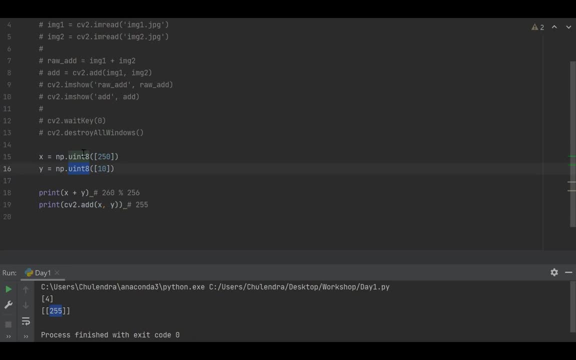 So I chose unitite array because image read by OpenCV is in unitite array. So that's why I chose unitite here. So if I use unitite, if I read an image from the OpenCV, I can make it in unitite array. 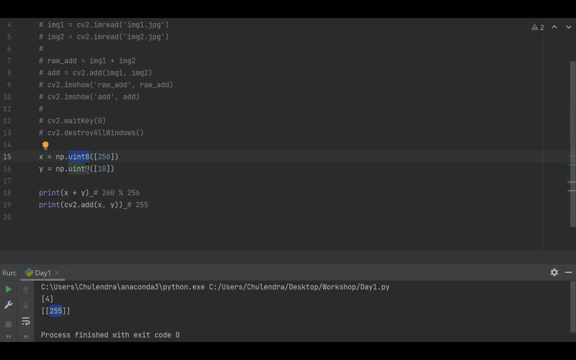 Unitite is the data type of an array, So unitite is a value of array. The value of the value of the array can be 0 to 255 or more, So the maximum value is 255.. So this is the normal addition. 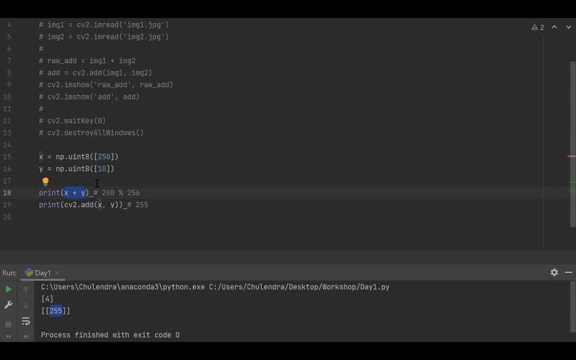 This is the remainder. 255 exceeds 255.. 255 exceeds 266.. 266 exceeds 255.. So 255 is the remainder. So the answer is 255 modulo 266.. So that is 4.. So the answer is 4.. 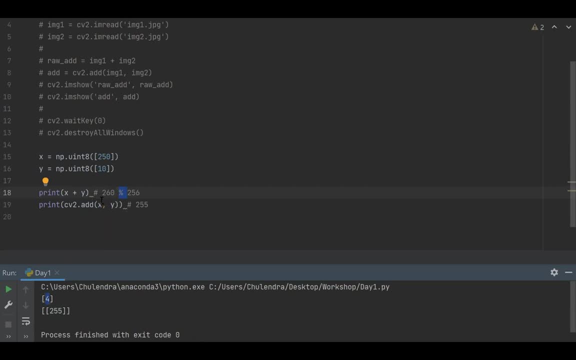 Let's say cv2.add will be added. So we have added cv2.add to add. so this is 266.. Now we cannot say 266, but let's say 250.. So you have to give the same as 250.. 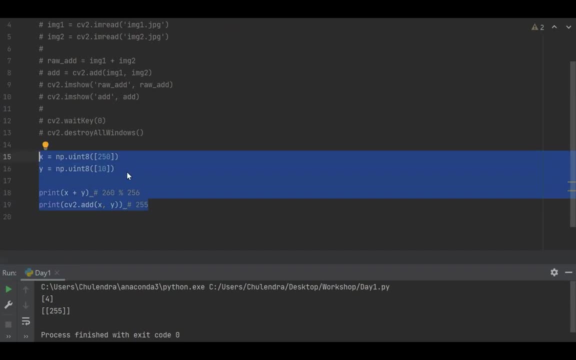 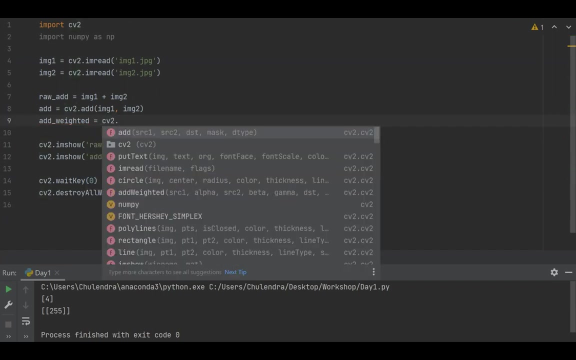 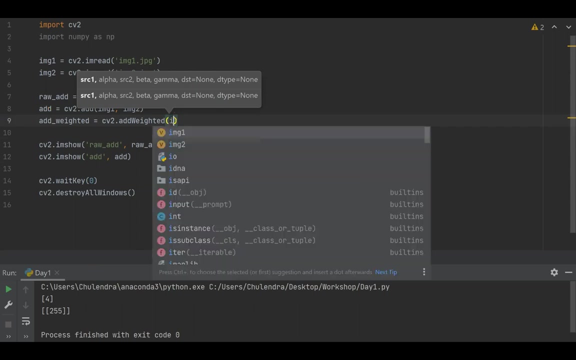 Here also, 255 is entered, So that is the remainder. So that is the remainder. Next, we can, I'm going to perform it. so we didn't wait. I'll call it as a trader and do the same thing to do and we did. source is image one. 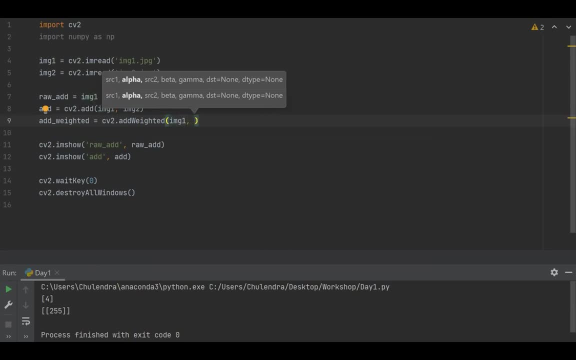 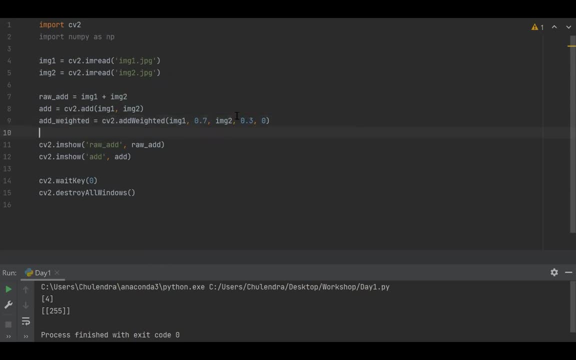 plus Point three, gamma, me point three, point three plus mesh, to write: this is this: is this is faded Right. So we are going. we are considering weight tested in this case. So these are the rates associated with each image. So point seven correspond to one. point three is correspond to mesh to 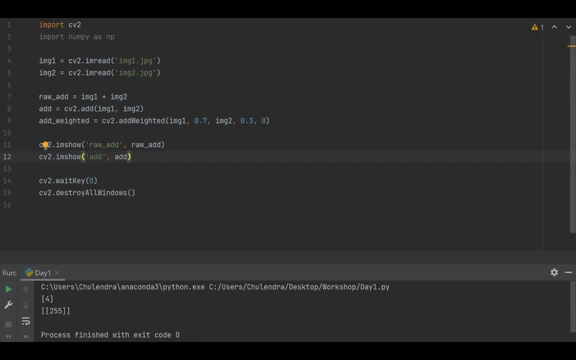 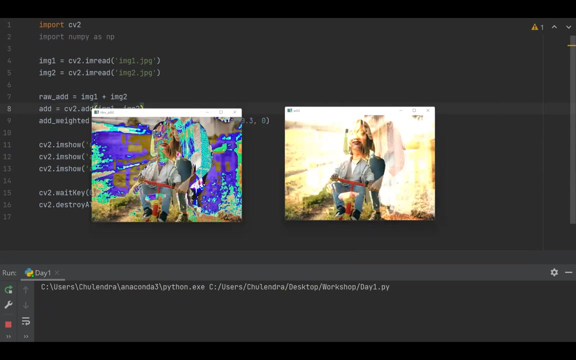 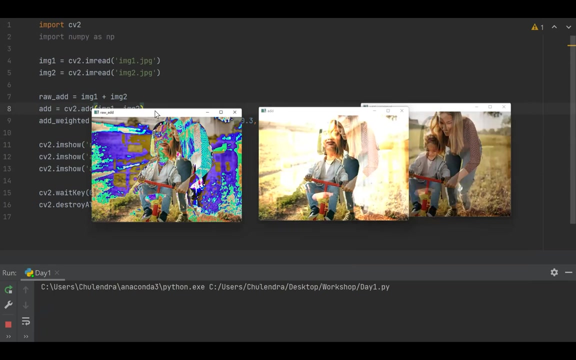 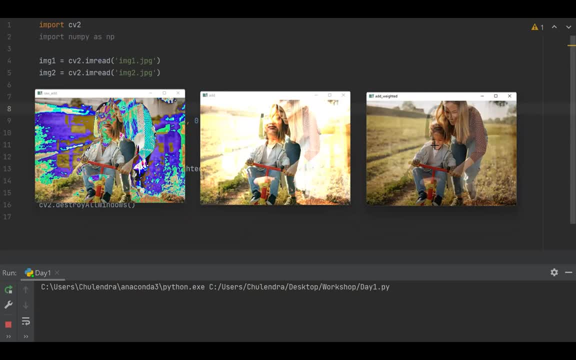 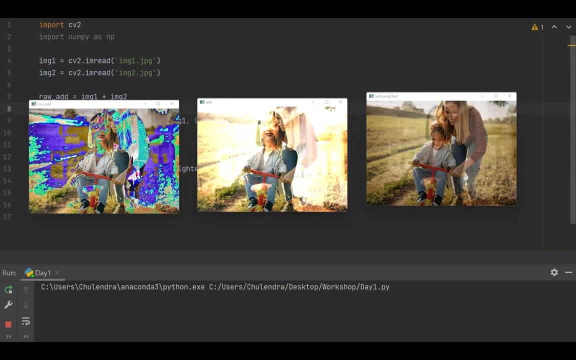 This one is The shadow of this second second Right, So you can play with this Right. Okay, So, Okay, So, So, Okay, So That's about, That's about, Okay, So, So. that's about the addition. 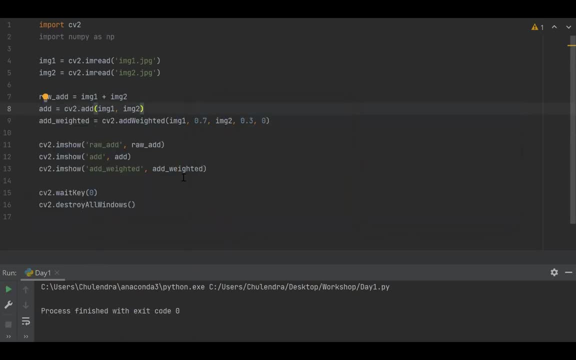 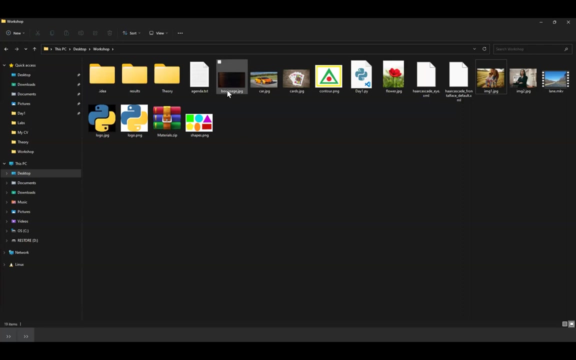 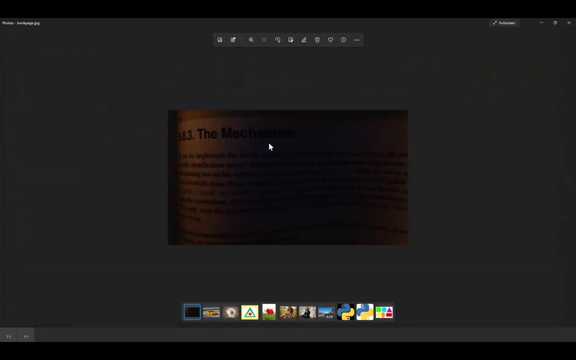 That's about. So, Okay, Okay, Okay, make addition. Let's talk about thresholding, right? What is in my thresholding? For that, I'm going to use this bookpagejpg image. So it is very dark image, right? Dark image. 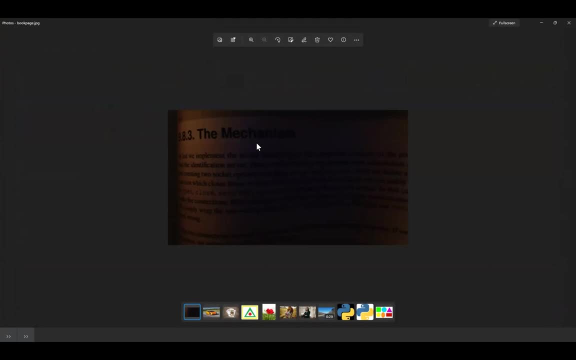 There is a variable. So this is very interesting. right, We can't read this one right, But using way of processing, we can make it clear. right, So we can't see. actually, Let's see how to read this one right. Using thresholding, we can do this Okay. 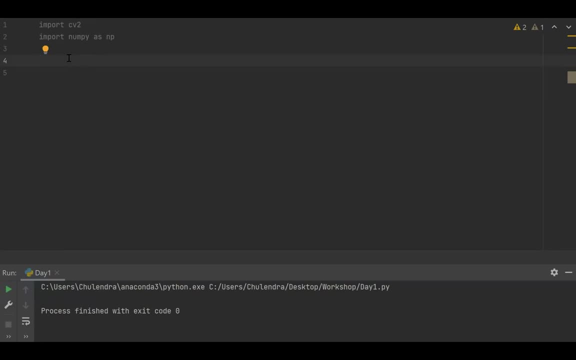 So I'm going to read the image and the image name, the path for the image. I have book pagejpg and let's have the gray version of it. gray we need before: before performing uh thresholding, we have to uh convert it into a scale: right way, scale. 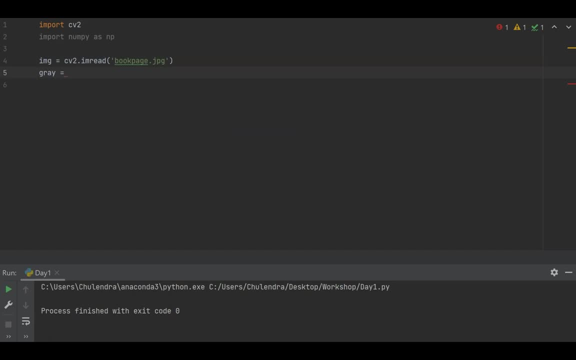 can use color thresholding also, but it is not useful so. so so we are using black and white pv, right? so scene 2: dot ct color image that we are going to change. the color space in the code code is nothing, but, as as i told before, 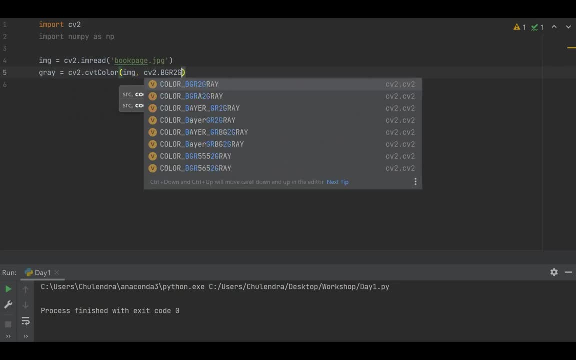 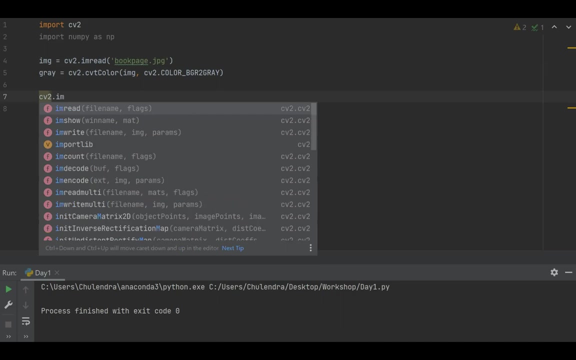 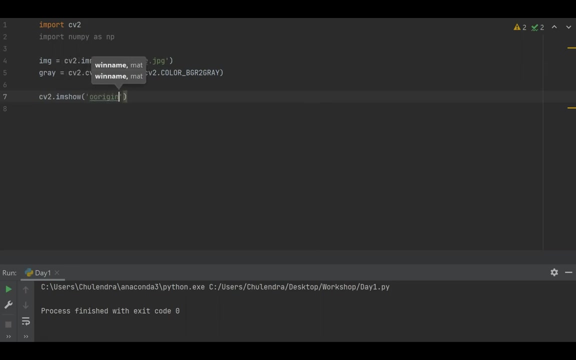 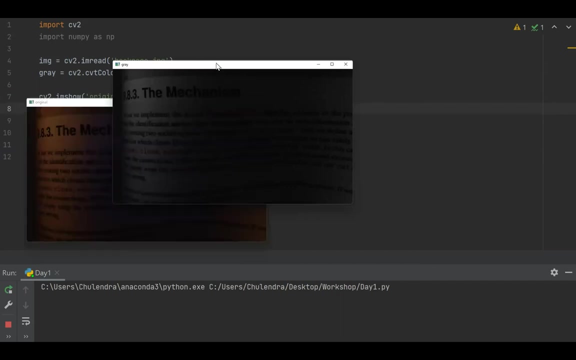 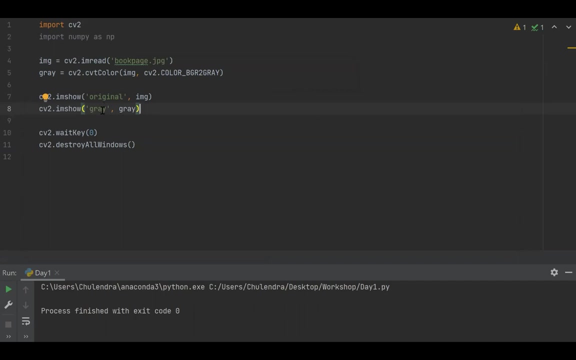 vgr, right. so sting to the. let's visualize this original image and i'm going to be pasting: uh, gray ocean right, more you, you, you. so this uh should be key. yes, yes, yes, yeah, this this output two we can't reach, but this is the last performance i showed you right. 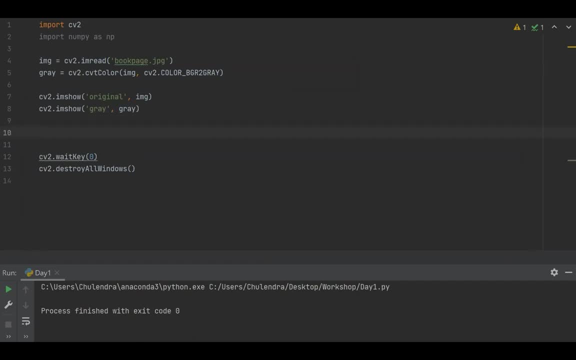 now let's come on personal special. so equal cv2 dot threshold. you have to pass the gray image here, gray, and the value value. i'm going to put this 10. so since this is a darker image, dark image. so we have to use a low value for the. 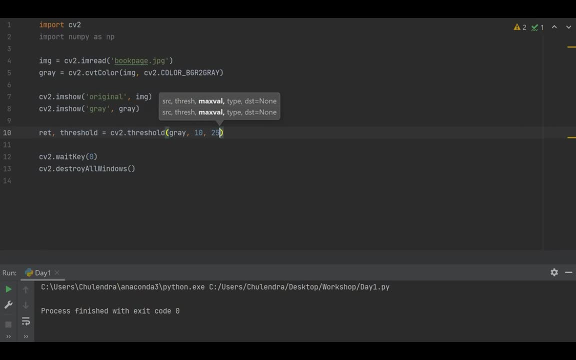 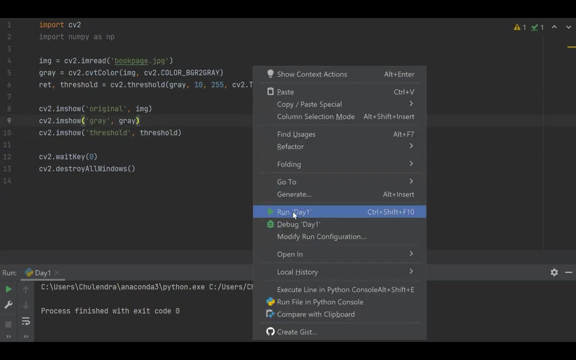 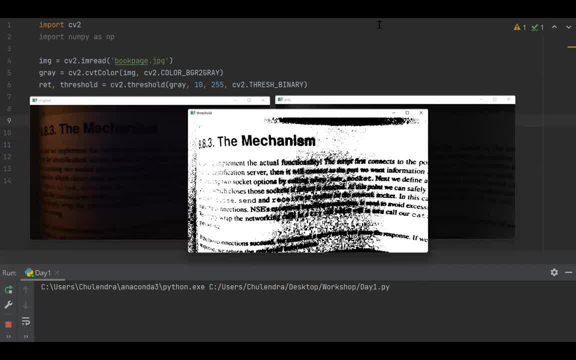 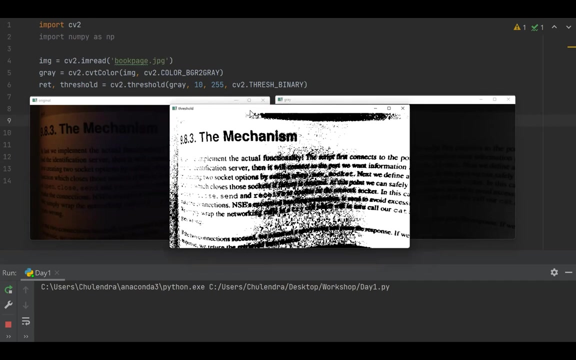 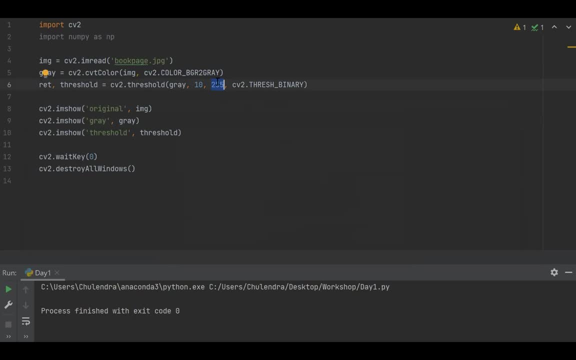 2.25 is the maximum value. this is the upper bound. the lower bound is 0. what is the value of this? it is like this. I will write it in the comment. there is a mass scale. f is the image, the pixel of the image. 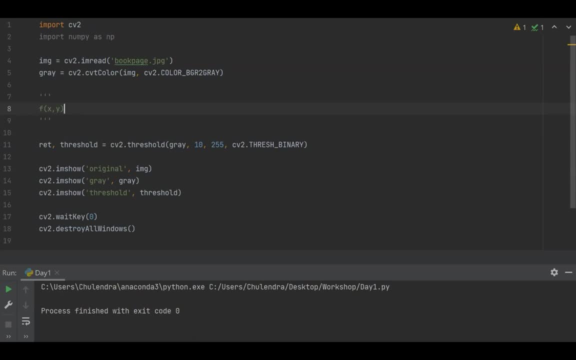 f is the image, xy are the coordinates. if the pixel value is the image. if the pixel value is the image, I will write f. f is the mass, the number of pixels. ok, f is greater than 10. if 10 is greater than 10, 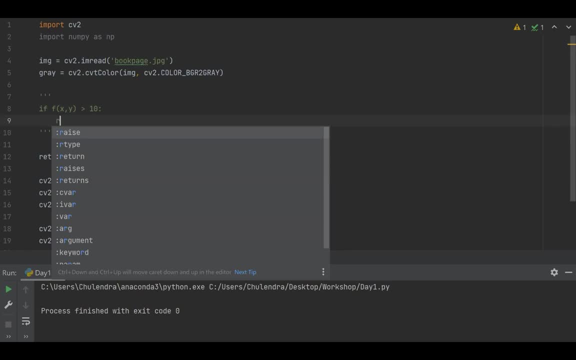 return. if 10 is greater than 10: return ok. f is greater than 5. f is greater than 6: return the error is 255, else else is 0. this is what happening. underline the threshold. so if a particular point of the image, suppose it is f, it is greater than 10. 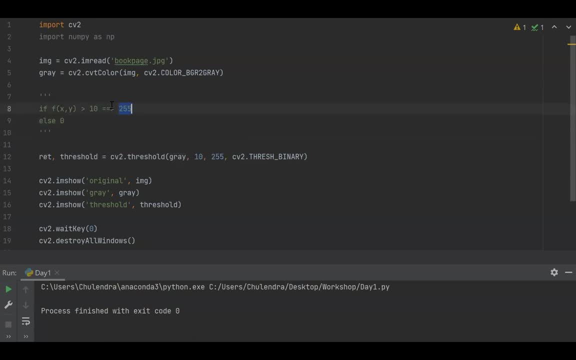 the resultant value will be 255. otherwise it should be zero. so this is happening. this is what happens in simple basic thresholding. there are some other thresholding as well. we will talk them in later in next right. so this is what happen in simple thresholding. 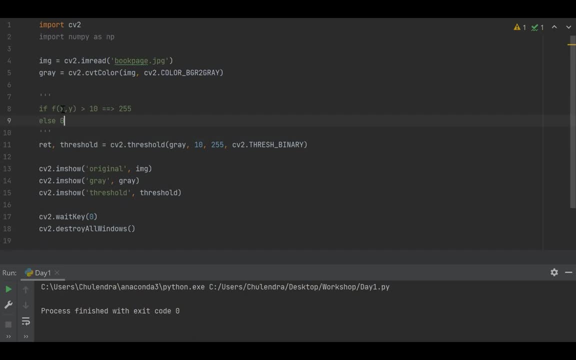 consider f as the pixel value if it is greater than 10- 10 is the one I am selecting here- which is greater than 10. return 255. otherwise return zero right. so so this is a binary right, zero id. it can be either zero or 255. 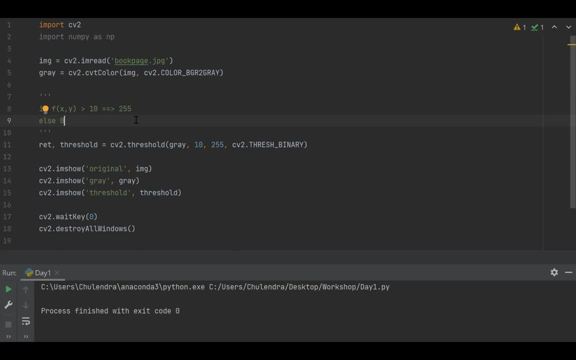 so, so, so, so, so, so. so, if you have any doubt regarding this statement, then in this call, please ask: right, so, what happened? is this one? right, so i can show you. there is an interesting we can, we can, so we can see how, how, the, how this binary made this change according to the value given into this position, right, so? 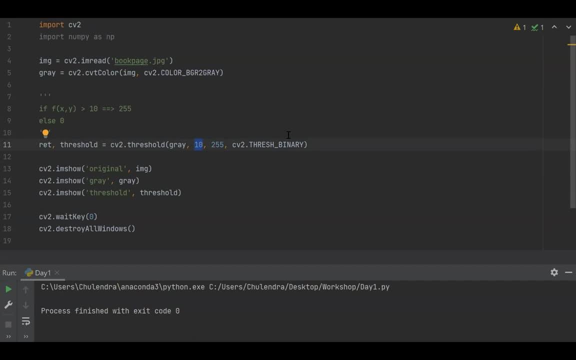 we can do it like this: we need to create a track bar for that, right? so i'm going to show you a demo, right uh, of what is happening underlying here, right? so track bar is nothing but this slider, slider, slider. so you have a volume broker in your, in your laptop, in your, in the 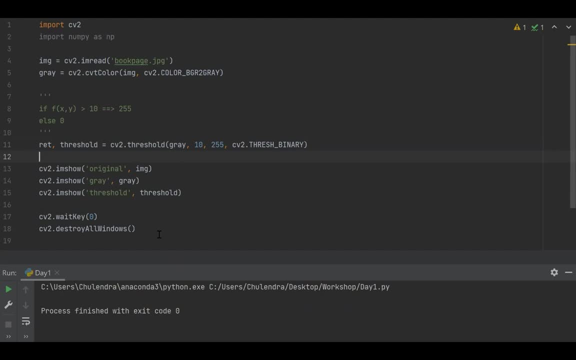 sorry, i mean the volume slider. there is a slider to change the volume in software, right, so so you can use such kind of implementation for this. for that we have to use the track bar, track bus, right, track bus. so let's see how to do it, uh. 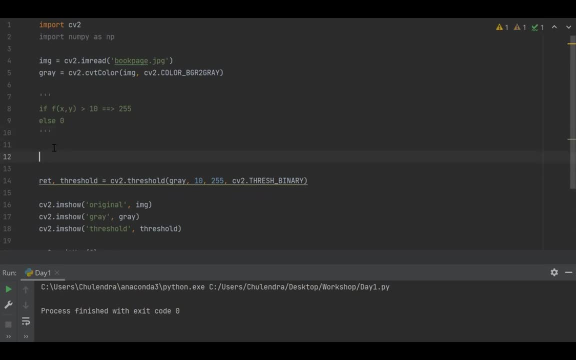 for this i'm going to. here we get a name window right. see, we do the name window name window. i'll call it as time bus. this is a window right with that name title title, right. so inside this tag bus window i have to create uh tag bar, tag t two dot. create thermal click tag bar. or here you have to specify the window. 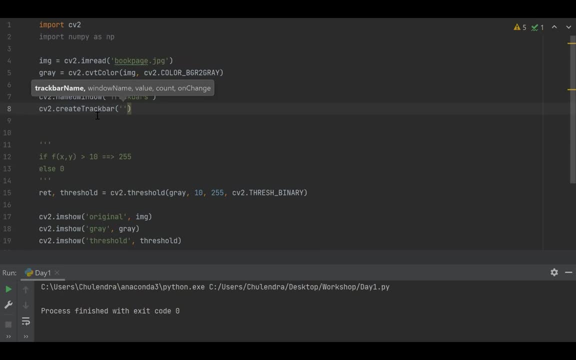 window. so we tag bar name, right. tag bar name is uh, drag one, but tag bar name ad is a little tag bar name I will show. I will select that to show Then Window name. Window name is tag box. We have what we have. 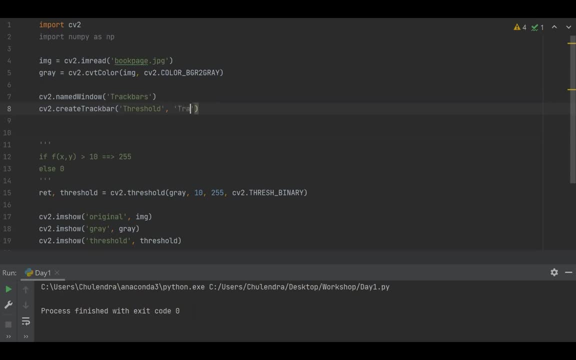 here: Tag box, Tag box, Tag box. Then Then what is the parameter? Then the default value. Right, Default value. I will choose as 0. Then the maximum value should be 255.. Right, This value can be. So I'm creating the tag bar for this value. 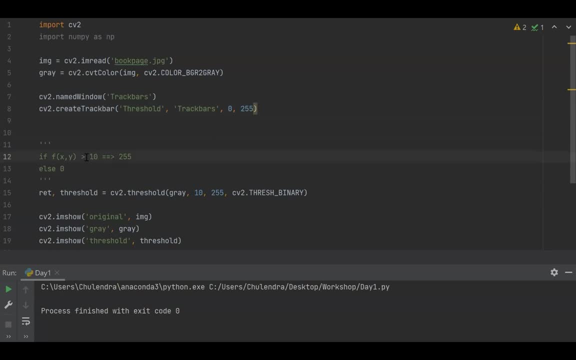 So it is. it lies from 0 to 255.. So that's why I put 255 here Then. Then we have to. So when? So when this event happened, when the changing of the size bar happened, there should be a function to call. 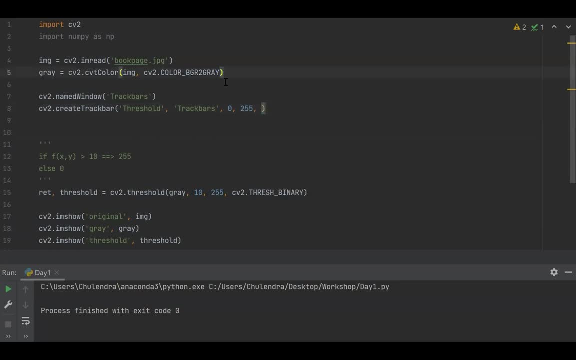 Right, This function should be written here. So I don't need any function for this. So I put empty function. I don't need any any function to happen. So I'll say as pass. So I'll say as pass, I'm creating this. 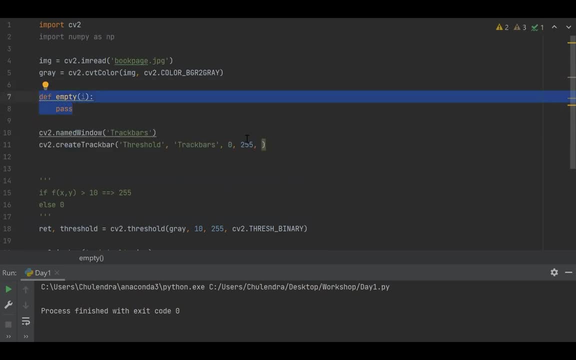 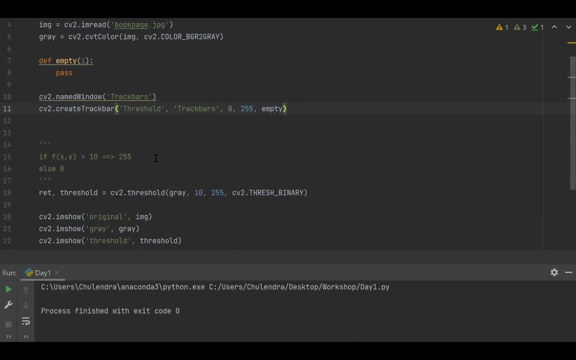 just a dummy, dummy function, So I'll call this function. when there is a change in tag box- So empty- You have to write the function name, Right, Okay? So that's how we create a tag bar. Then what I'm going to do is: 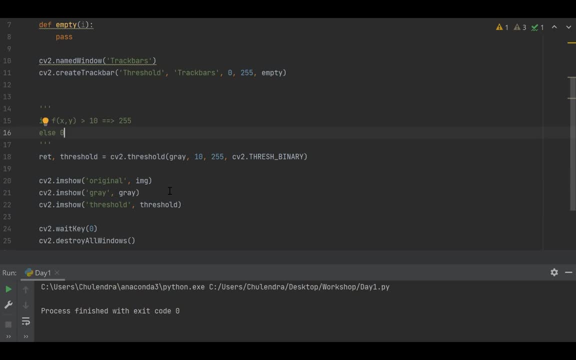 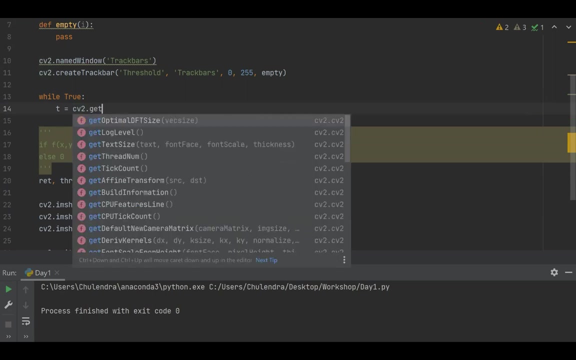 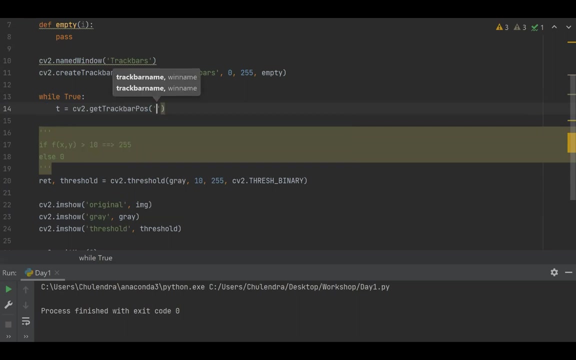 inside, inside the infinite loop, inside the infinite loop, while through, while through, inside the infinite loop, inside the infinite loop. I'll put as t as t, You will don't worry, My name is, my name is. the short name is tag bus, tag bus, right. so? 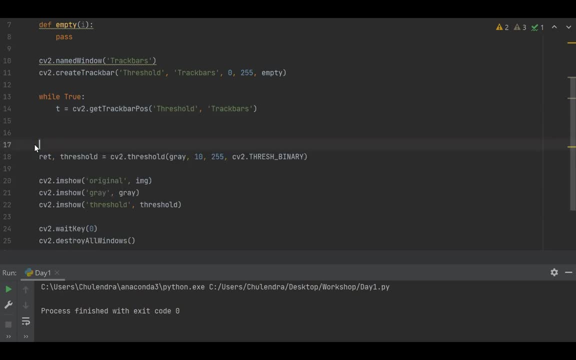 then I'm going to- I'm waiting- this one, I'm going to cut and paste this one here. so here I'm going to select: use t, here t, and I'm going to show the ensure. also this one will be. I have to change the instantaneous change. I have to use the instantaneous. 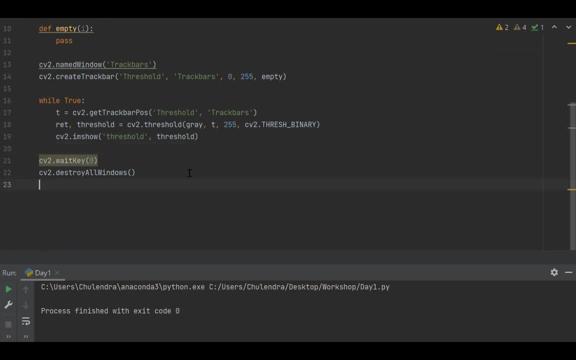 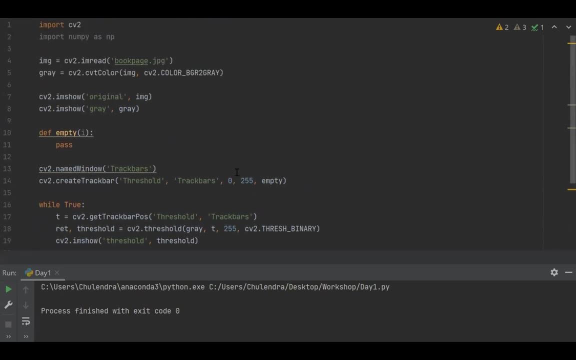 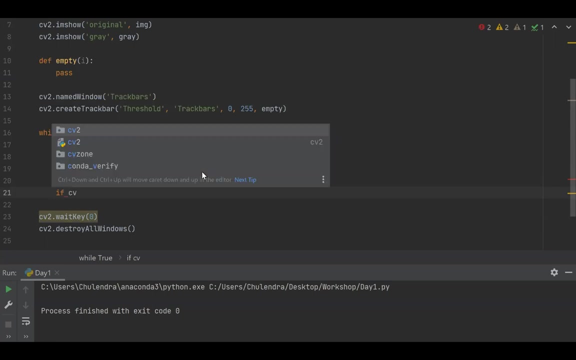 change of the units. right, okay, so let's start. hmm, before that I have to turn it, there's the condition, there should be a condition to turn over this group. so for that we do not wait. wait here, one right place, okay, so let's run this. so this is the result of the special 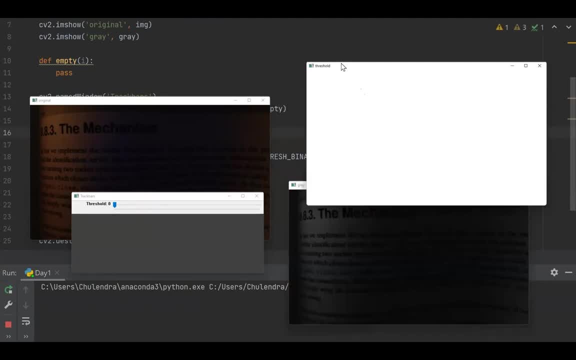 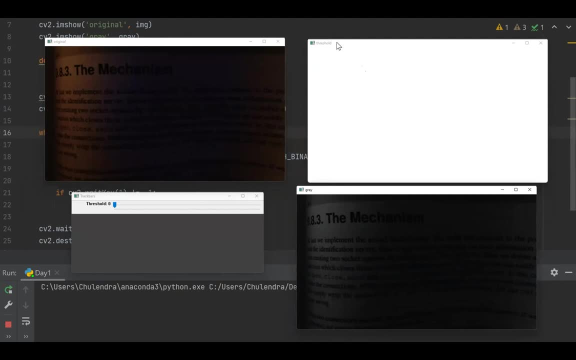 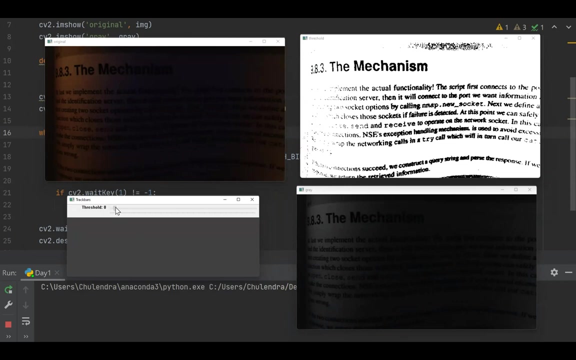 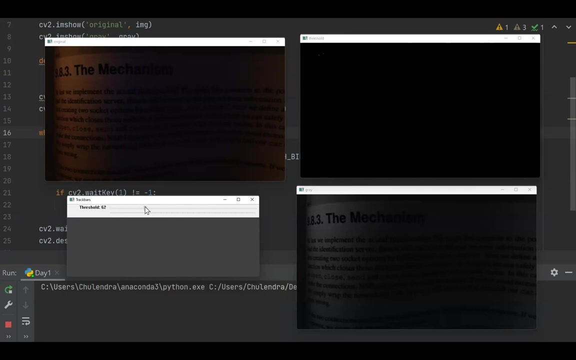 right, so this is a fully white image. let's see what will happen when we are increasing threshold, right? hmm, as you can see, you can see the. you can see the change, what I'm going to, what I'm doing, right, okay, increasing. so it will be very. 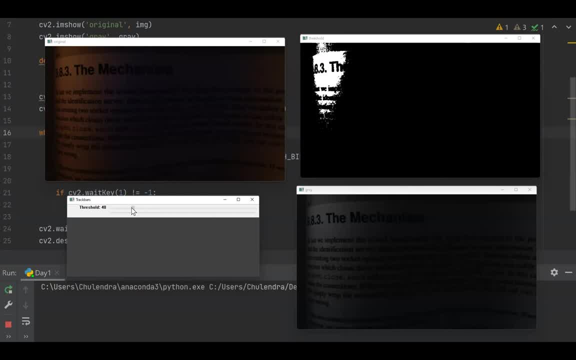 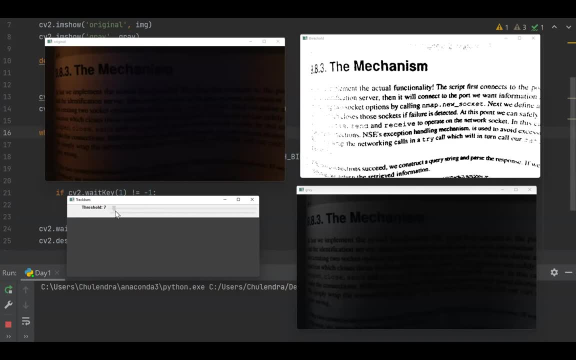 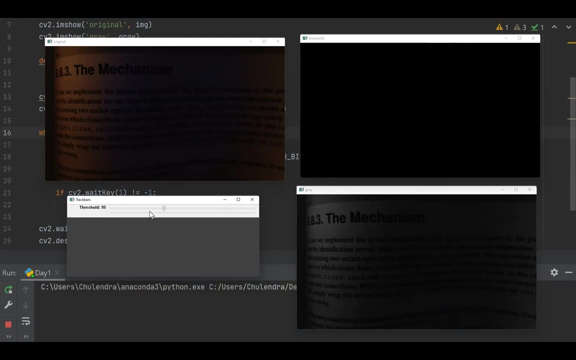 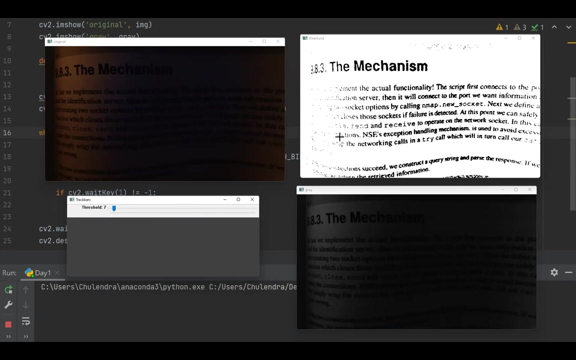 so for the dark image, the ratio value will be very low, right? so so to read this clearly, I think that needs to track. hmm, eight, eight, so you can play with this. well, right, this is valid right. so this: this path is not visible. this path is not visible. 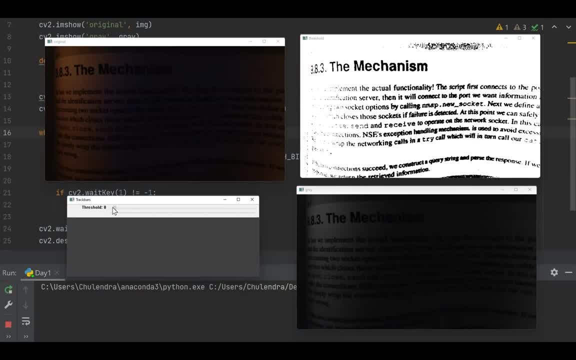 then increase the starboard, because this will be. this will be then: 10, 10, 10 is a good value, 10 is a good value. name name is good. name is good. name is good: 10, 8, 8, 8, 8, 9, 10. 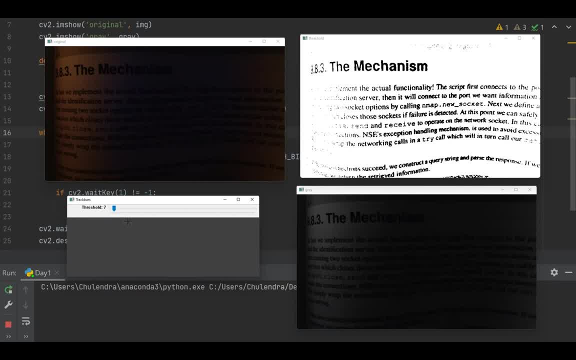 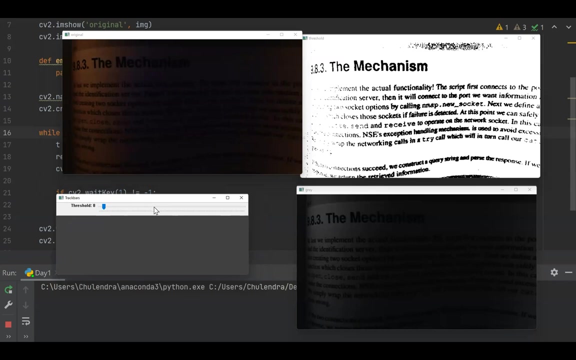 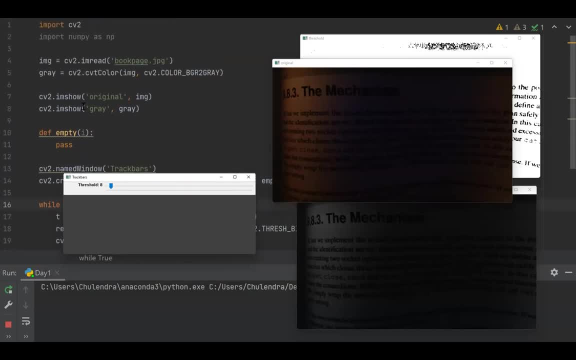 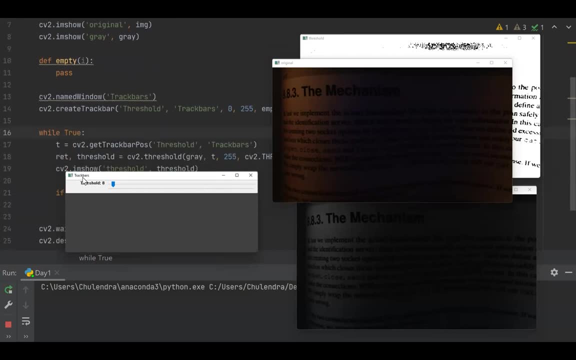 so first what i did was i created a window window name as tag bus. so this is an indoor name with tag bus, right, tag bus. so then i created a tag bar, so window window name is tag bus, the tag bar i created inside this window, this tag. 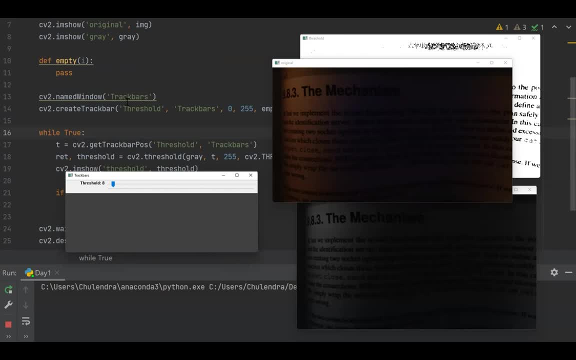 is for threshold. so this is the tag bar, tag bar name, threshold, threshold, and, and the window name is tag bar. tag bar is the window name, then zero means the default value. so when i started this, uh, if i run this again, if i break this, uh, if i run this again. 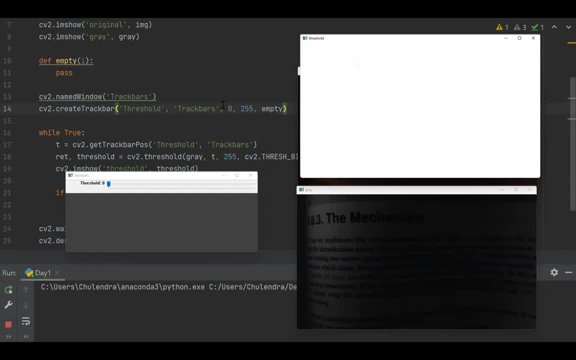 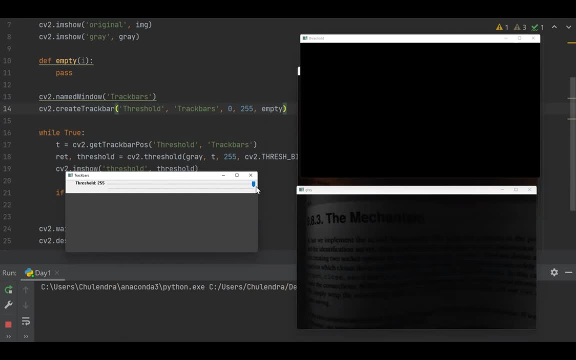 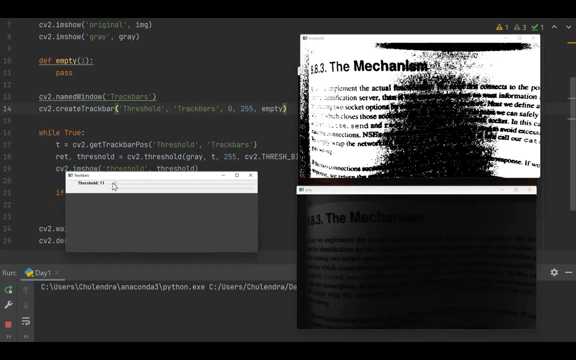 so this is default value- will be zero. so this is that's what i put here: zero, then the maximum value will be 255. yeah, but yeah, you see, the 255 is maximum, right, okay, so empty mean when, whenever we run, whenever we did your change to this. 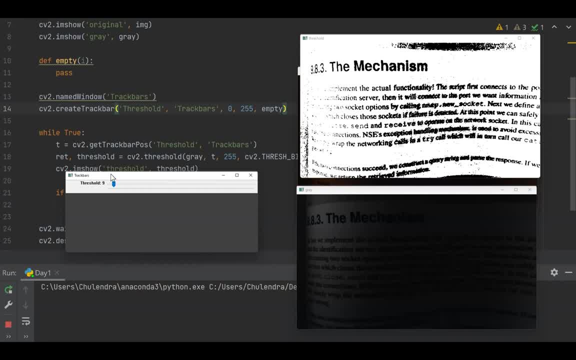 subtract bar. yes, there is a function to call right that. this is the function that i'm calling. i don't need any specific things to do, so that's why, that's why i uh define it as pass right. just a dummy, dummy, dummy, dummy function. me dummy function, yeah. 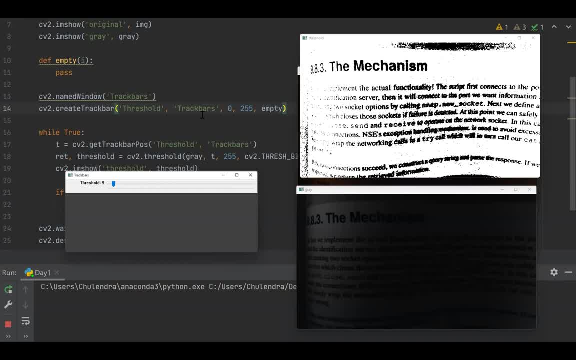 i when i slide it because it doesn't work, i don't need it. that's why i i passed it. so then this is a dummy function. uh, but it's eight. that's the best value i've seen. it's not as good as eight. it's not as good as eight. 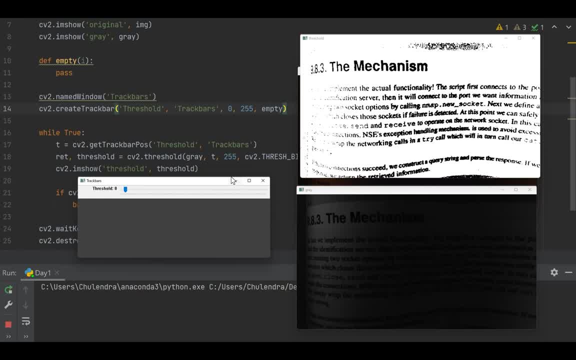 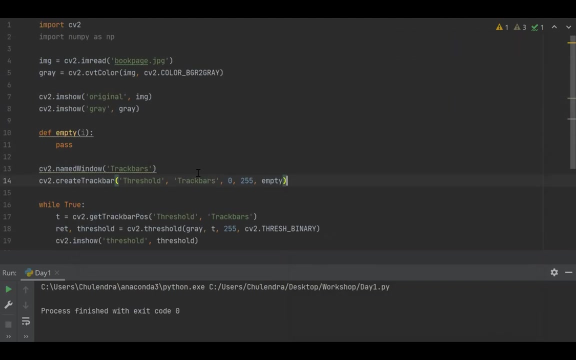 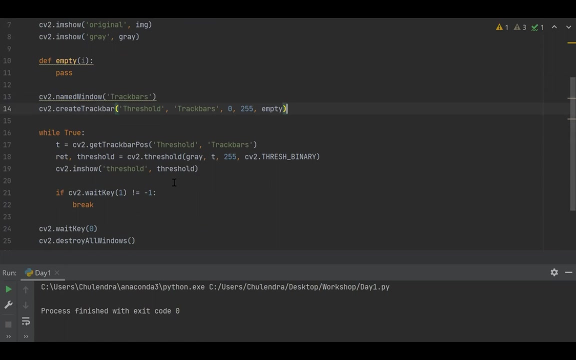 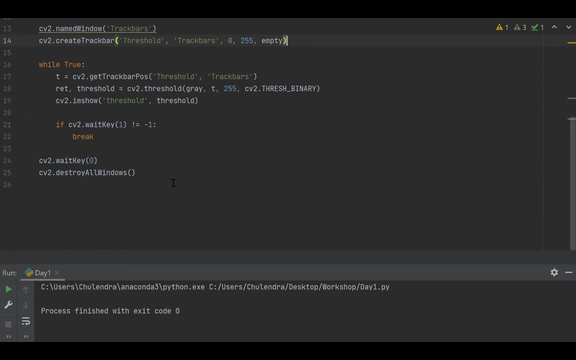 so this is the basic structure of this one and this is your way. but if you want to, just annoying, but um, with your preset limit, and да, um, sorry. now what i'm going to do is: uh, there is another thresholding technique called uh- adaptive, to show you adaptive, to show you right, adaptive thresholding. so 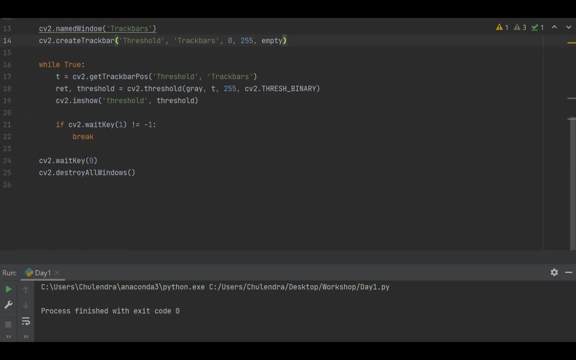 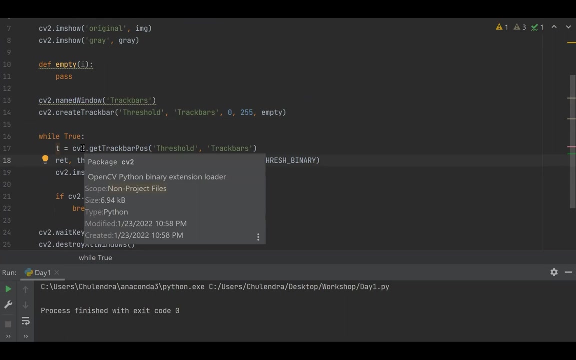 so in simple thresholding, the global value of threshold, that means global value of thresholding- this t value is the value that i'm going to use to threshold right, so this global value of threshold was used, which remained constant throughout. right, so it is a constant. so this t value is constant. this track bar, the value given by this track bar, is constant. 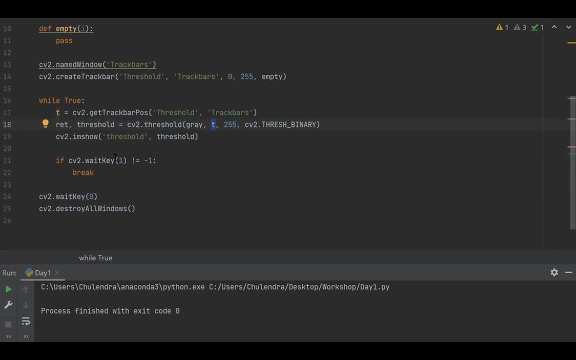 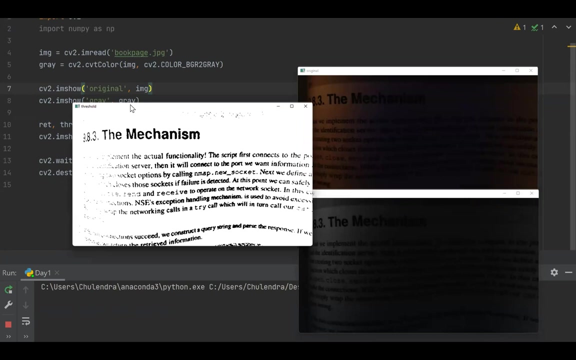 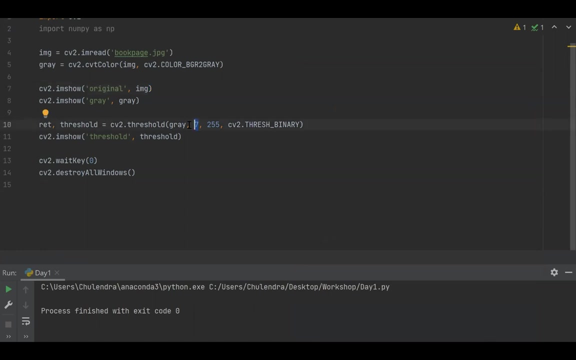 uh, so i have removed this tag bar, so i want to know that it is seven, so i'll delete this tag bus. i don't need this anymore. i'll remove this, so i will select that seven. so seven is so. so this: this is the global value of threshold, right? so this is the. this was given to us, right. 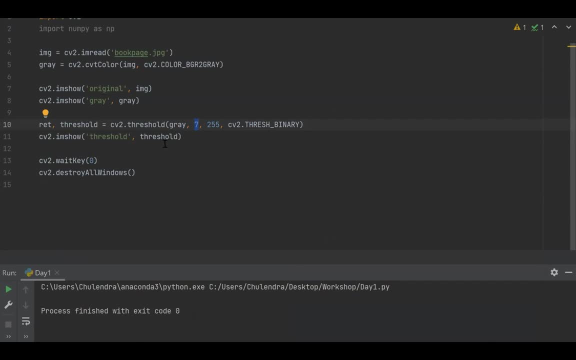 so. so concentration value won't help in the case of variable lighting conditions right, in different areas. so if there is a variable lighting condition in different areas, this thresholding is not good at all. right, because in variable lighting condition the thresholding value has to be way right. 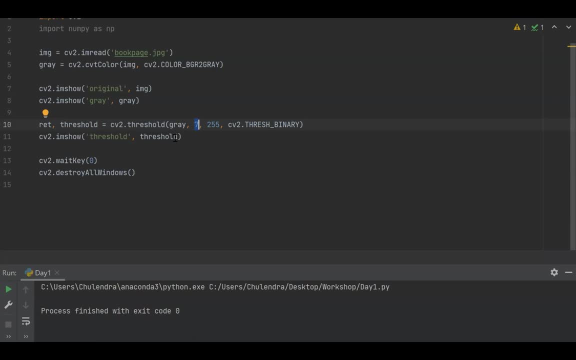 so so, maker, maker, you can take a deep time factor choking. the method where the threshold value is calculated for smaller regions leads to different issues for different region with respect to the changing lighting condition. so we use cv2.adaptive threshold for this right. so so let's see c2.adaptive threshold that will show for that. 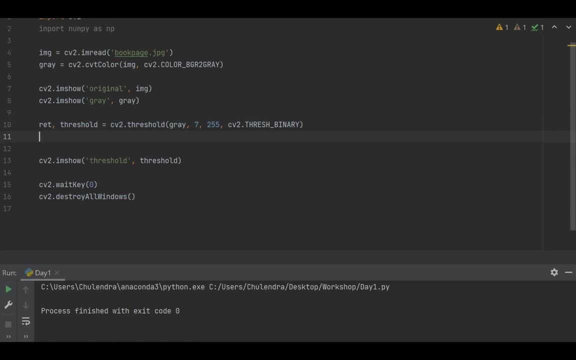 you can see that this is the cv2.adaptive threshold. adaptive as polycats adaptive. adaptive equals cv2.adaptive threshold. let's pass gray here. gray maxi value will be 225. adaptive matrix method. there are there are some adaptive methods, so i'm going to use cv2. 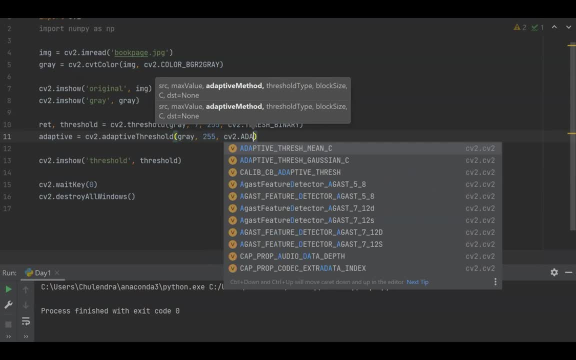 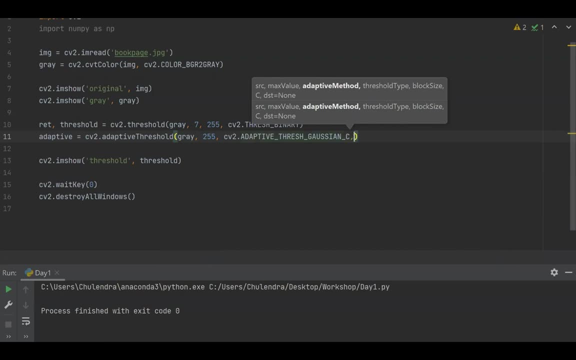 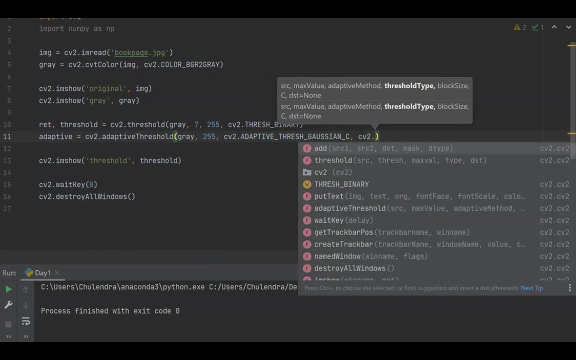 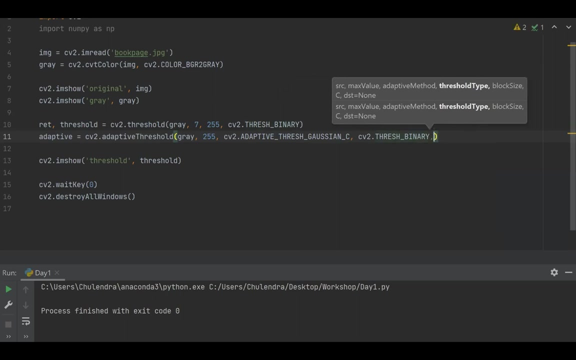 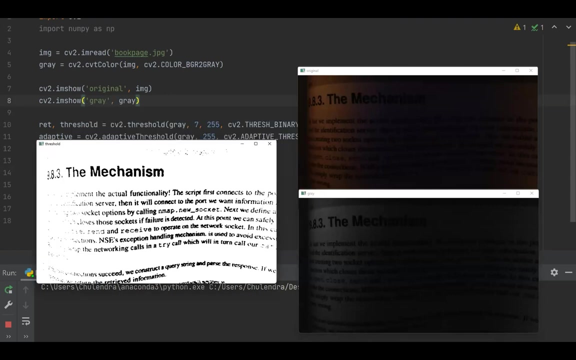 and that and then do this: go: cnc, cv, then middle threshold, type, cv2, cache, cache binary, binary binary- and the block size- i'm selecting 115- and the cv1- cv1 adaptive to show adaptive adaptive. this is my adaptive. let's run this. where is my adaptive? 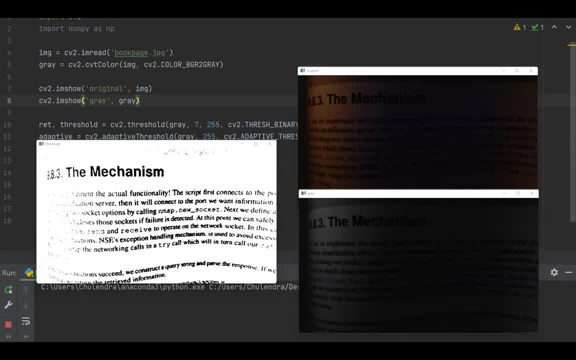 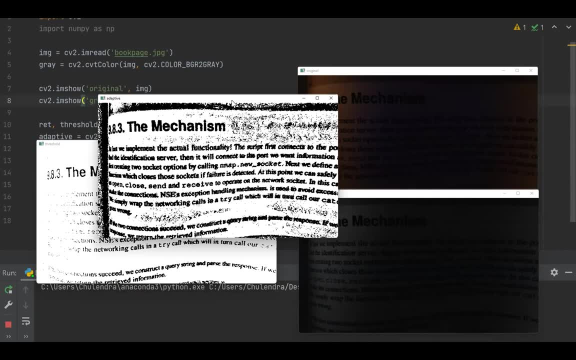 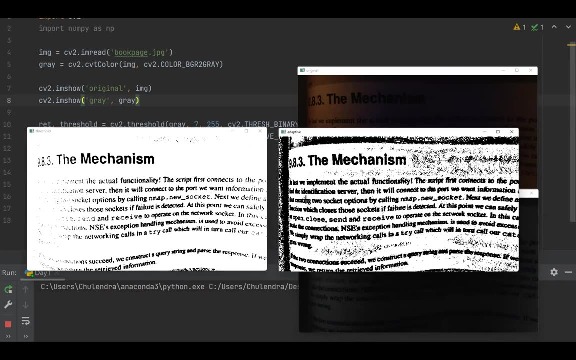 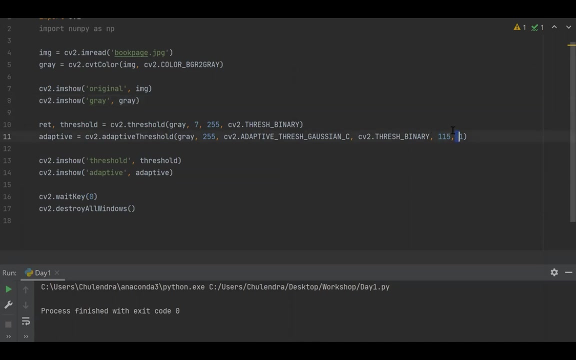 this is the adaptive thresholding result. so it is very clear than this one right other than thresholding- simple thresholding, adaptive thresholding- is very much here right. these are the parameters to pay with right, the 115, and you can use tag bar for this for this. 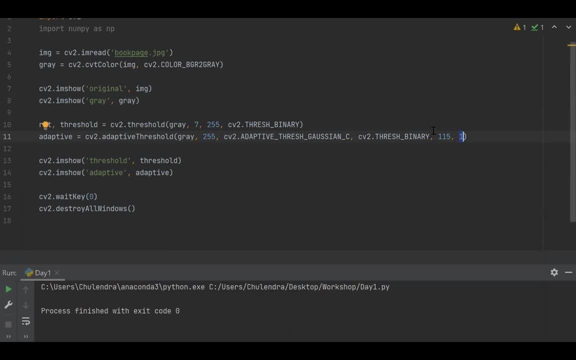 for this same case, but i'm going- i'm not going to use trackbars for this now as the time flies. so this is the. this is how this is. this is the thresholding method mode. then this is a adaptive vision, adaptive type, right, so you can refer to this. 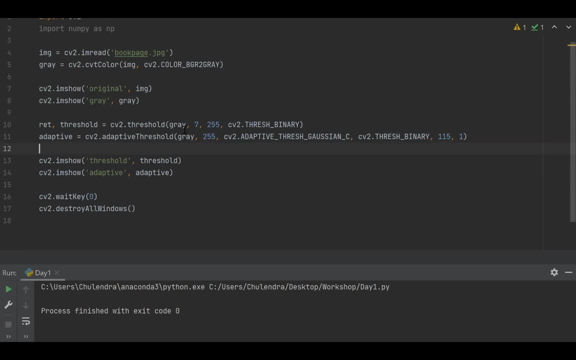 later, so you can. there's a theory. it is more simple theory you can understand. here is to go through it. so i have some links. i will post them. so i have planned to create a notebook. i buy the notebook, uh, including all the exercises i did. i am doing this, i'm doing this. 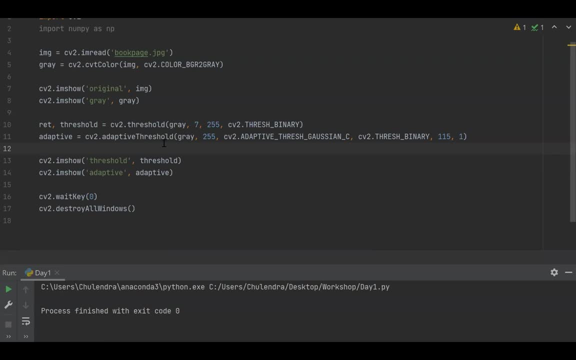 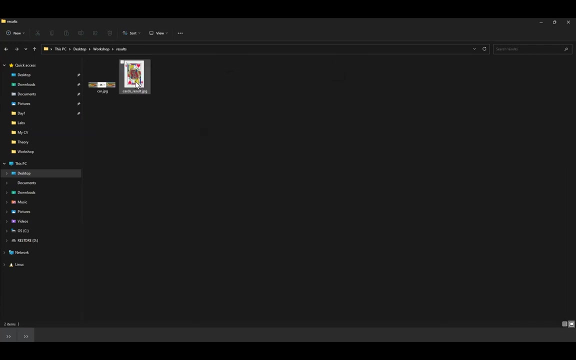 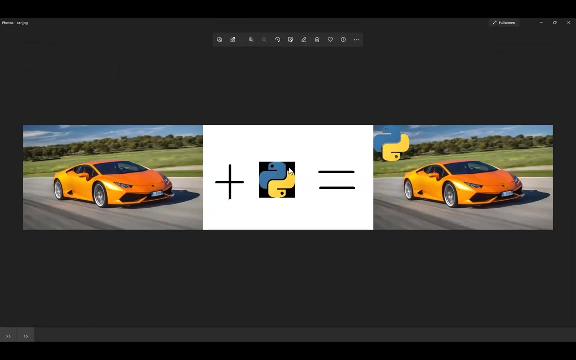 uh, workshop, right in that workbook i will post the all the theories regarding to each functions, so don't worry about it. so, so, that's about thresholding. so since, yeah, we have good knowledge in thresholding, so let's have, uh, a cool thing, which is this one. so i have image like this, right? so, and the image also like this, right. 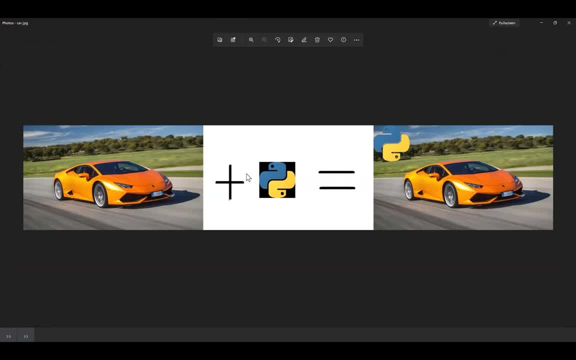 so, when i add these two images, i am going to superimpose this image on this image image. so the result will be like this: right, how to do it. right, that's what we are going to see, right, so, as you can see this, this black parser filled with this, with this image, right. 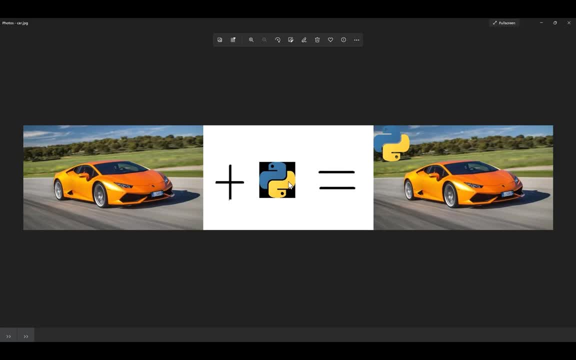 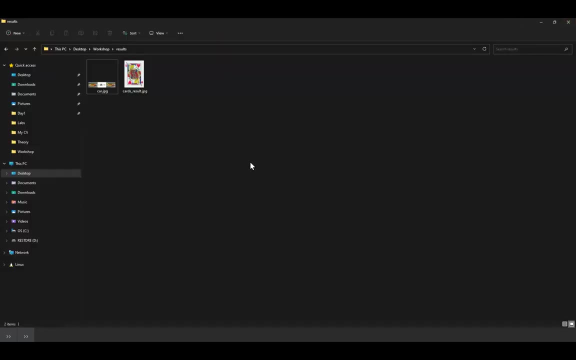 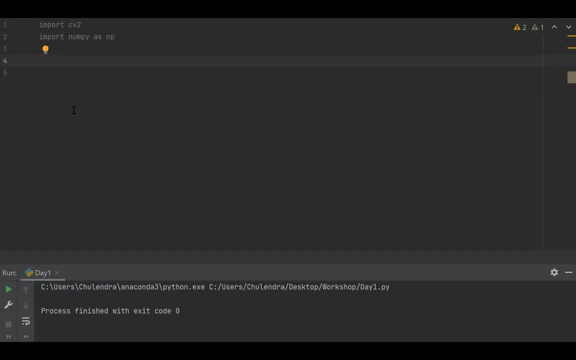 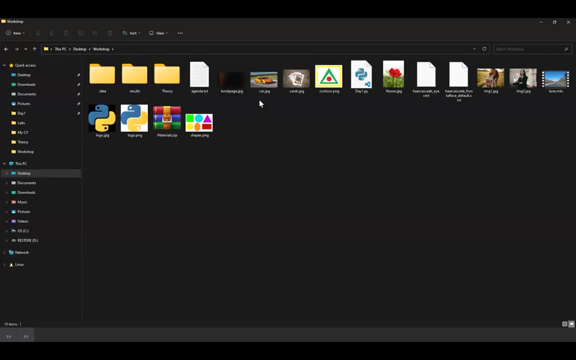 so. so this is the result of thresholding, so let's see how to obtain this one. this is very easy. there's a couple of kodi, so i have two. so in my directory i have two images: cardjpg and logojpg. right, i will do these two images, okay, so? 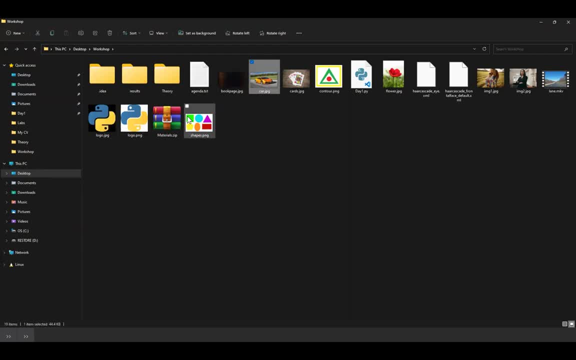 after that, i'm going to use these, these two cardjpg and logojpg, but here, first, i'm going to use this cardjpg and logojpg. logojpg has black background. right logopng has white background. let's see how to do this. to do that, let's first 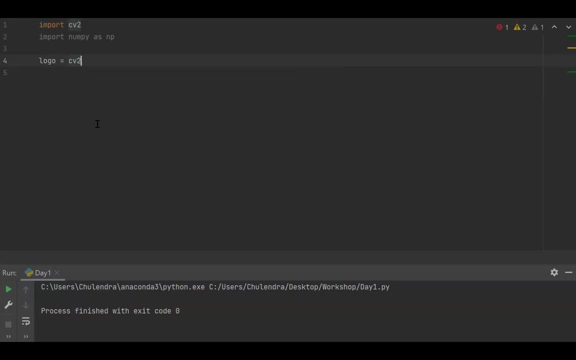 read logo file: c2 dot img. read logojpg. logojpg and image is. this is a background image: c2.inv. cardjpg. right so, boss, columns, chance, Bingo. check the course. check, no, no, who has three, three nougat shape. ingredients of tuple with number of rows, number of columns and. 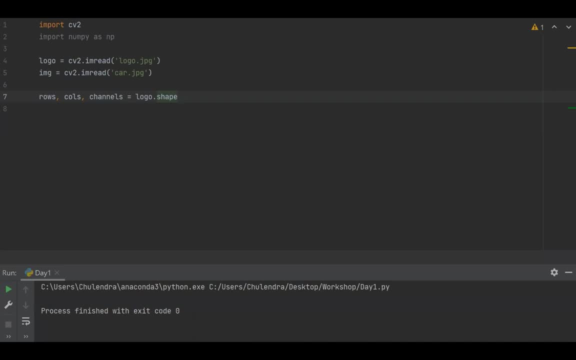 number of chat. right, so i'm i. so i have routine number of rows and number of columns, so i lead for these four. uh, super, super. so let's select the region of interest. region of image. region of images is the region of image. what is mean by that? because 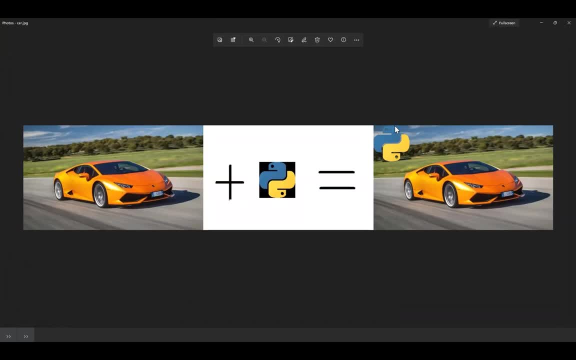 then you can see that i have taken this logo and i have highlighted it here. so i have taken this box and i have highlighted it here because this is my roi, so i have to do this work in this box. this is what i have taken in this box, so that box is my roi. region of image. 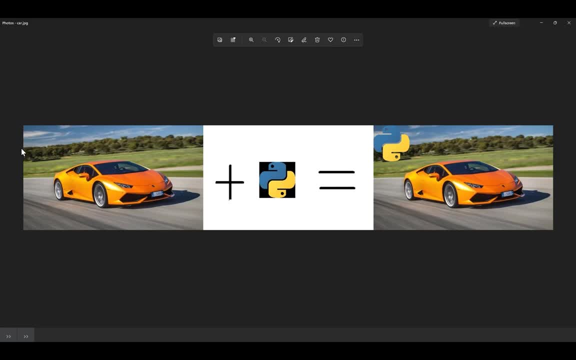 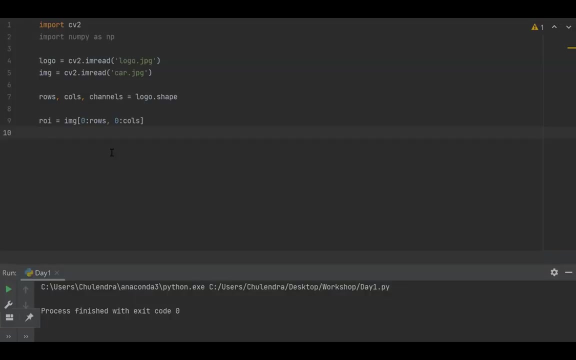 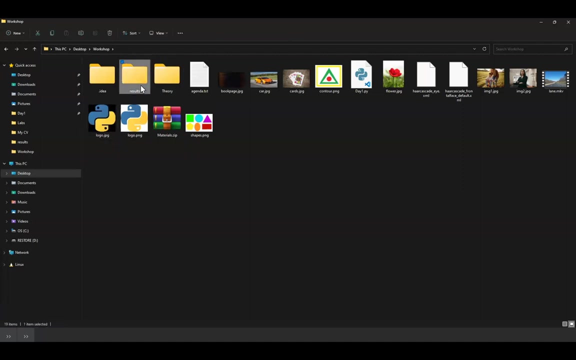 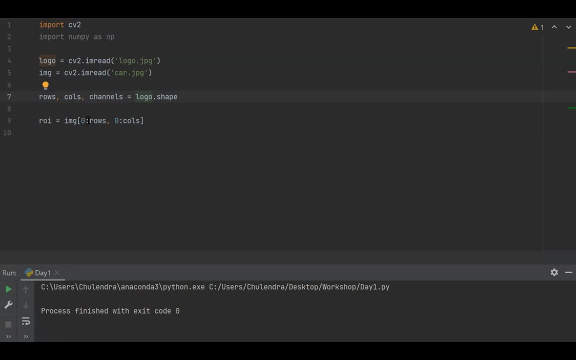 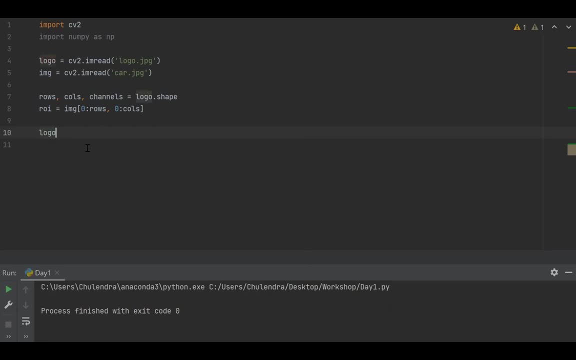 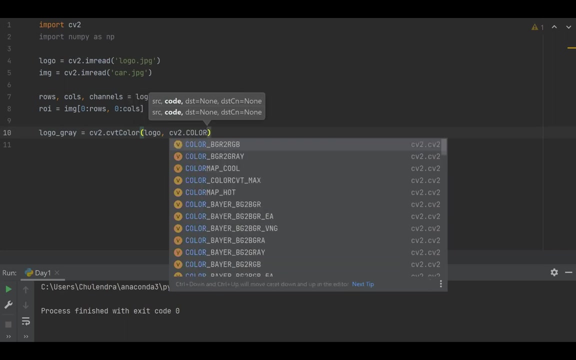 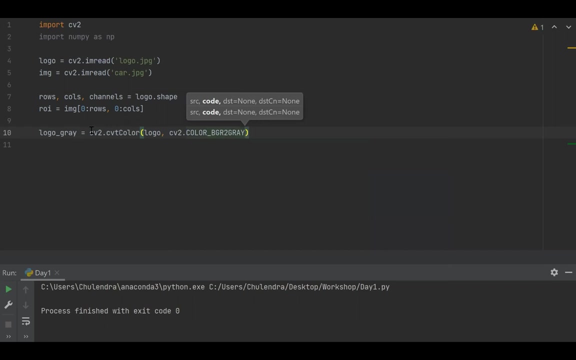 So I will use the standard color Logo: gray. I am going to threshold the logo. I am going to gray scale the logo. The region is gray, The region is gray. I am going to gray scale the logo. The region is gray, The region is gray. The region is gray. 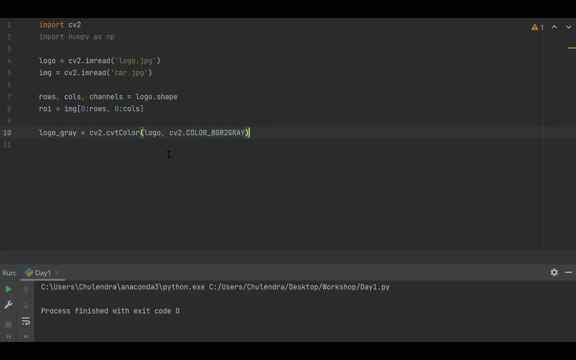 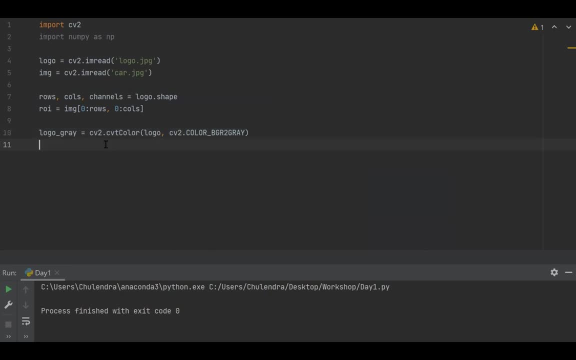 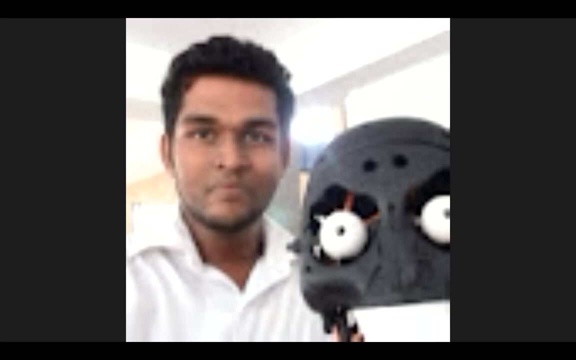 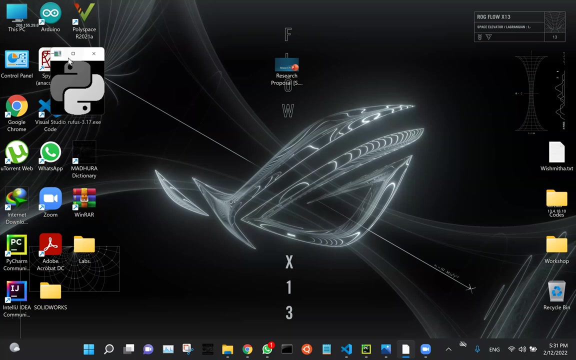 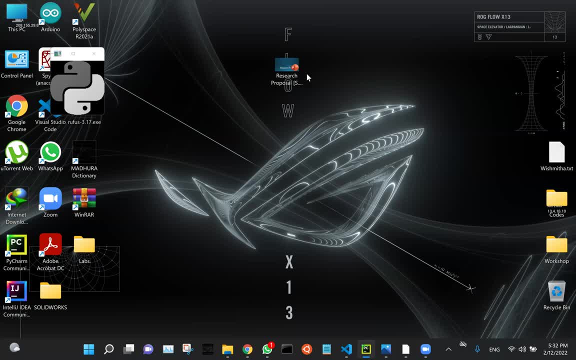 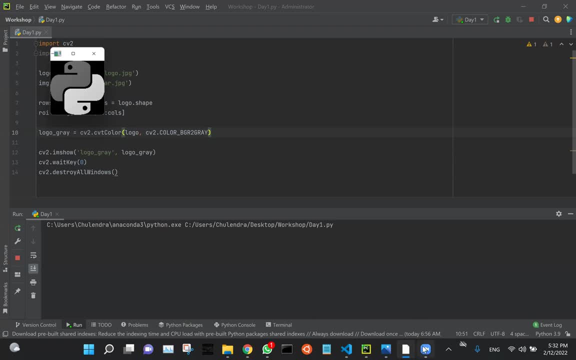 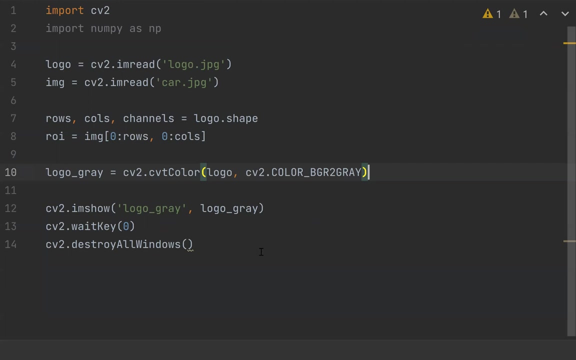 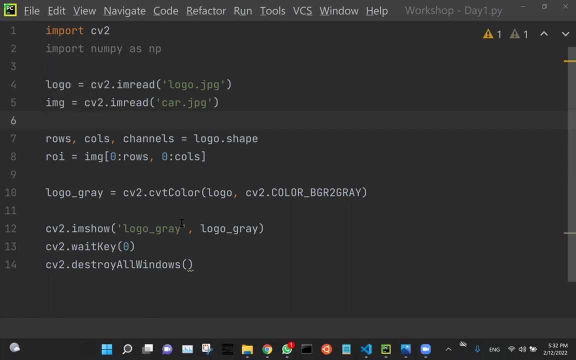 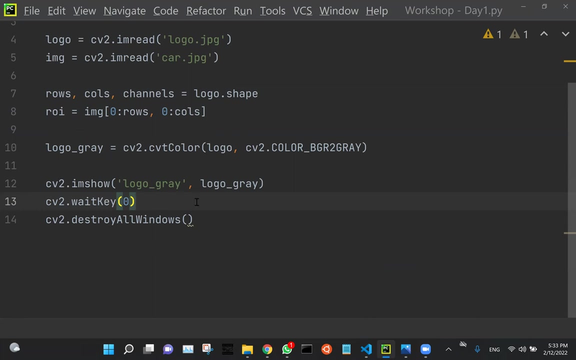 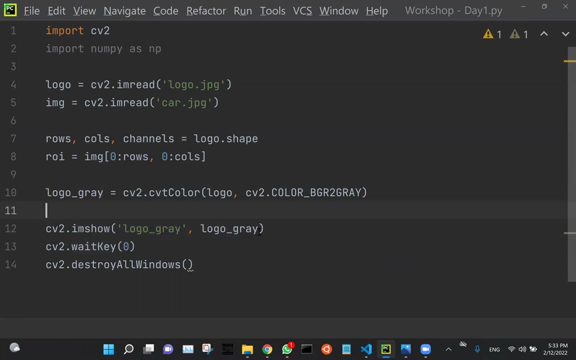 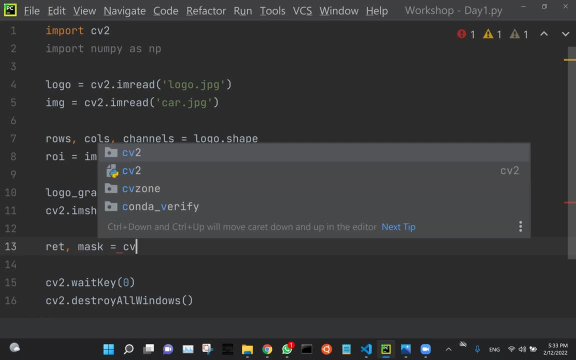 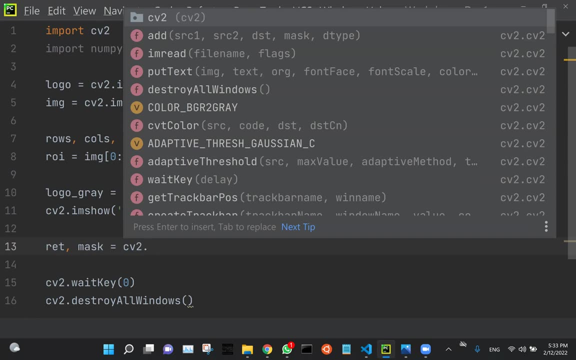 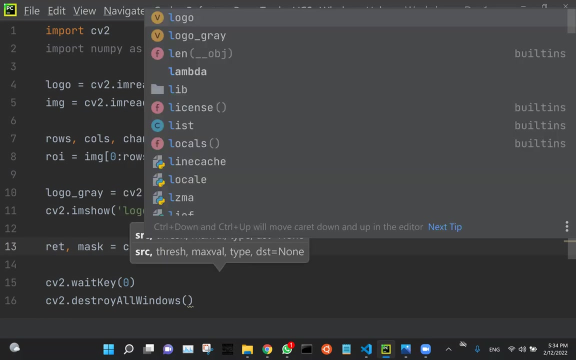 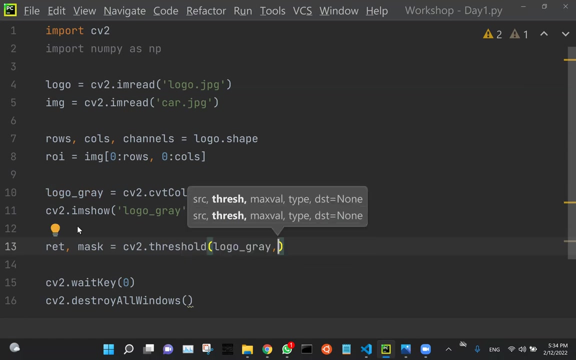 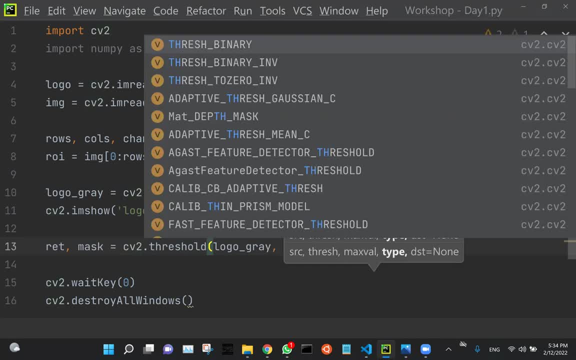 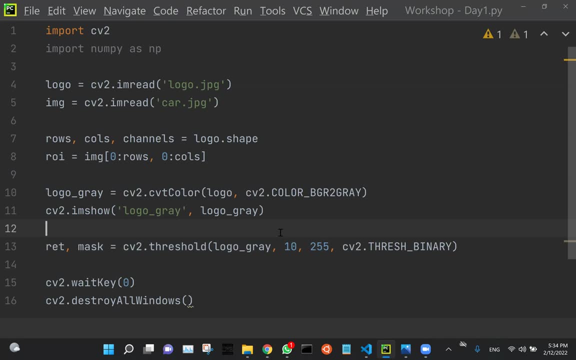 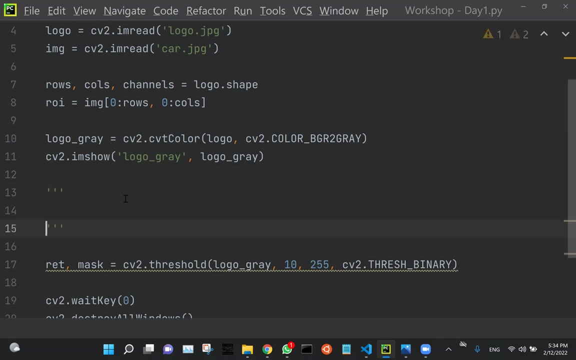 And profusely asked the next minute: Bye, binary, just. binary means. I said before this binary, so if I recall that they showed in technique, if it's from a wide greater than 10, you should 255 else here. so see to the test. binary means the. 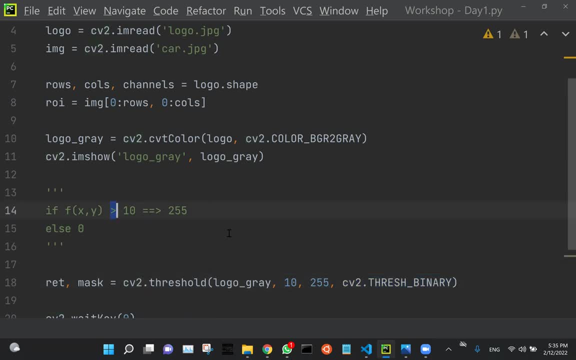 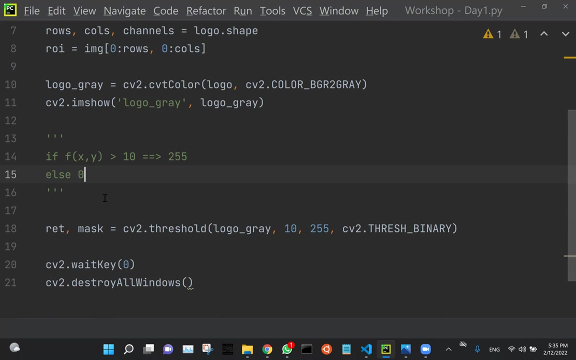 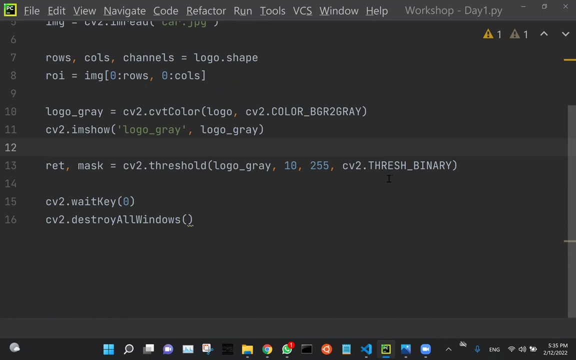 comparison operator is in this way right to say this binary in binary, in this comparison, will be like this, like this, right like this, so. so in this case, I'm going to use this one, which is test binary, this binary, and I'm going to do this so I have period mass, so I need a unit mass also. 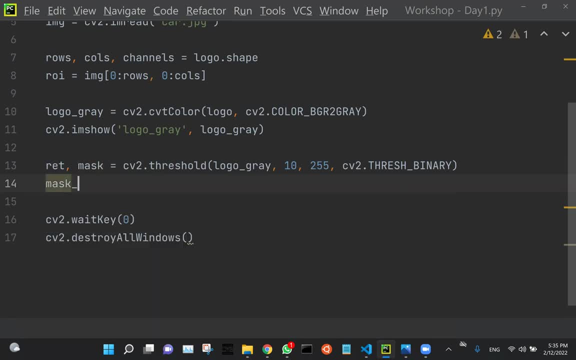 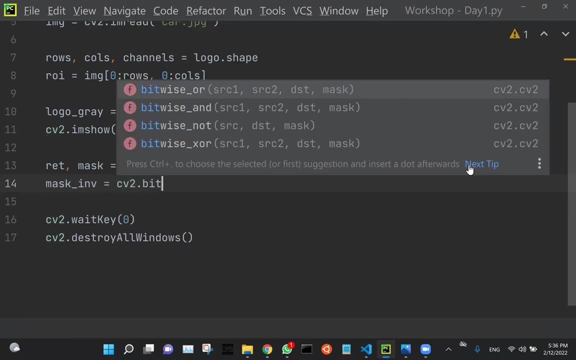 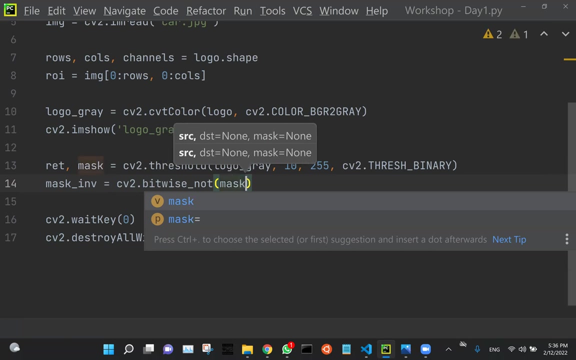 right mass in equal c2 dot. bitwise naught. bitwise naught right. so I have period mass, so I need a unit mass. also right mass in equal c2 dot. bitwise naught that. but this is not operation of this mask, so you will see will. you will understand what. 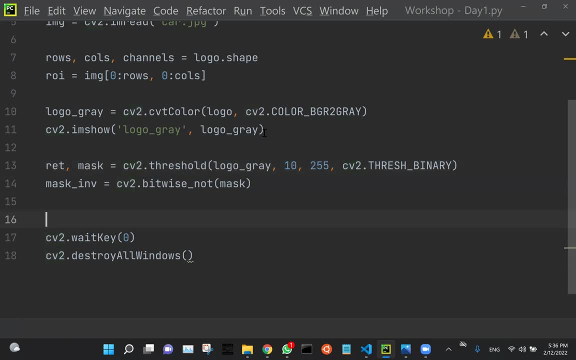 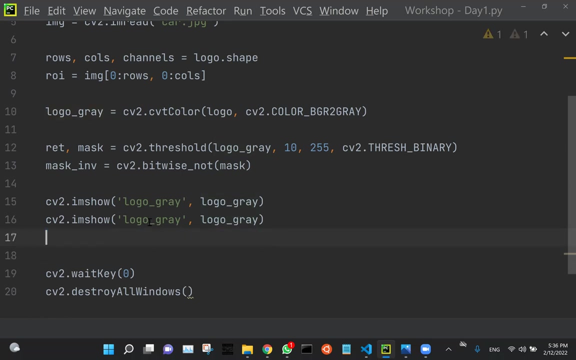 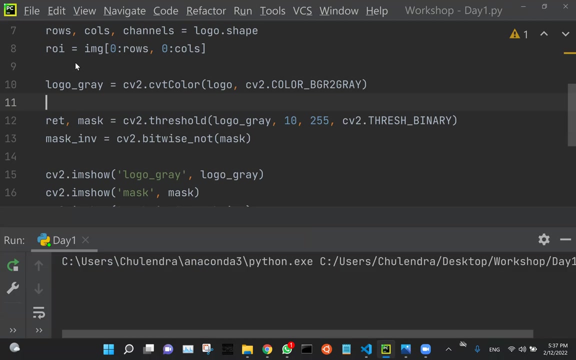 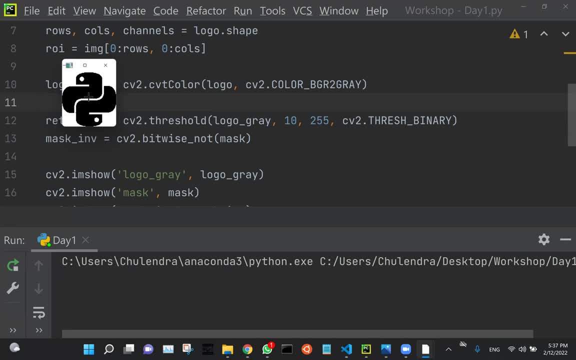 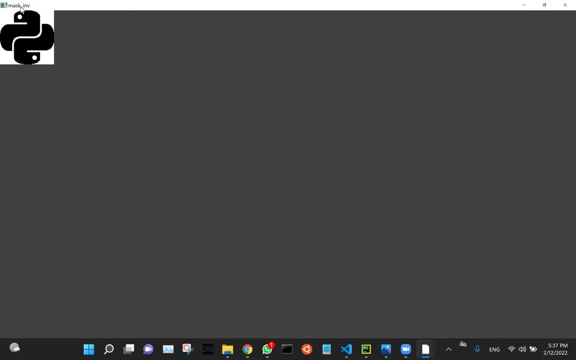 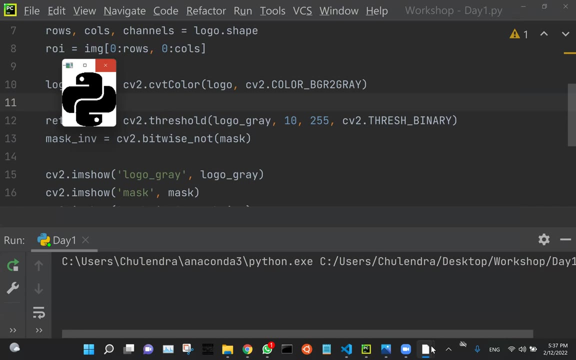 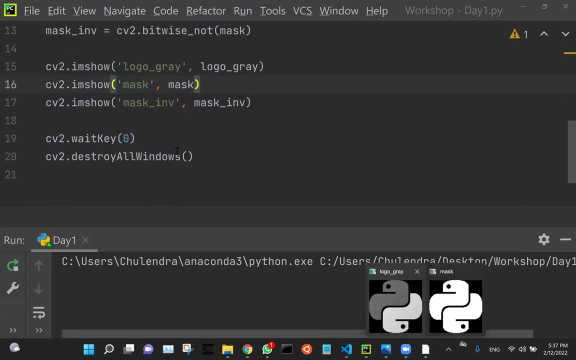 This is the binary, The Binary in Mass in version, Mass in, And This is the mass. This is the mass in Mass in Right, As you can see, The, The Background, The, The, Now, theena. 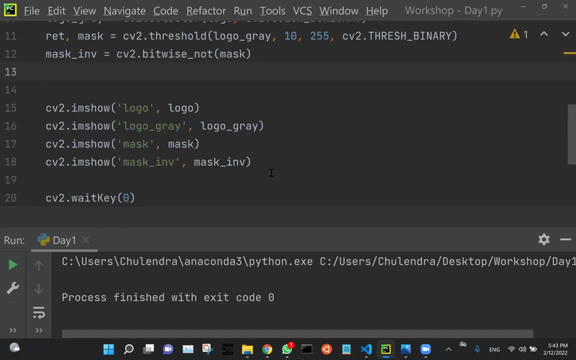 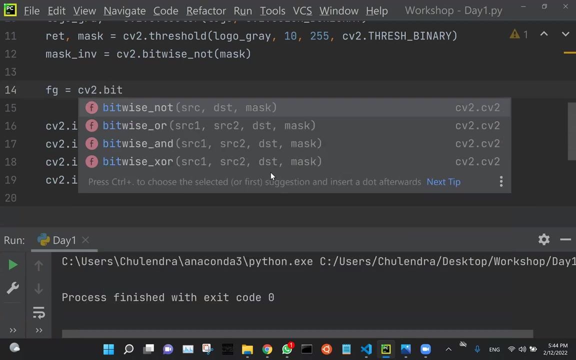 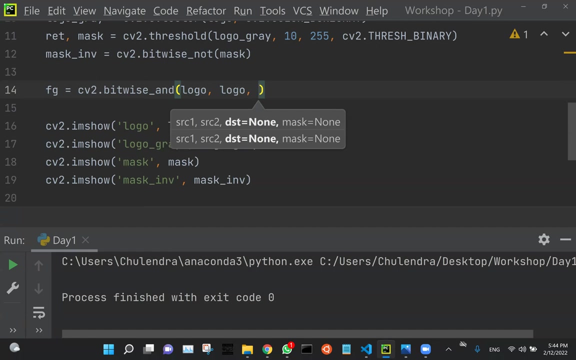 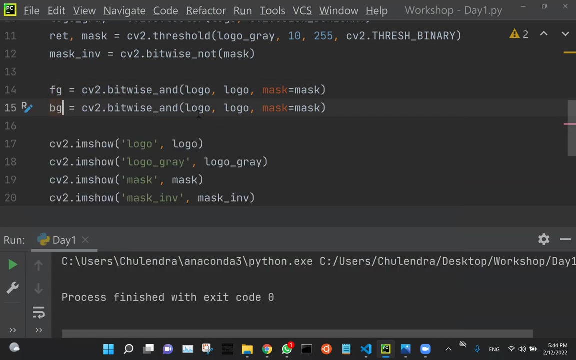 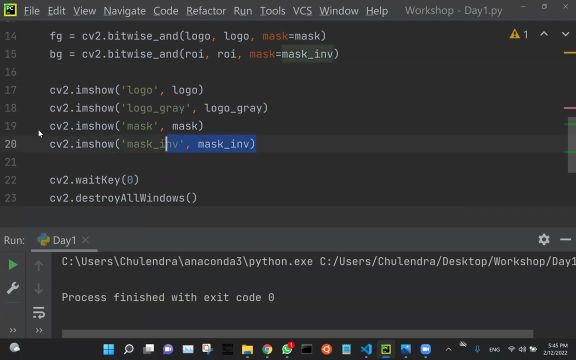 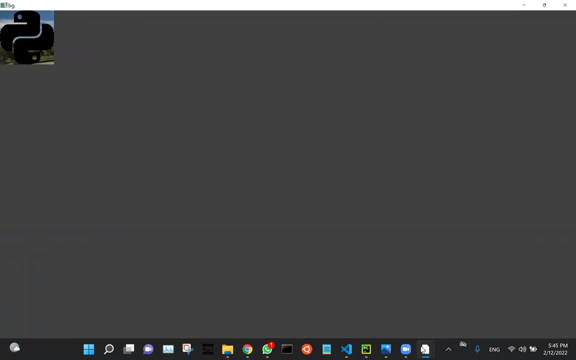 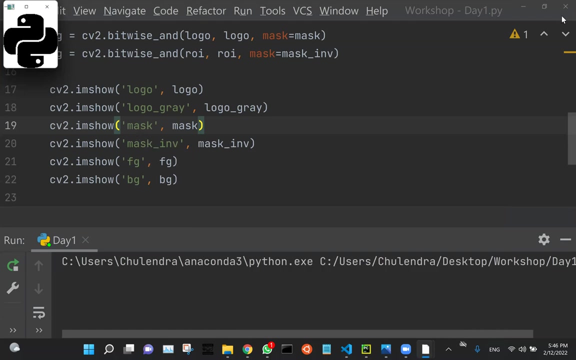 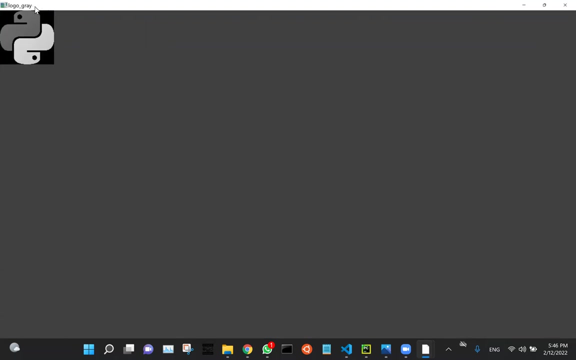 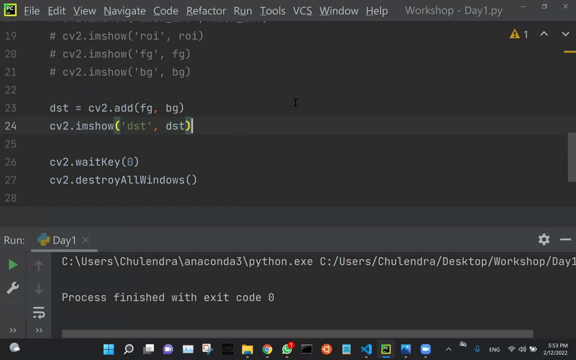 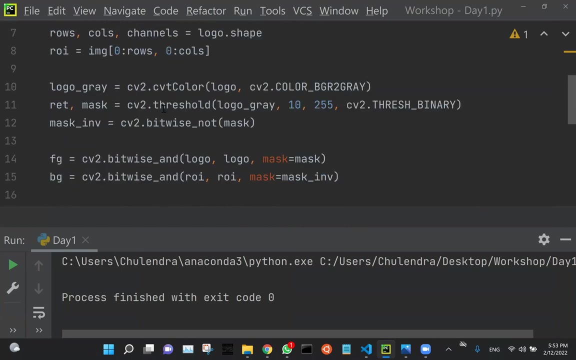 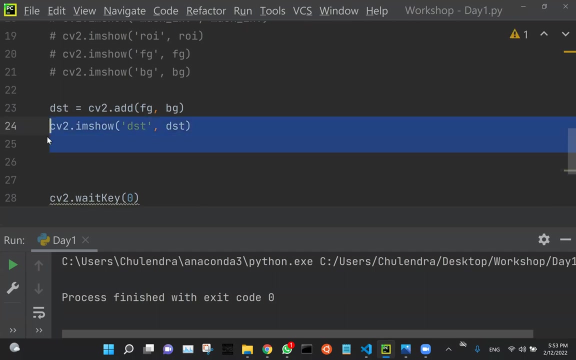 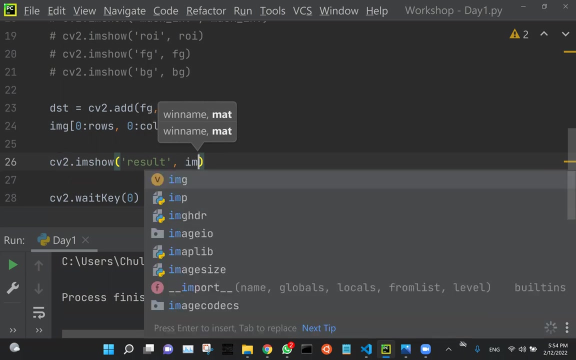 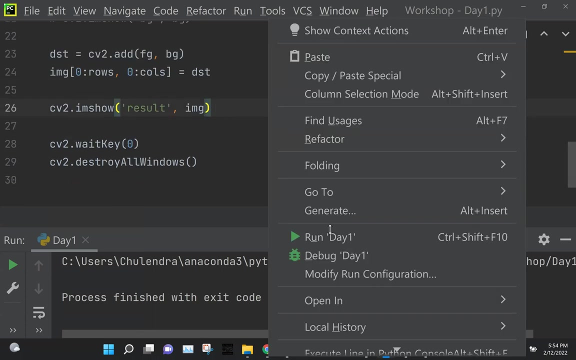 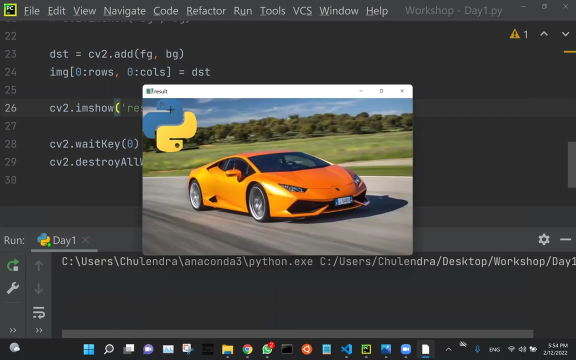 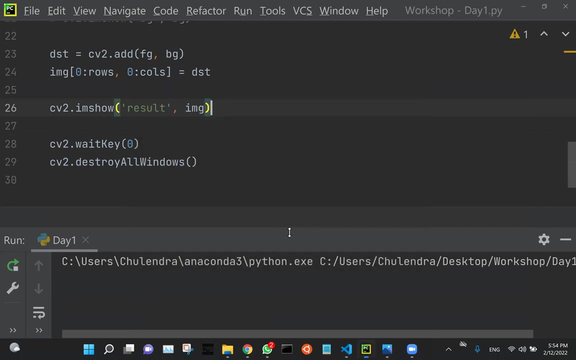 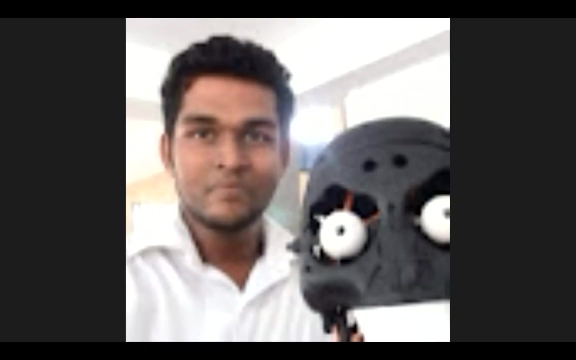 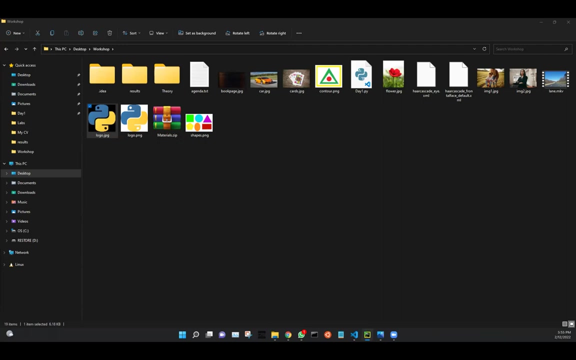 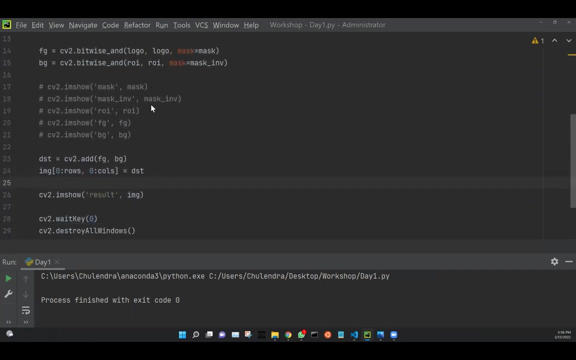 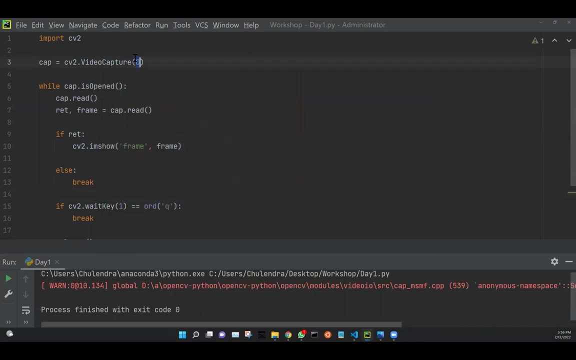 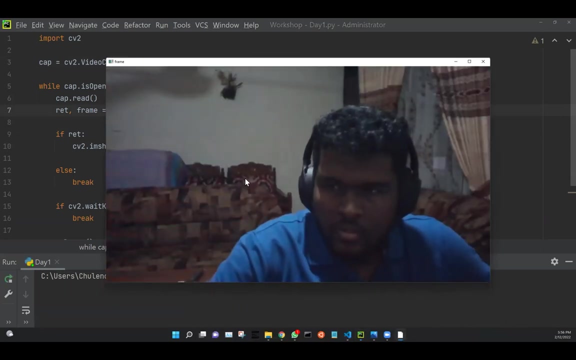 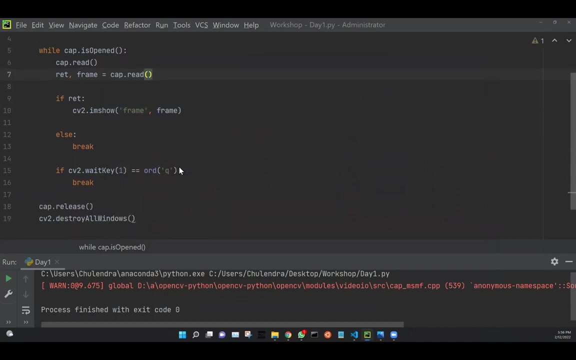 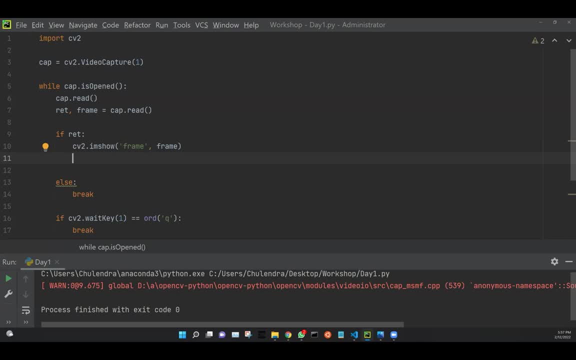 Okay, So yes, he could see me, do not Kenny? So, as time flies, I just copy and paste this code. I just see equal, Can you see? so? so this function is called Kenny, So we can see. So here we have to use the values and we can't remember what are these names that I'm doing. 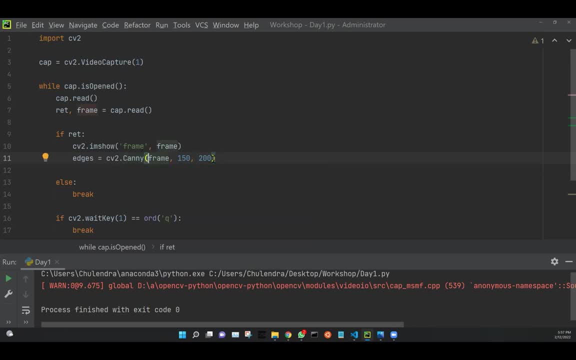 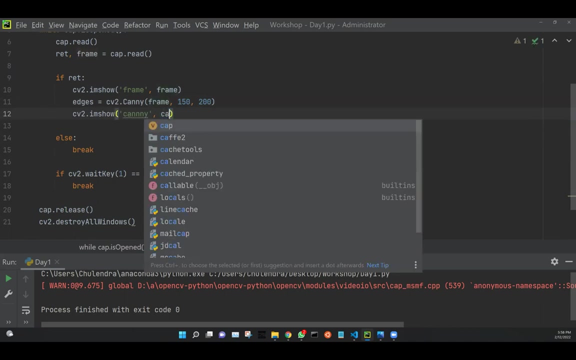 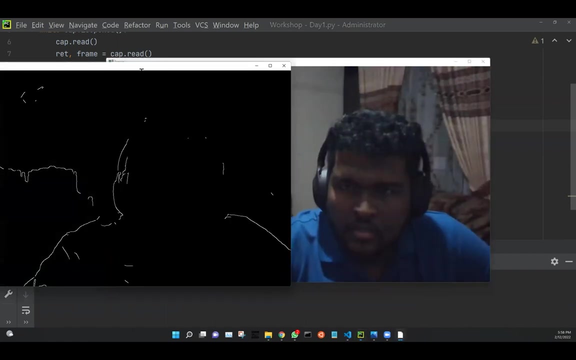 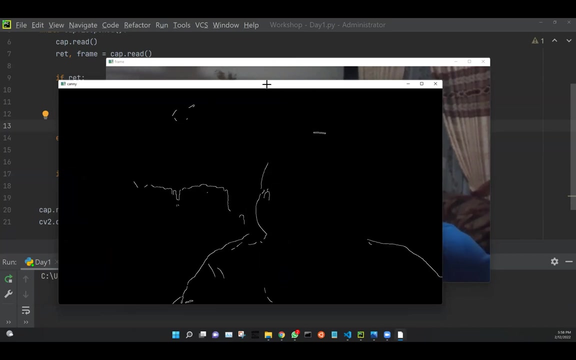 To show one and to show to play. you can play with these values using tug bus. So for this purpose, I'm nice Just on 15200.. So let's visualize this, Kenny, okay, and this and this. these are the. this is the image that i'm going on and i'm receiving. 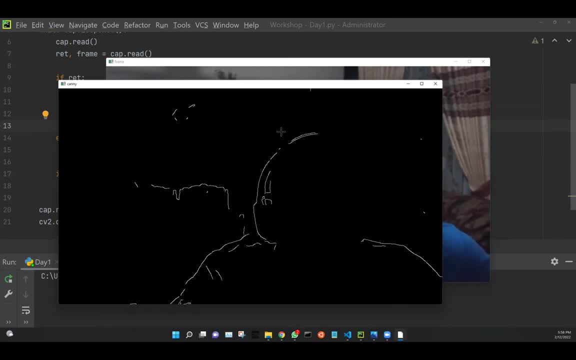 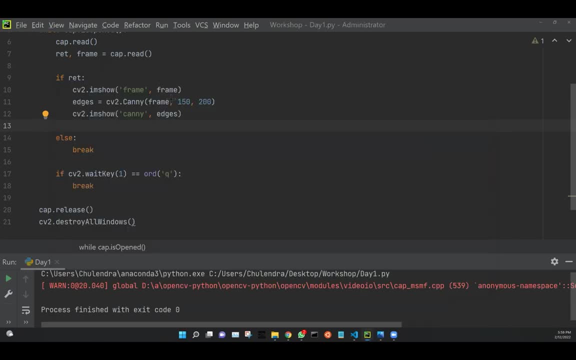 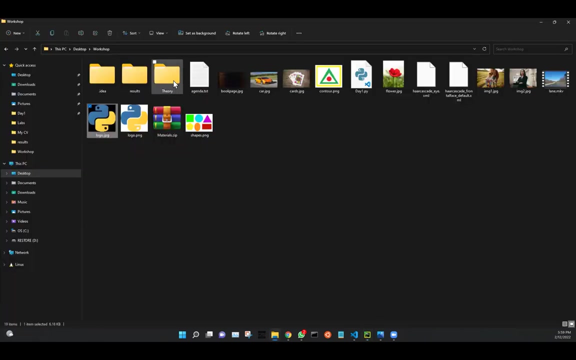 uh, as you can see, you can play with these numbers. uh, so that's all for today. next today, uh, and and the next tomorrow. i would like to talk about vast perspective, past perspective, in fast perspective. uh, i will tell you tomorrow. yeah, aspective color direction, apological transformation, shape detection, face detection. 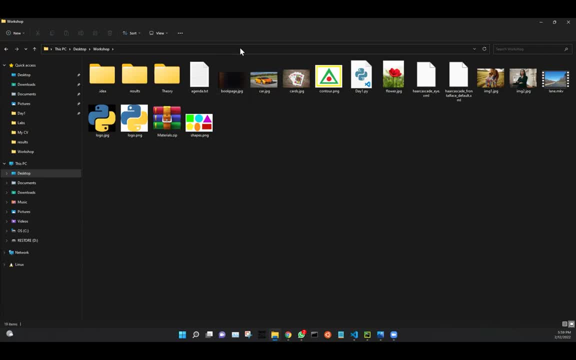 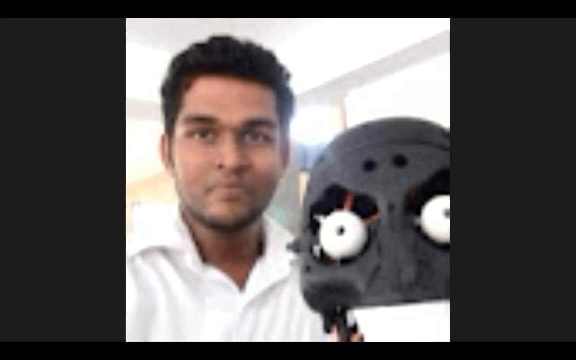 point to us all. those, all of these will be um will be touched tomorrow. so, so, so, let's, let's meet tomorrow. yes, thank you, uh, thank you, uh, so, uh. this is the end of the today's session. uh, so, uh, there is another workshop for uh.